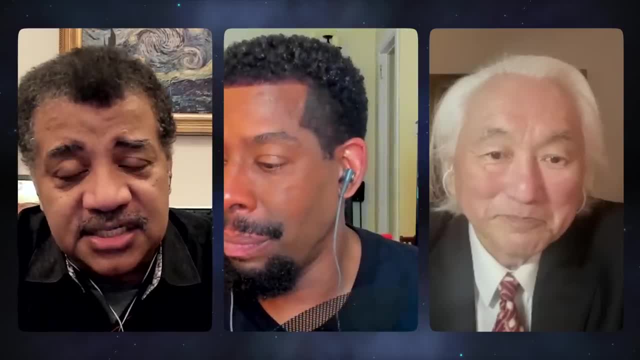 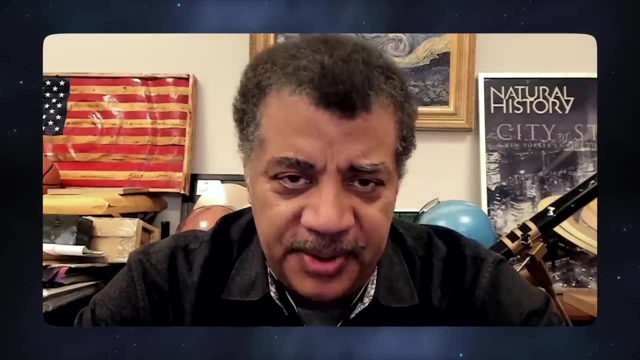 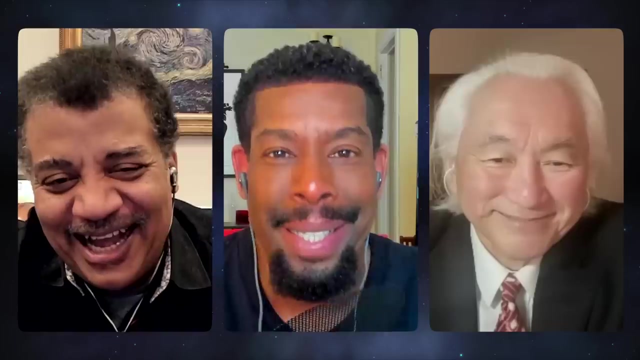 this is at Cosmic Queries, where we solicit- have already solicited questions from our patrons through our Patreon portal. But I want to just warm up a little bit And could you just give us in one sentence what? no, Yeah, Yeah, Exactly, I'll give you a little more than that, So tell us. 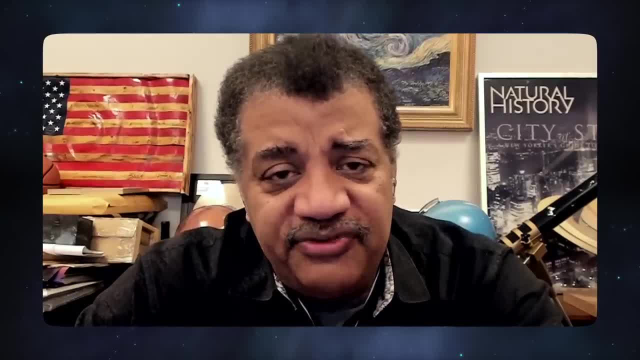 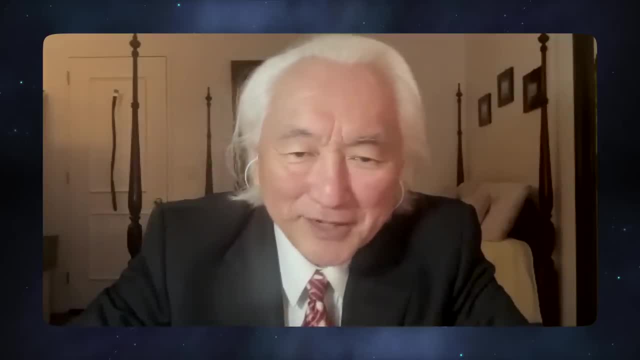 what we should know, what quantum computing will do differently from regular old computing. Well, computers have gone through three stages. The first stage was analog. computers will be computed on sticks, levers, gears. We would turn the crank to do a calculation. 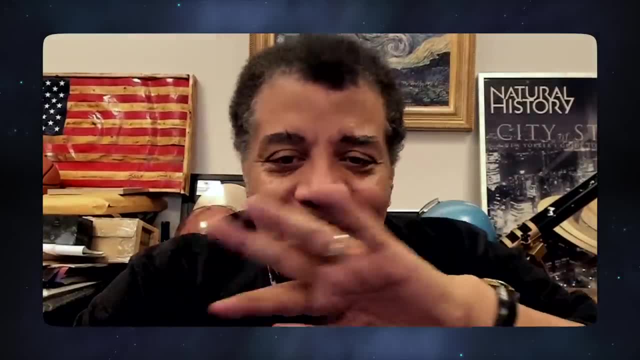 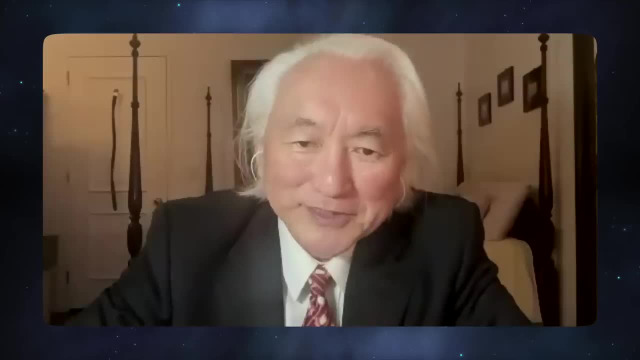 But the abacus was one of those too. right, The abacus, The abacus, that's right, You know. slide rules, right. Then comes electricity, So, and the transistor, So, all of a sudden, everything becomes a matter of zeros and ones, zeros and ones and digital. 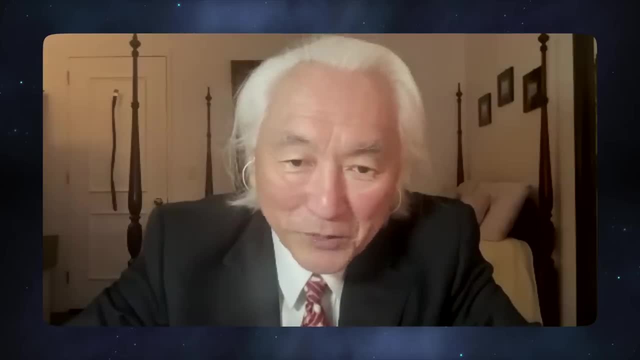 And that's the computer revolution of today. Now we are beginning to enter the third stage in the evolution of the computer: No longer computing on transistors, computing on atoms. This is the ultimate computer. You can't do better than that: Computing on atoms, And that's. 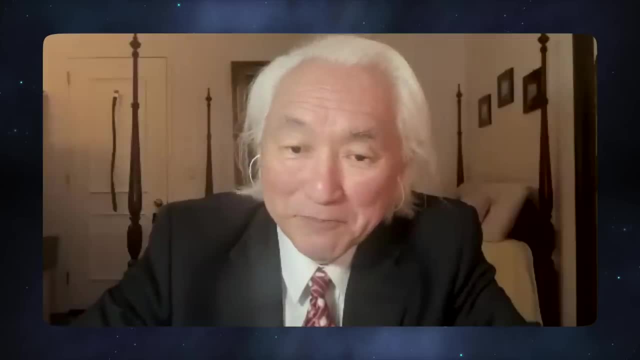 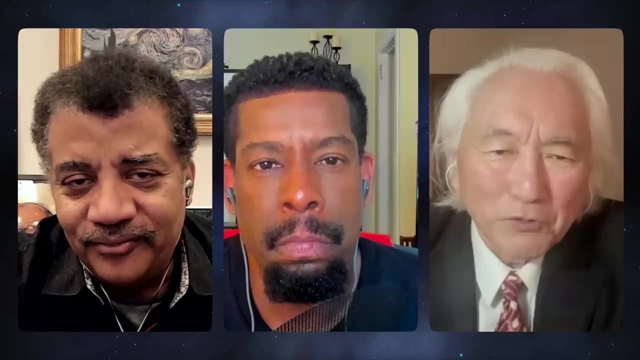 what the quantum computer is all about. They exist already. They are millions of times more powerful than our most powerful digital computer on certain tasks. So there's a race, a race between China, between IBM, Google, Microsoft, a race to see who can get the first all-purpose quantum. 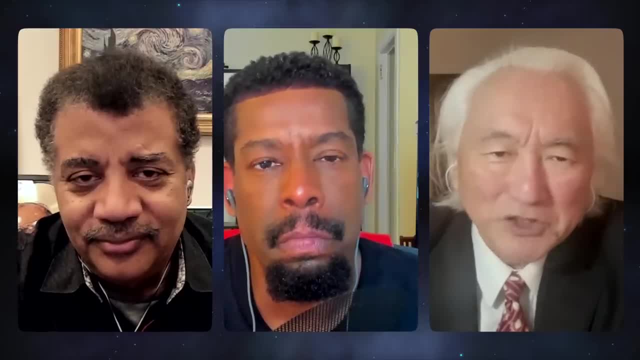 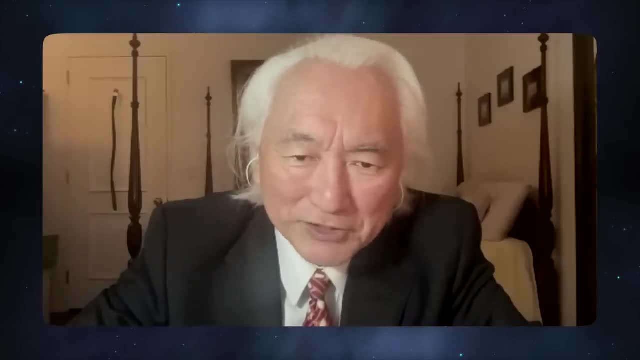 computer to put on the marketplace, which will change everything. The CIA is interested in this, All the big commercial banks are interested in this. Aerospace energy, you name it. Everyone is interested in who is going to be first to to bring out a commercialized quantum computer that could outrace any normal. 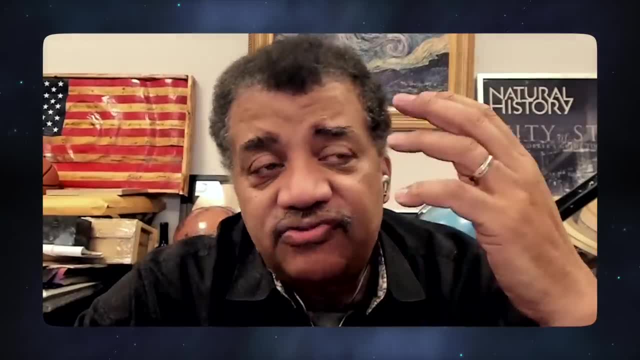 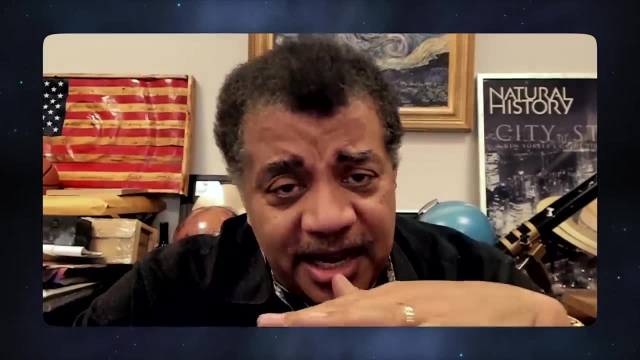 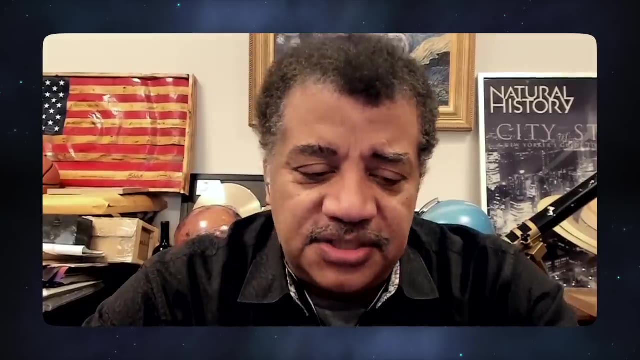 computer by a factor of a million. So, by the way this race, you know, scientists among them, but certainly the military, were early out of the box in regular computing, right. So, and then that regular computing that finally sort of spilled out of the military and science and engineering, 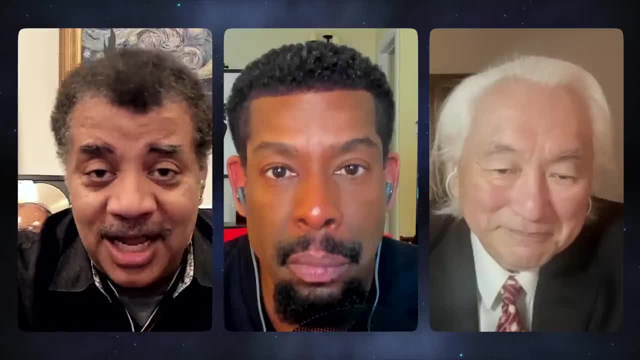 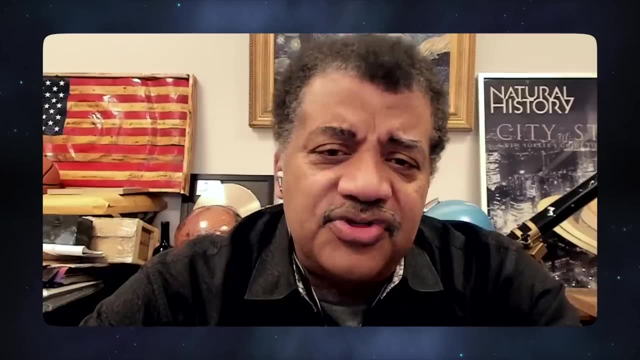 communities and made it to people's desktop and then their laptop and then their pockets, And that clearly changed everything. So so should we fear this change relative to any other? I think that other change was quite welcomed by people. Was it because it was slow and we got used? 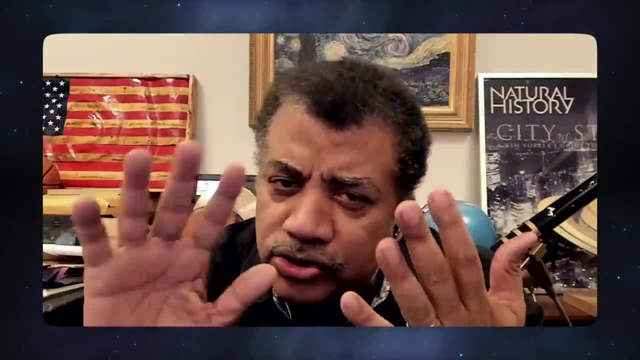 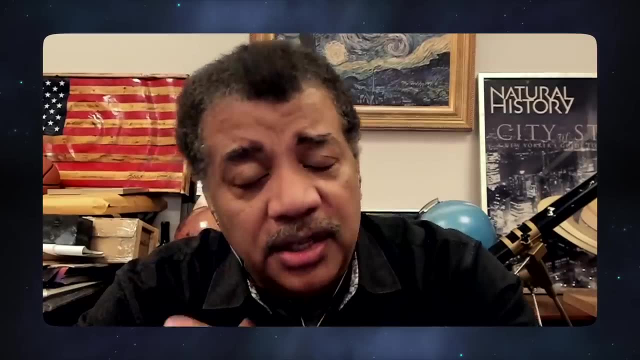 to it or because we saw what it could do and understood what it can do. How would you, how would you characterize it? How would you characterize this shift compared to the one we've all entered already? And does it? and is the military looking for this? for the same reason they did the first computers. 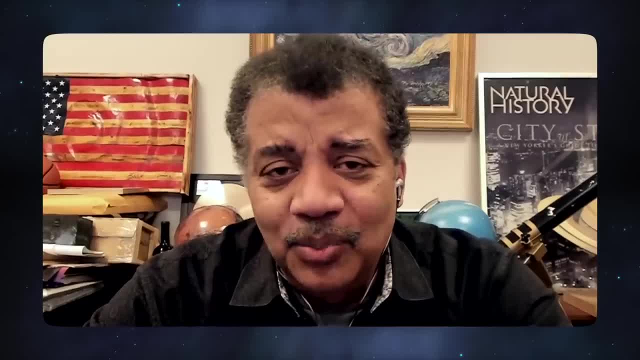 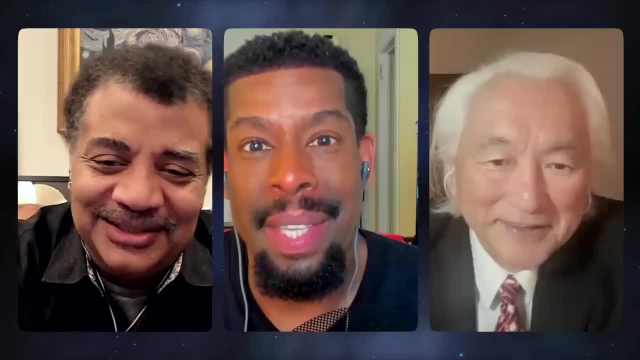 that, that that we talked about in the second stage. Chuck, what do you think? What do you think? Want to grow to grow flowers with it? Well, I mean, We're talking about the US Pentagon, dude, I guess. so, God, that's, that's, that's frightening. 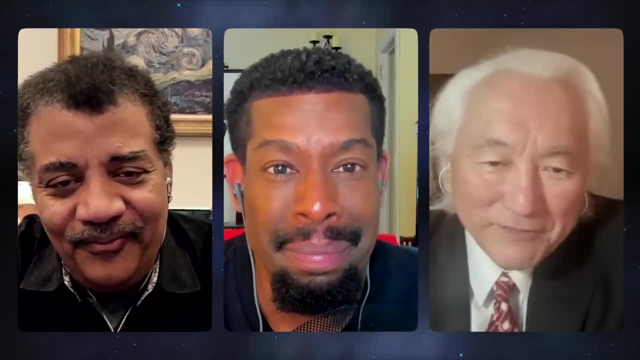 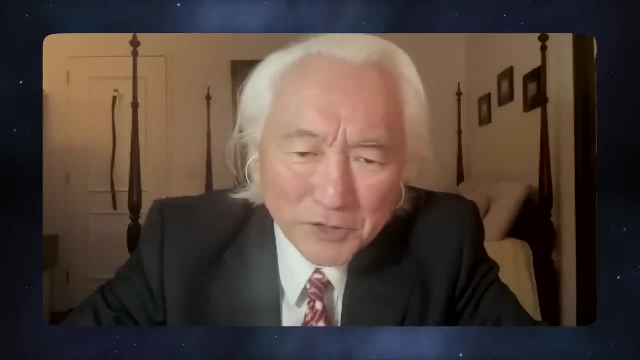 So, Michio, where are you there? Well, first of all, everyone's interested in the. the CIA is very much concerned about it Because they are so powerful. These quantum computers can crack any known digital code. Oh, So this means the crown jewels, the crown jewels of any nation, with all their top secrets about the. 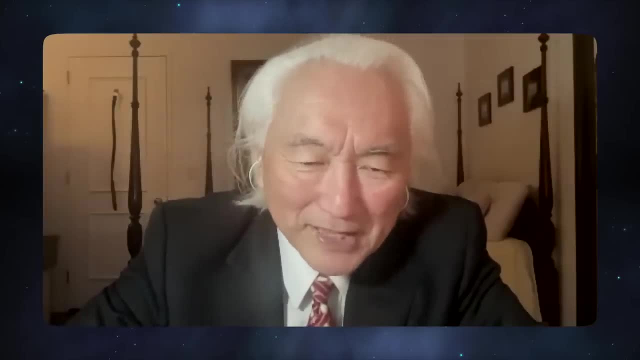 military and defense posture. all of that can be broken into by an advanced quantum computer. But of course everybody else, the sciences and the sciences are to say, because this means better cars, rockets, food, energy We're talking about. 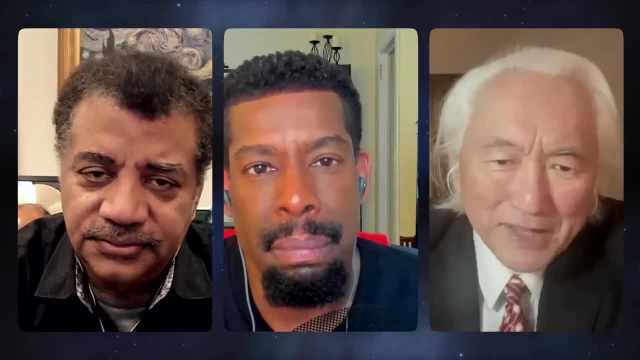 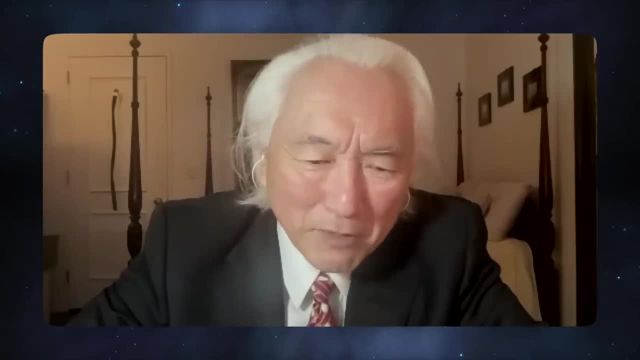 unveiling the secrets of the Big Bang, the understanding of black holes, neutron stars. In other words, everything is going to be affected when we can multiply the power of digital computer by a factor of millions to billions. So we're talking about a new era in computation that'll change everything. 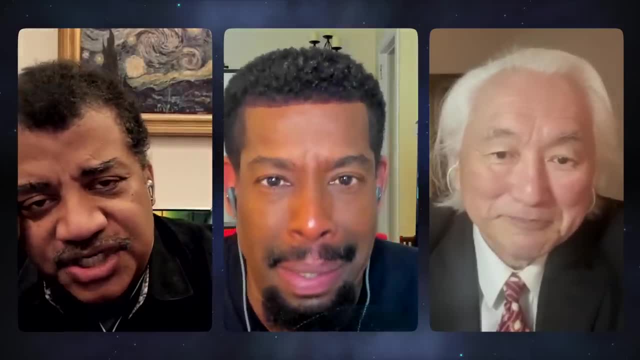 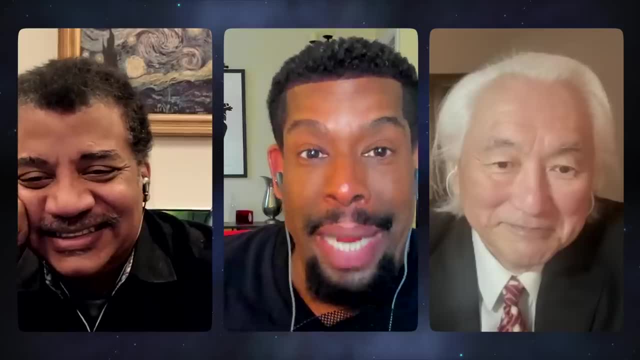 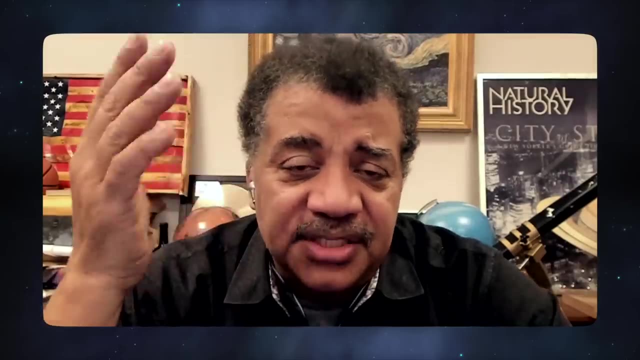 I know I don't even want to ask them at this point. So so one last question. We've all heard of quantum bits, of zeros and ones. all right, This is the binary nature of classical computing. Let's call it that. 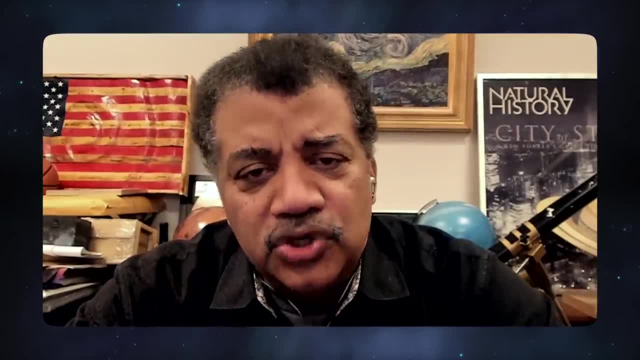 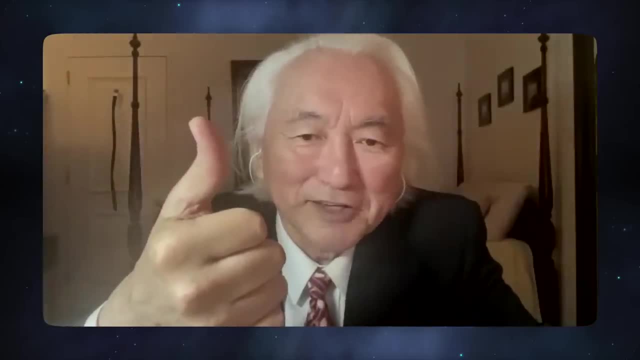 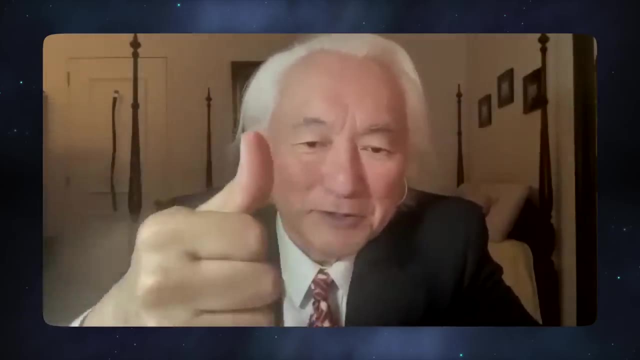 So could you tell us? I've heard the term qubit. Could you tell us how a qubit differs from a bit? Well, think of a spinning top, like an electron: They can spin up or spin down. This is one, this is zero, and that's how electricity can be used to calculate zeros and ones. zeroes and ones. 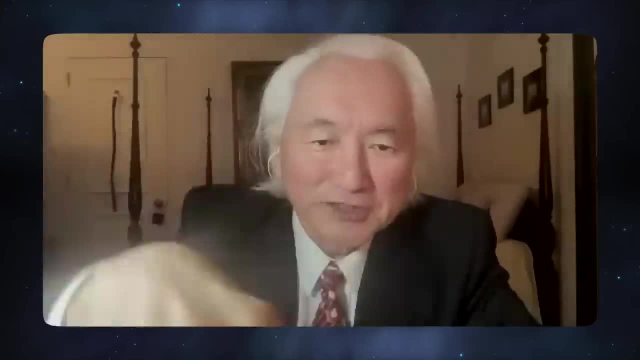 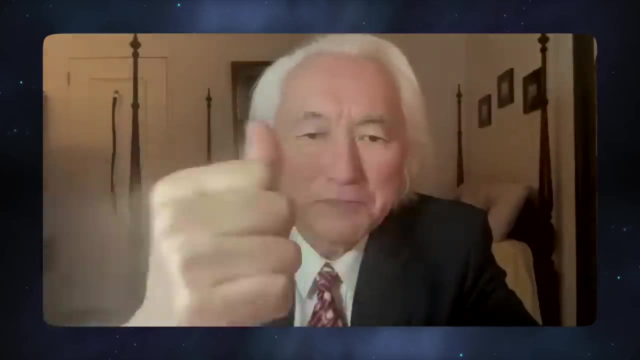 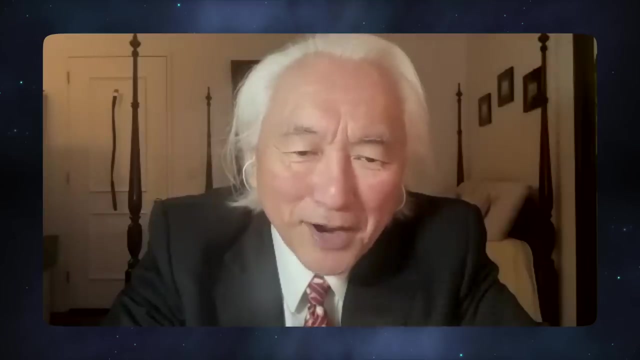 Now let that spinning top spin in all directions simultaneously. So not just up or down, Not just up or down, but in between simultaneously, with all positions. How much more powerful is that than an ordinary digital computer? An infinitely more powerful paradigm shift. 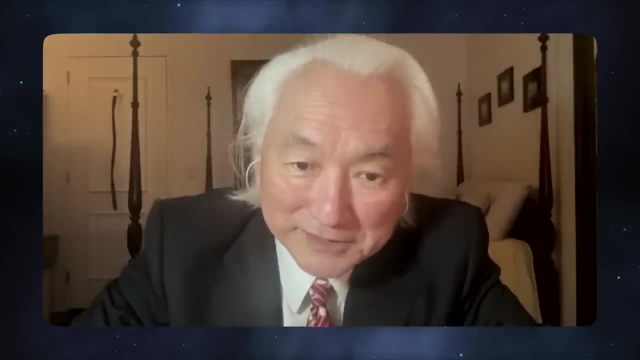 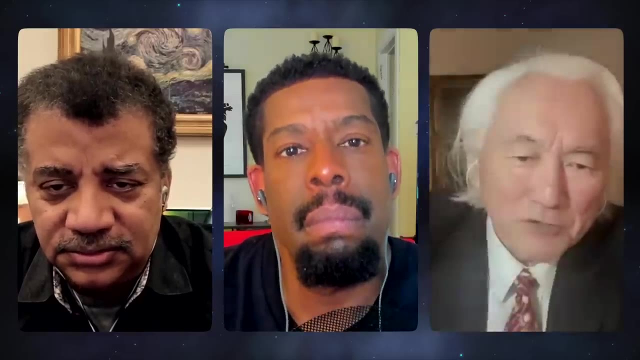 And these electrons compute in parallel universes. universes, because these electrons are simultaneously rotating in all possible directions. Now you cannot be two places at the same time. Electrons can do that, And this is what they live that way. 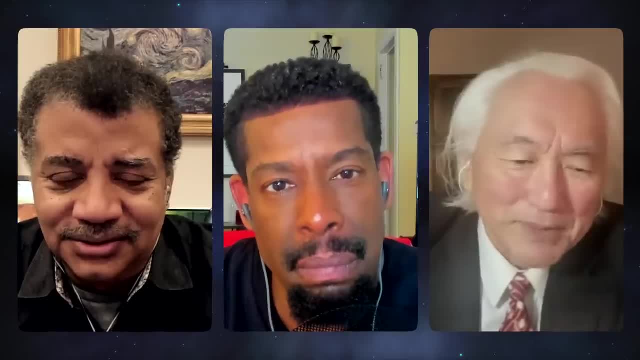 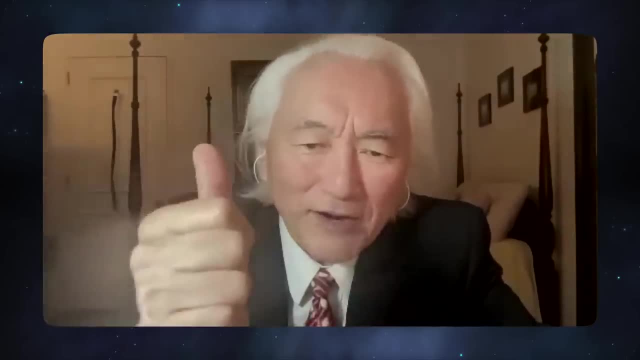 They live that way. Powerful Right, That's right. Electrons can be two places at the same time, And a quantum computer they are in all orientations at the same time. That's why they are infinitely more powerful than a traditional digital computer. 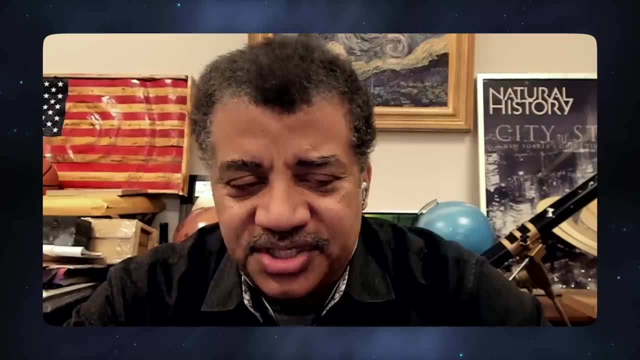 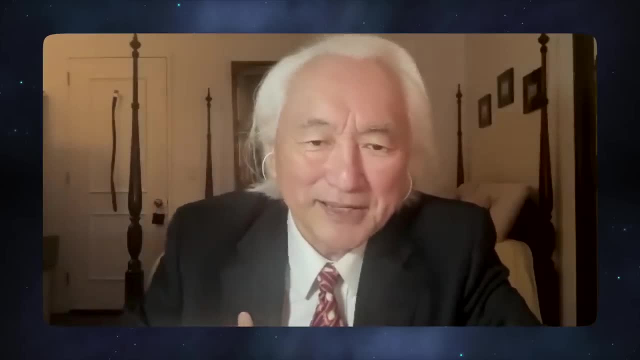 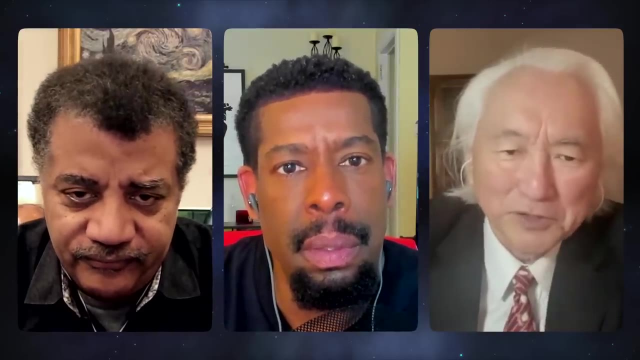 And who uses this Mother Nature? Because that's the nature of atoms, That's the nature of atoms and flowers, and enzymes of the body, and cancer and Alzheimer's. All that stuff is at the quantum mechanical level which is beyond the reach of digital computers. 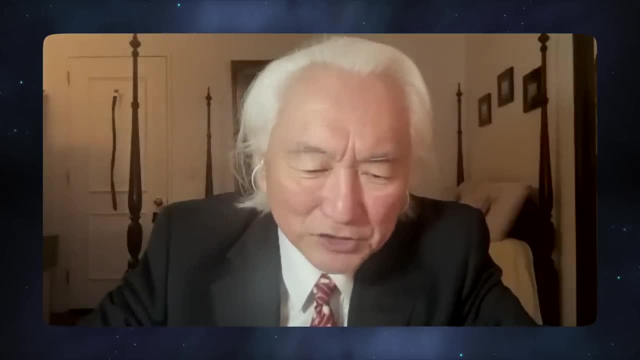 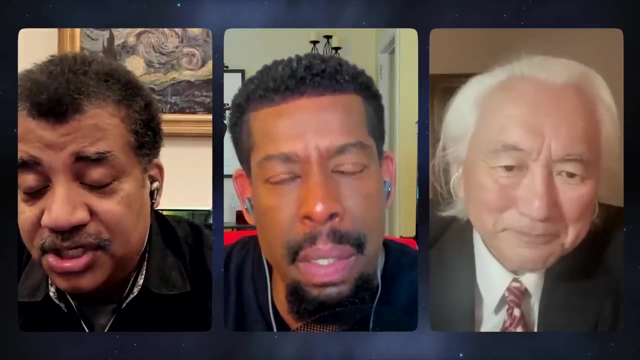 That's one reason why we don't have a cure for cancer, for example. Digital computers cannot model cancer. Quantum computers, we think, can. So, Chaka, just to be clear, Michio kept sticking his right thumb in the air. 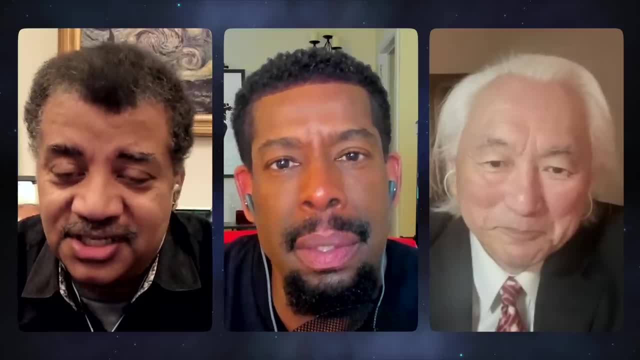 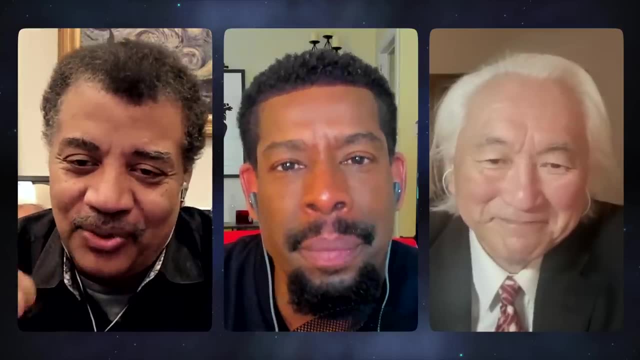 Do you see that? Yes, So there's something called the right-hand rule in physics, which was completely implicit in what Michio's gestures were. Okay, So I just got to untangle that, Michio, before we. So if you put your thumb up right, 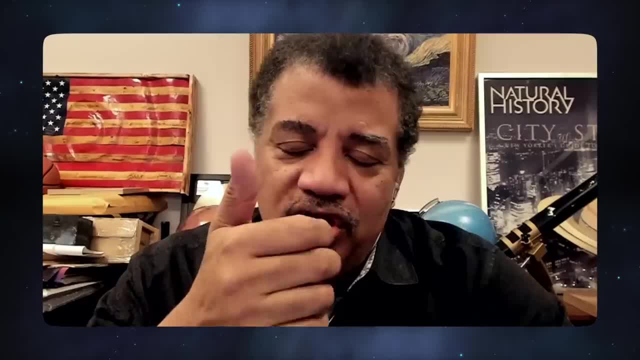 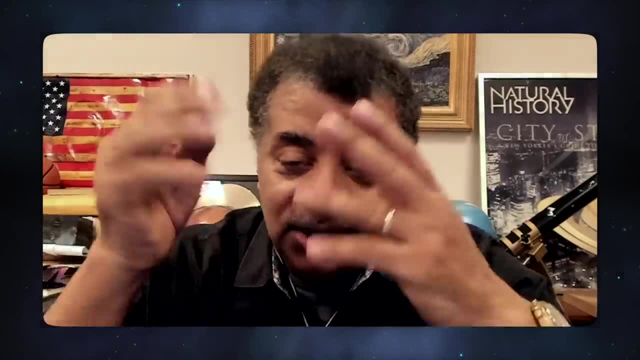 Right And curl your fingers. Okay, All right. So if your fingers are curling in the direction an object is spinning Right, Then your thumb is pointing up Right- I mean in like the north pole- for that object. 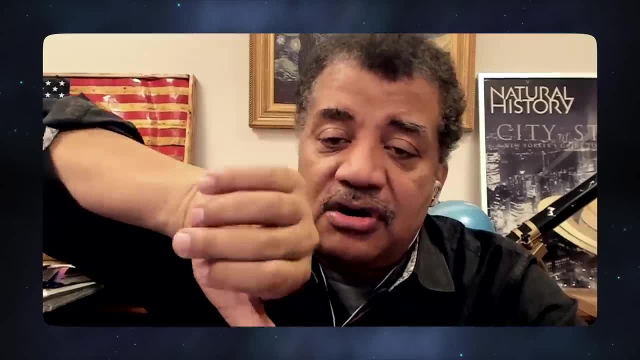 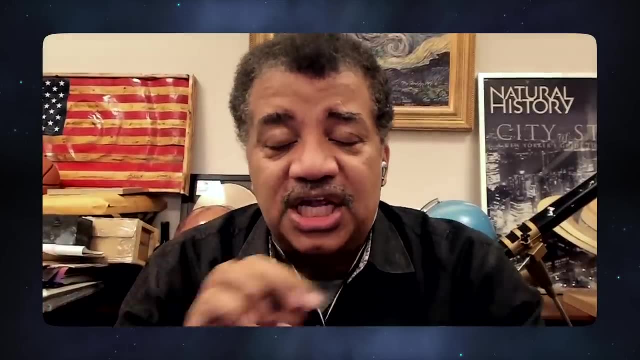 But if you stick your thumb down Up, Then your fingers are curling in the opposite direction. In the opposite direction. Right, That's right, That's right. So that's how we decide which way things are rotating for everything in the universe. 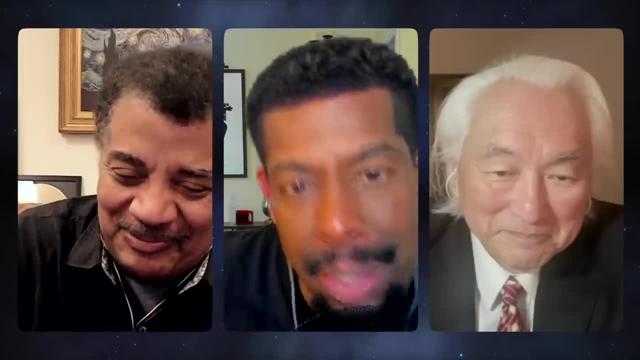 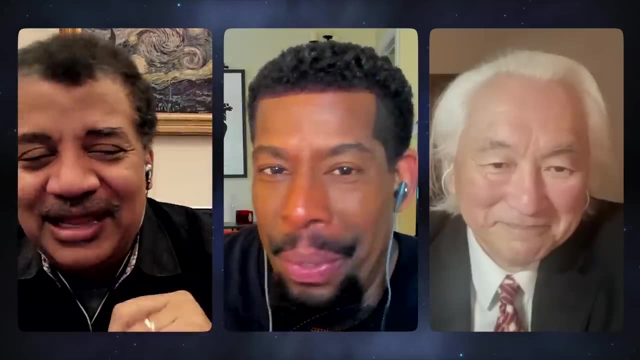 Is it rotating? if it had a thumb, Is its thumb pointing up? I was going to say it's a good thing pigeons didn't discover this. Yeah, who knows what that rule? We call it the different rule. I mean it's a completely different rule. 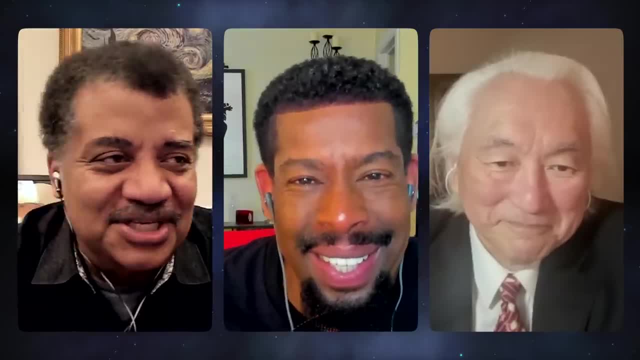 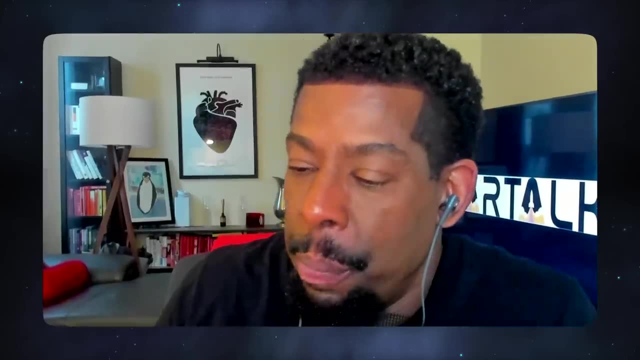 Yeah, thumbless creatures. What kind of physics did they invent, Michio? All right, So Chuck. So let's start off with some questions here. All right, Here we go. Plenty of curious people here on the Patreon portal sending us their questions. 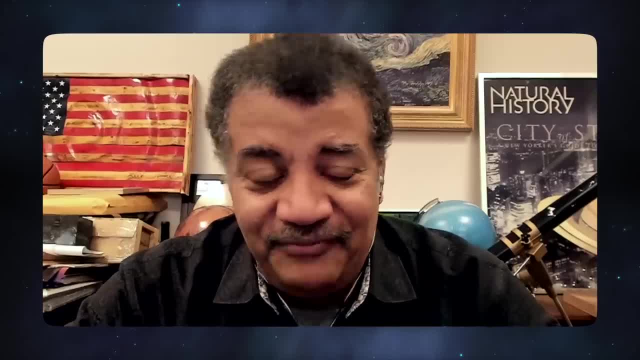 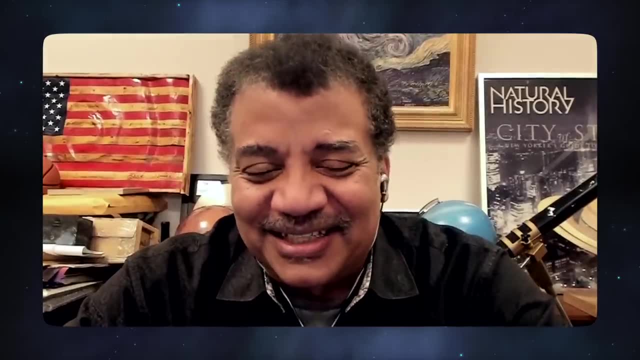 And we will start with our old friend Violetta. Violetta, Cool. She says hello, Uncle Neil, Uncle Chuck, Dr Kaku, Excellent. She says: this is Violetta here, Violetta Rohr, 14 and a half year old astrophysics kid. 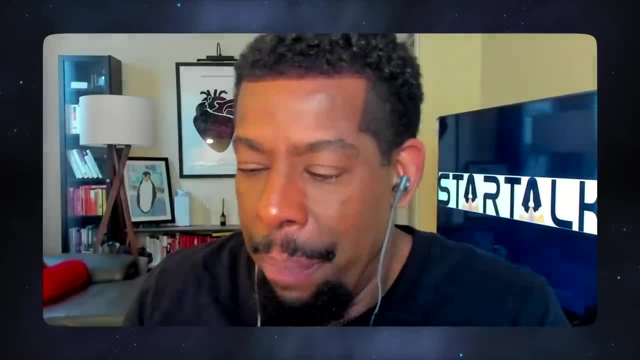 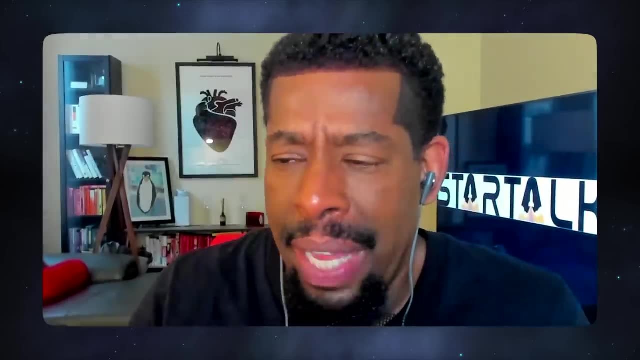 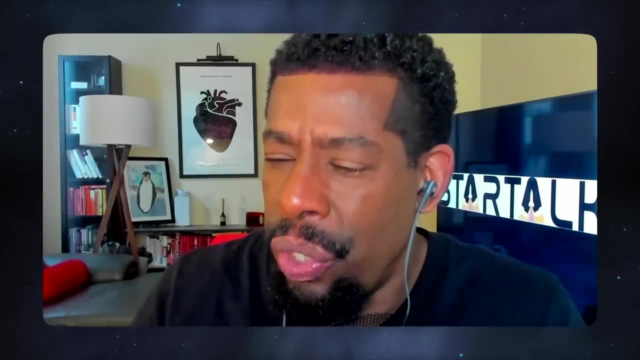 14 and a half writing from Washington DC. I'm keeping it simple this week. Quantum computers are said to harness the laws of quantum mechanics to perform certain calculations exponentially faster than today's supercomputers. What are those calculations? 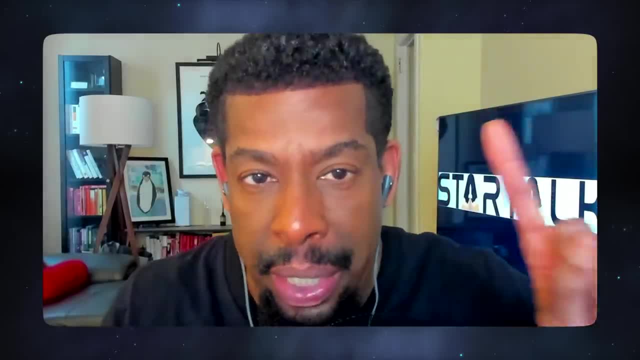 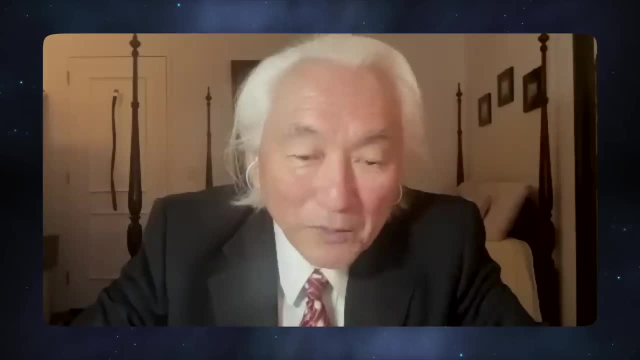 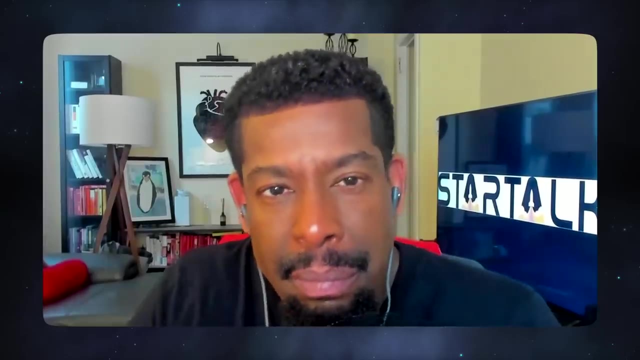 And what could their technical applications be to? and here's the rub, specifically astrophysics: Mmm, Mmm. Okay, well, I got into this quantum computing game because I work in something called string theory, Mmm, which we think is the theory of everything, including the Big Bang. 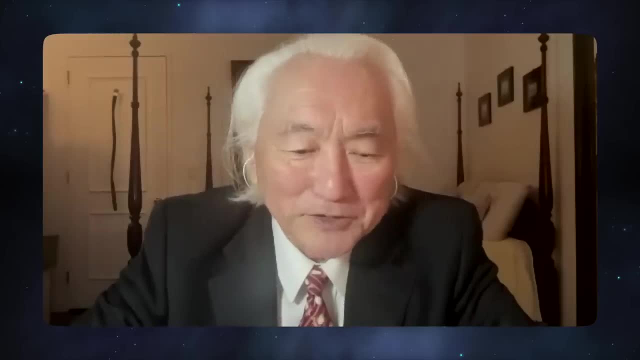 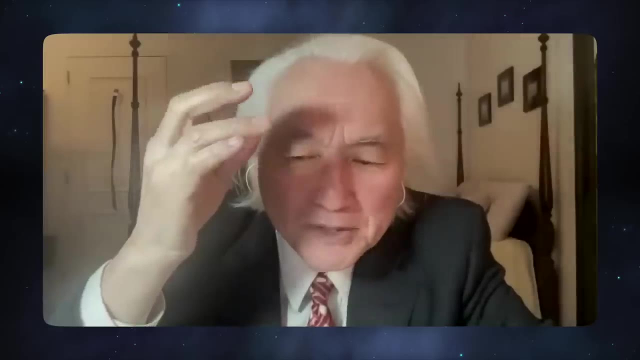 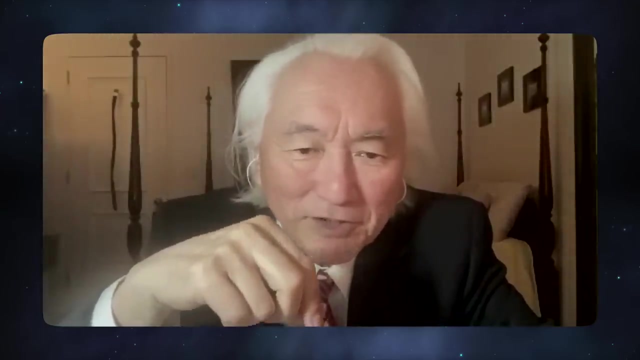 But string theory is so complicated and so complex no human has been able to use their mind to solve it. Now, when we look at a proton, how do we solve the mechanics of a proton? By hand? No, by computers. Lattice-Gaiss theory allows us to solve the properties of a proton. 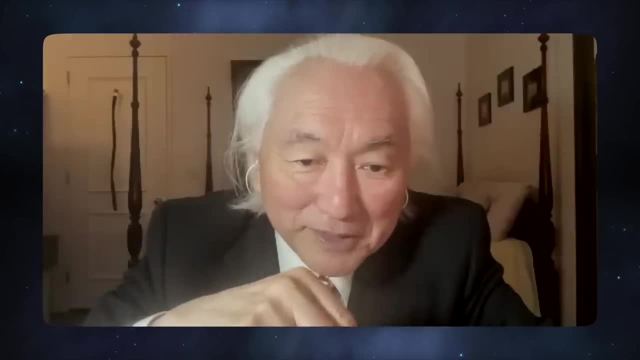 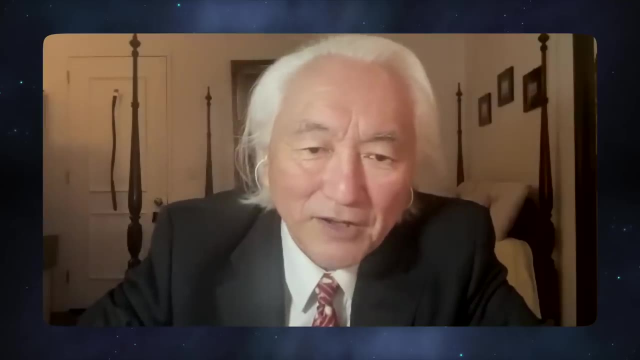 We use computers at the fundamental level. So I think that for the Big Bang, to calculate what happens at the center of the Big Bang, the center of a wormhole, whether or not time travel is possible, whether or not parallel universes can be visited, 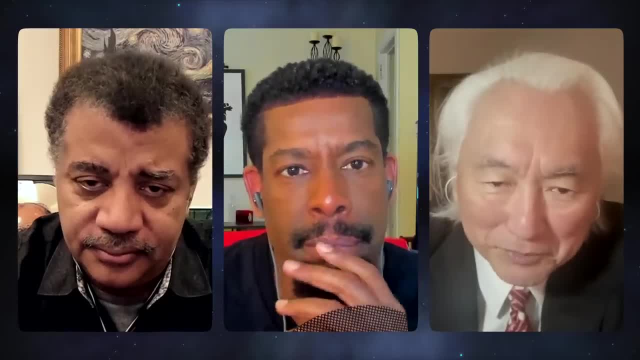 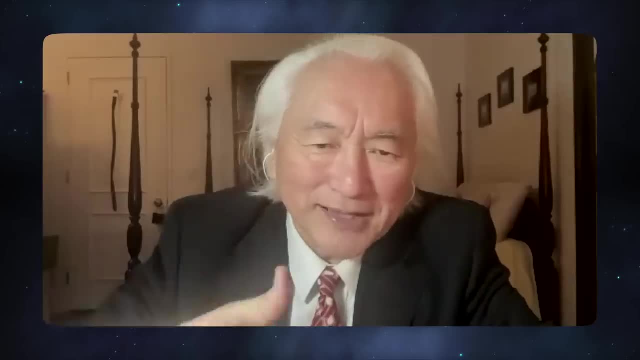 all these questions can be solved using a quantum computer rather than a digital computer, which computes on zeros and ones and zeros and ones. And that's how I got into it, Because I think in astrophysics there are so many problems that cannot be solved with a digital computer. 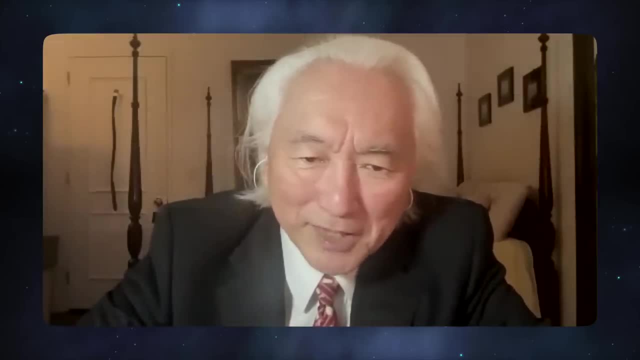 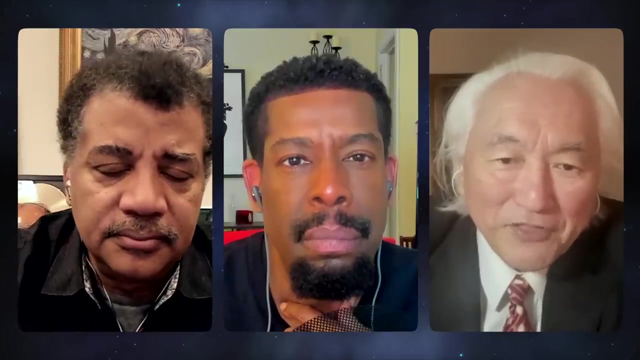 For example, we know that the sun explodes. sometimes it releases a coronal mass discharge. In 1859, it just wiped out telegraph wires throughout North America- the Carrington event. Quantum computers may be able to model that event, So we can predict the next Carrington event when the sun goes berserk. 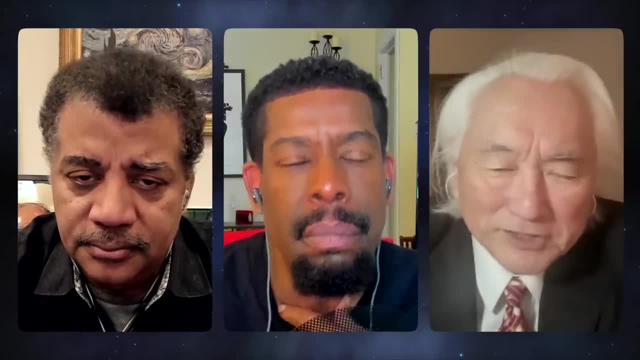 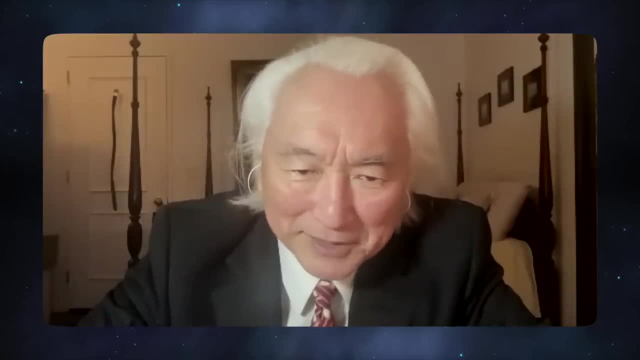 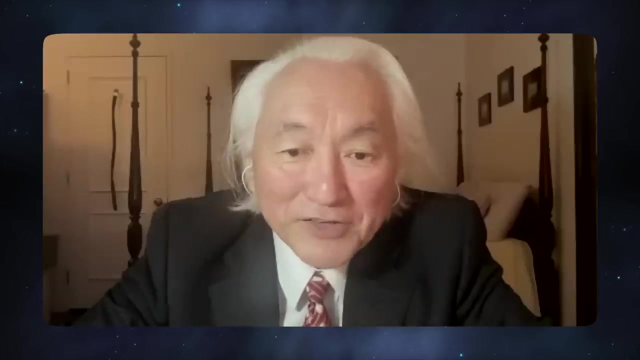 and shoots a tremendous coronal mass discharge at the planet Earth and wipes out all communications, causing at least two trillion dollars in property damage. Everything that's floating above us, satellites and all that crap will just get wiped out, Including power plants on the surface of the Earth. 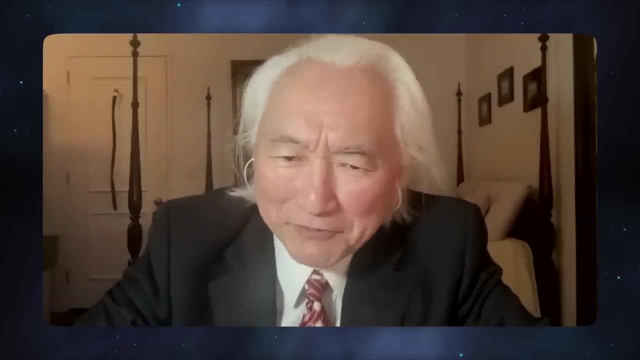 We're talking about a blackout, a planetary blackout. We've never had that before: A planetary blackout where every single nation on the planet Earth has its power wiped out simultaneously. Therefore, there's no rescue crews, no ambulances, because they're out too right. 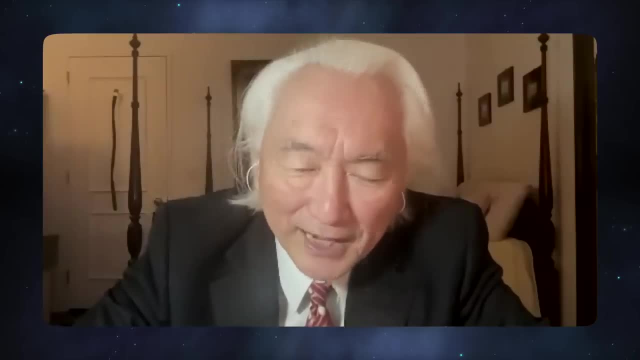 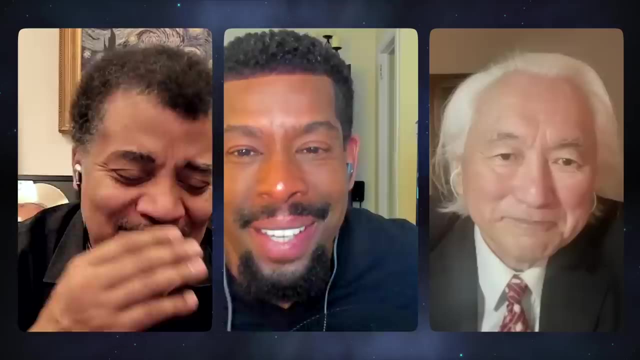 The entire Earth is the infrastructure. Electrical infrastructure is wiped out by, in other cases, the Carrington event, And we're helpless. And that's our show people. I know that's what I'm saying. Good night, Enjoy your evening. 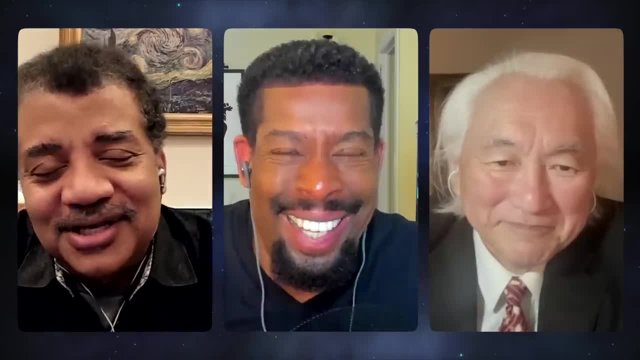 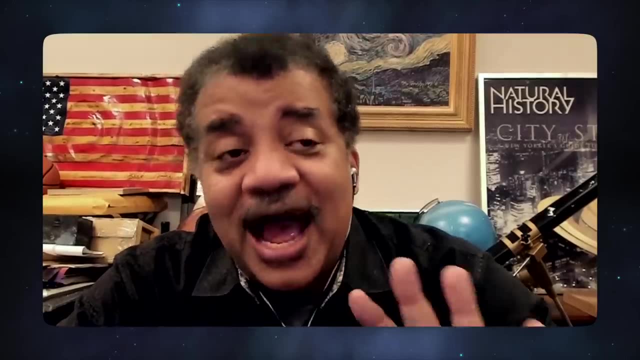 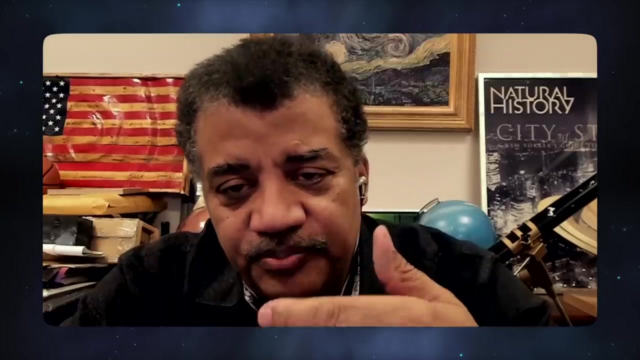 Kiss your ass. goodbye, Right. So, Michio, I'm reminded that you're like the king of disaster scenarios. I've forgotten. Thanks for reminding me about that. So a couple of things. Let me just sort of put some further punctuation on what you just said. 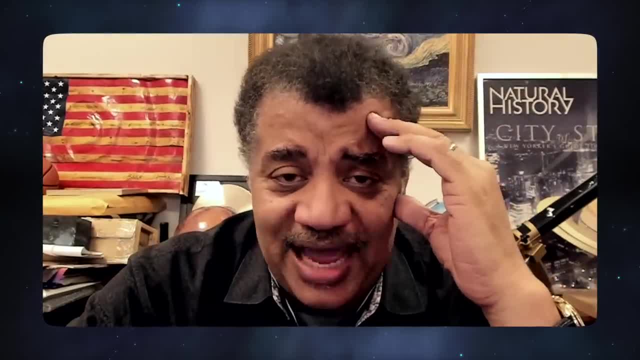 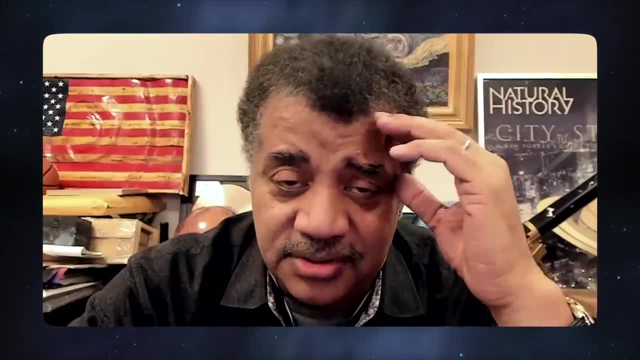 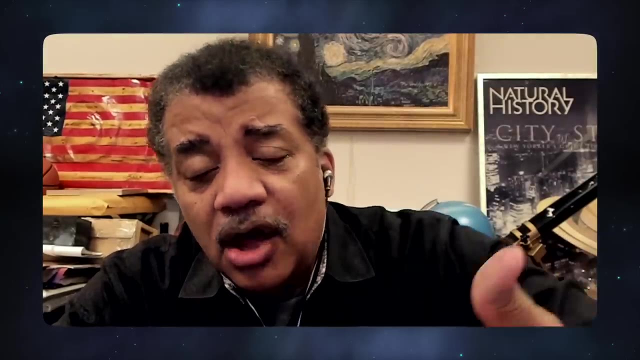 The sun is a roiling mass discharge. Right It's a plasma with free electrons roaming among mostly hydrogen and some helium and some other trace elements, And there's a magnetic field coursing through it that's getting dragged around the surface because the sun is not rotating as a solid object. 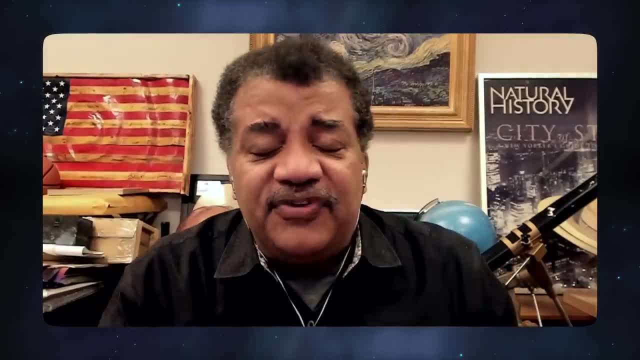 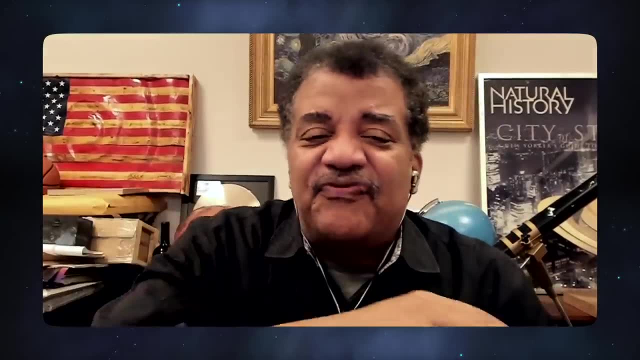 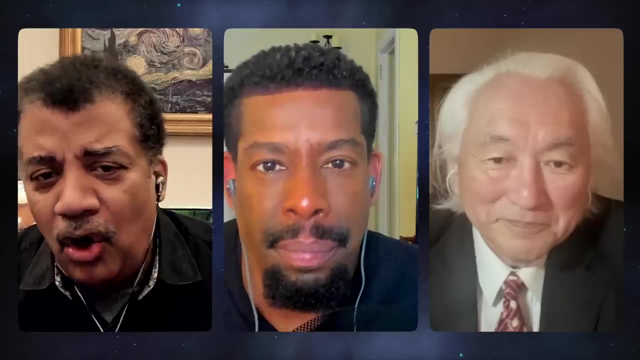 So the magnetic field is embedded in the plasma, That magnetic field is getting stretched in all directions and then there's a point where it snaps, It flings material with it and all we could do is watch. And, Michio, if we could calculate all the stuff that's happening there. what a boon. 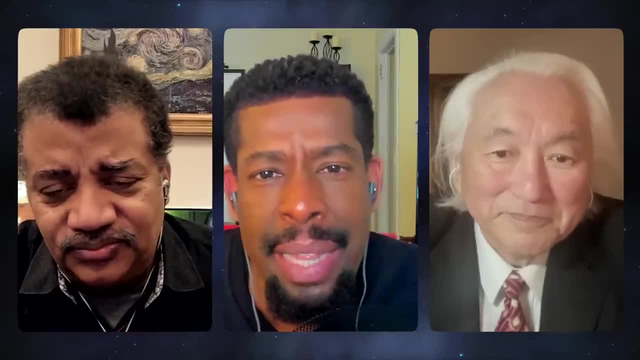 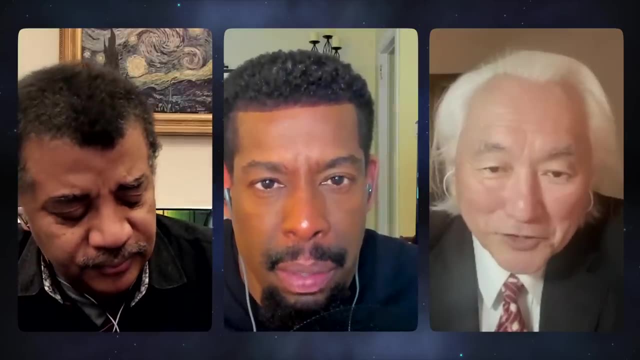 that would be to solar physics. So now, is that different than a solar flare, or just bigger than a solar flare? This is much bigger than a solar flare. This is the mother, the mother of all solar flares, capable of wiping out all power supplies. 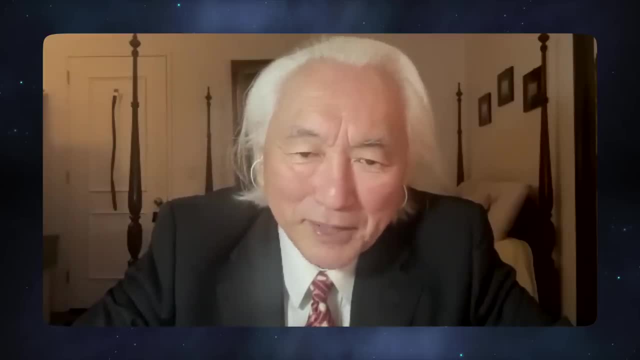 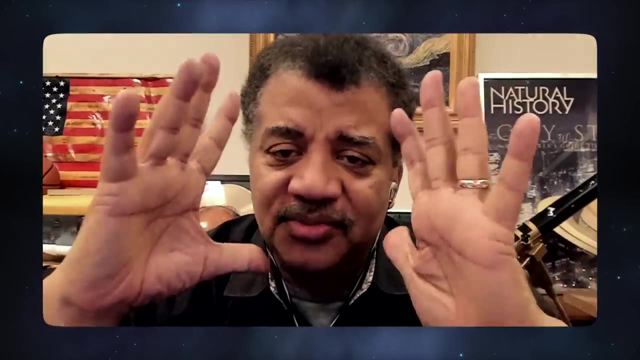 in on the surface, In outer space surrounding the planet Earth. We're talking about shutting down civilization as we know it. Wow. So it's a matter of scale of energy, Chuck. Scale of energy. Yeah, It's energy, Yeah. 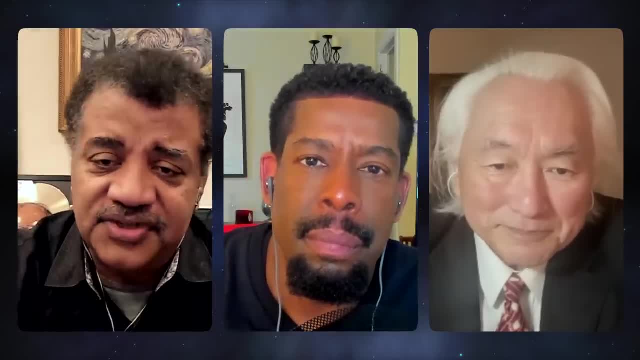 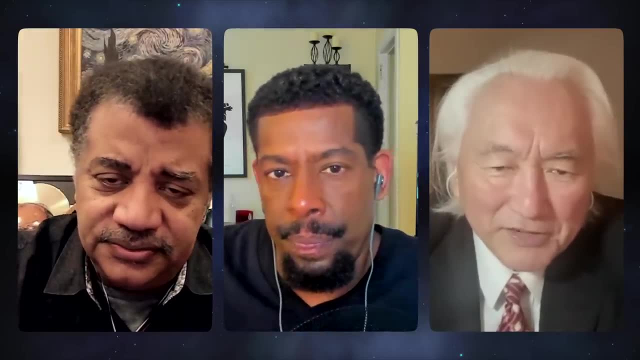 It's just right. And we have evidence in relatively recent past, right 160 years ago, where this actual with Carrington event- right, That's what it was called in Michio, That's right. And even before that, 700 AD, 800 AD- this has happened before. Again thousands of years ago, Yeah, But we can now track these Carrington events even into the past. Wait, Their computing didn't collapse in 700 AD. Yeah. What evidence do you have? How do you think we got back to this point? 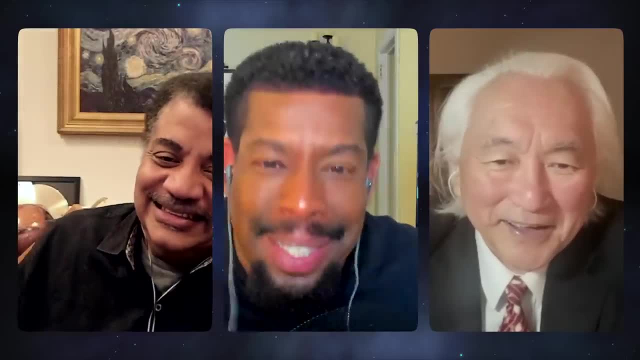 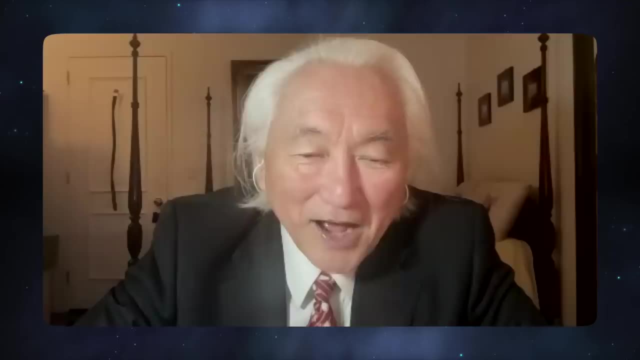 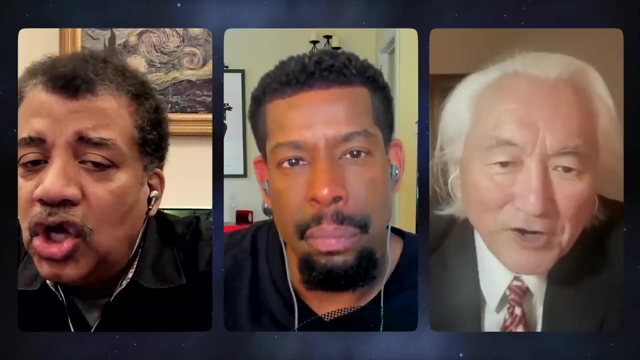 All this time we've just been working back to this point, Back to AD 700.. How do you know it happened in AD 700? Because several things. The radiation affected tree rings- Oh Yeah, Tree rings. Oh, It also affected the Arctic. 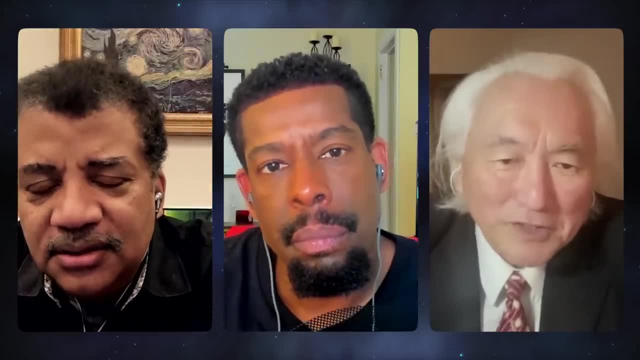 Ice cores, Arctic ice cores- Oh, of course. So by looking at ice cores and tree rings you can see there was a disturbance in 700 and 800 AD. Wow. And of course there was no electricity back then. Right. 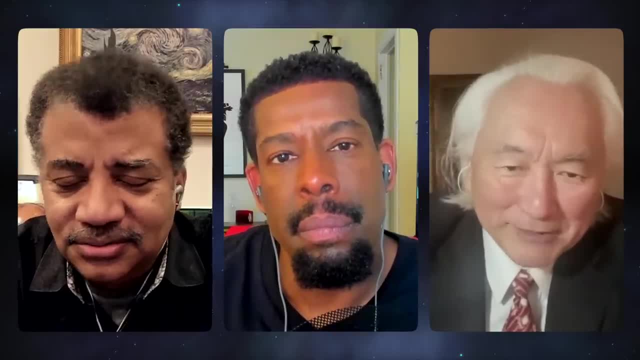 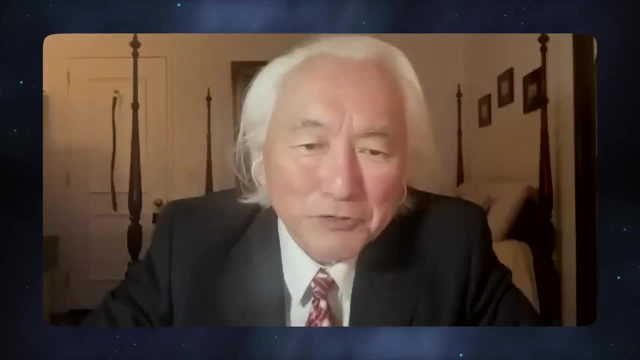 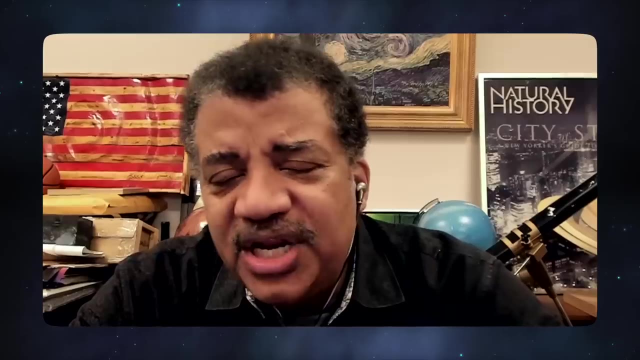 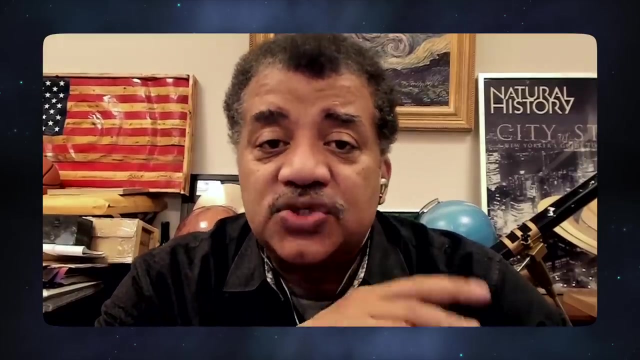 Right, It'd be a horrible mess And we're powerless, but we do know it happened in the past And that's where quantum computers can calculate- we hope calculate- some of these disasters. We need a backup plan to have civilization restart itself, such as how we lived before. 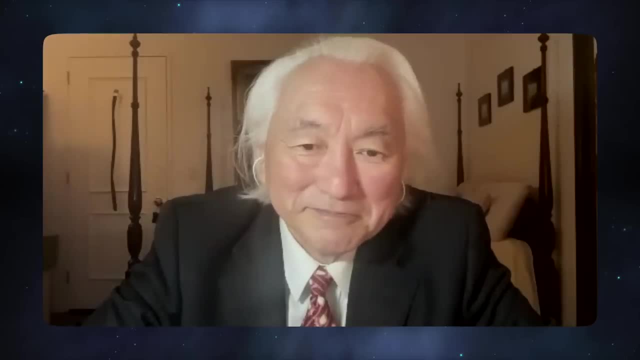 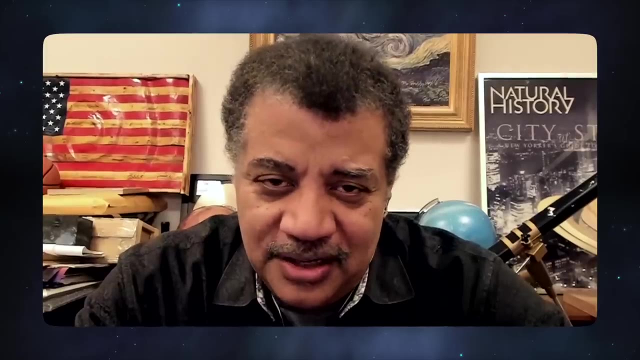 there was electricity, right? That's right. We are with my good friend and colleague, Michio Kaku, professor of physics at the City University of New York, and we're talking about quantum computing, As described in his current book. what did you call it, Michio? 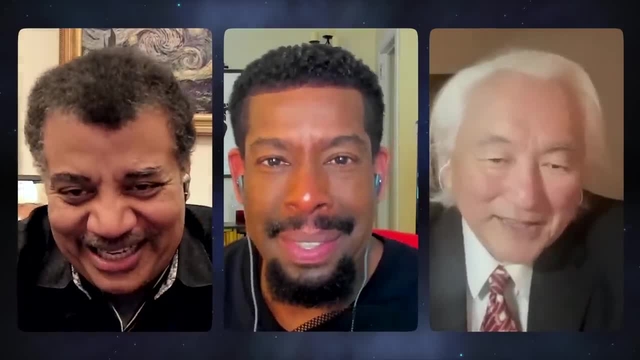 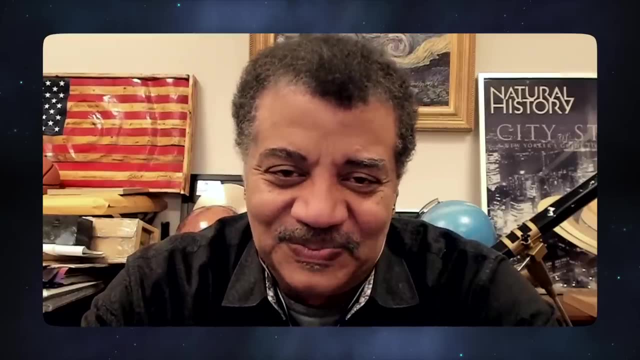 Quantum Disaster. Quantum Supremacy. Oh, Quantum Supremacy. Okay Yeah, That was coined by a physicist at Caltech. All right, It's his word. We'll get back to that when we return on StarTalk. We're back. 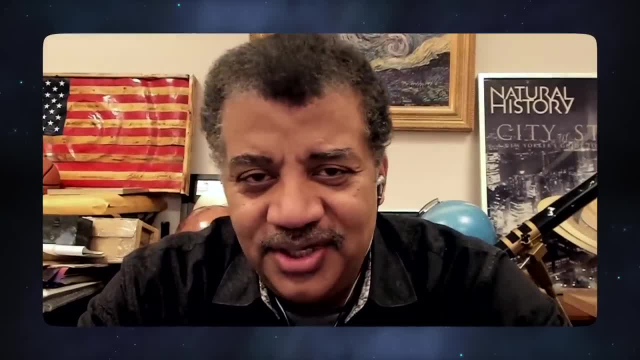 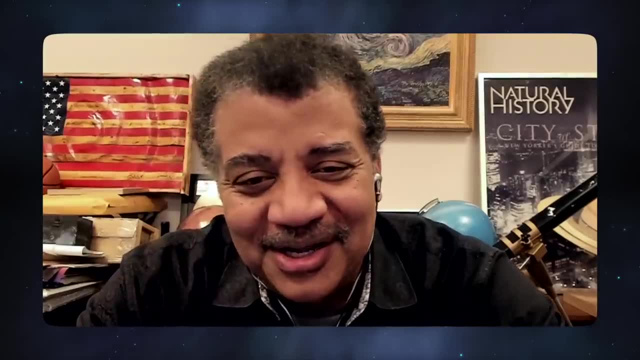 StarTalk- Cosmic Queries. Quantum Computing is back. We're back. Quantum Computing is the subject and we've got a man who wrote the book, a book on quantum computing, Michio, you call it Quantum Supremacy and just before the break you said that you're. 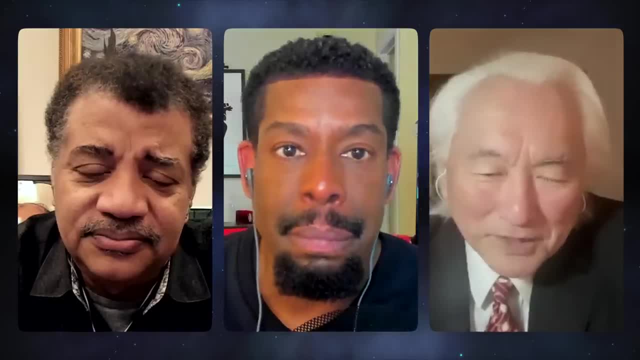 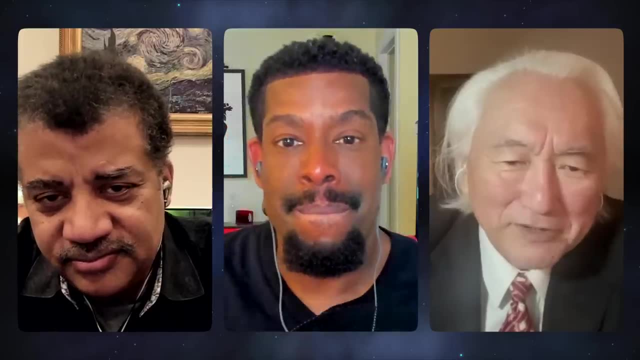 quoting someone who called it that. Who was that? Yeah, Joel Preskill at Caltech. You see, people used to think that quantum computers could never, never rival a digital computer. So Quantum Supremacy is the point at which a quantum computer can be used. 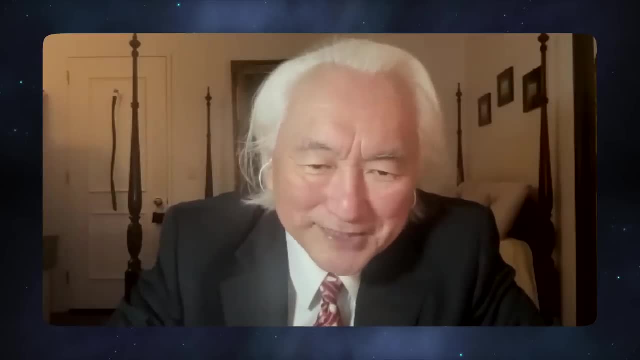 It's the point at which a quantum computer can be used. It's the point at which a quantum computer can beat a digital computer on certain tasks. Two years ago, the Chinese and also Google built quantum computers that were millions of times more powerful than a standard computer for a specific task. 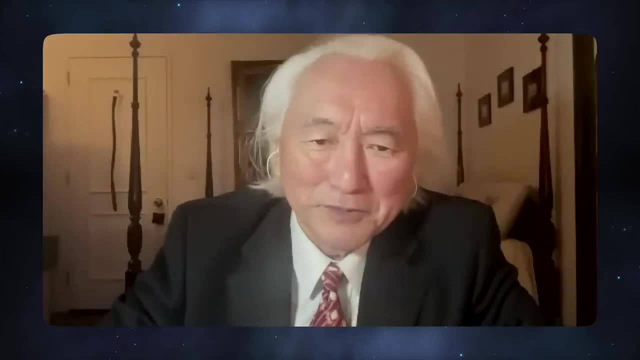 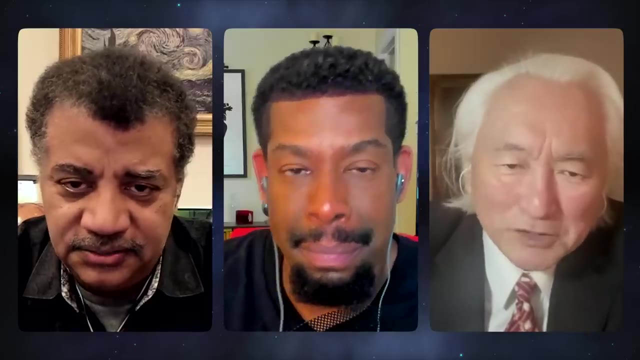 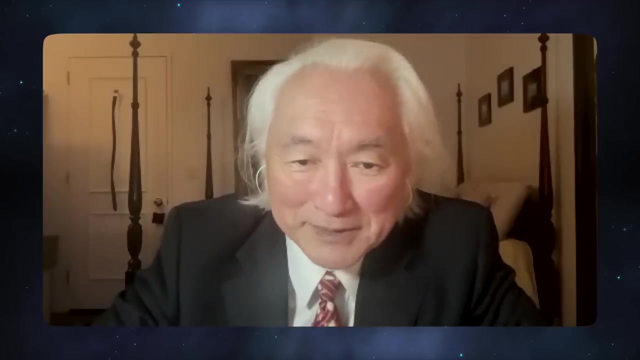 The next step is to make an all-purpose quantum computer that can outrace a general computer on all possible tasks. That's the race. It's a horse race. Wow, Yeah, Yeah, Yeah. I mean, not only are there leaders in the horse race, but IBM is in it. 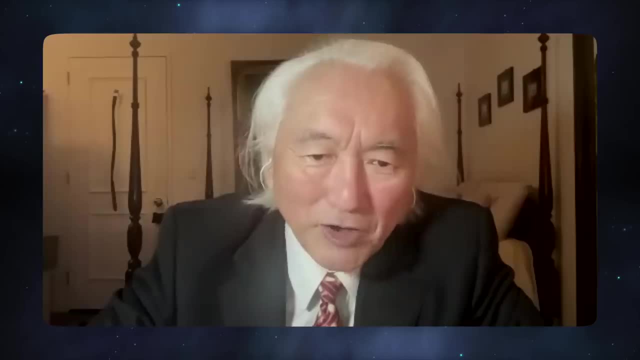 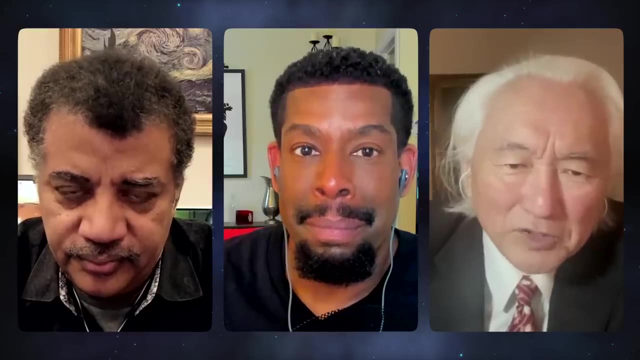 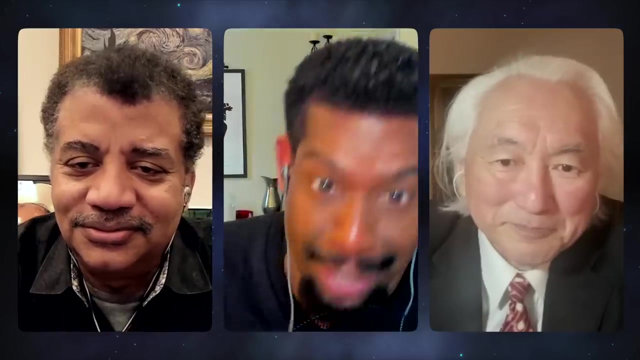 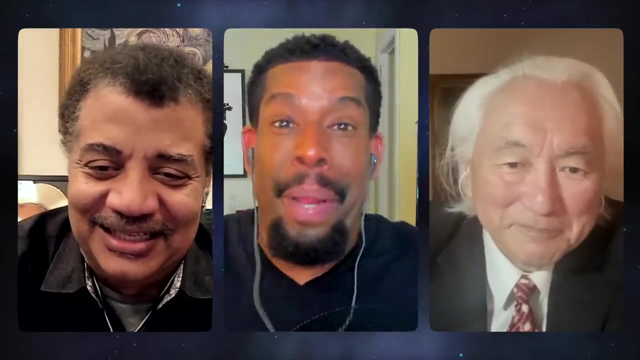 I mean also, Google is in the race, Microsoft, Honeywell. everybody realizes that whoever wins this race will dominate the world economy. Oh man, I'm sorry, but this sounds very Third Reich. I'm just saying. I'm just saying it's like we've got this race that's supremacy leading to a master. 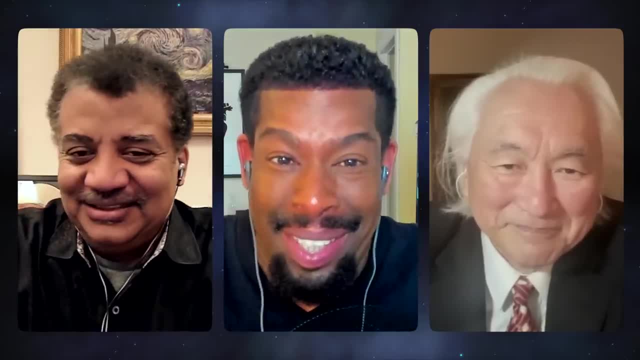 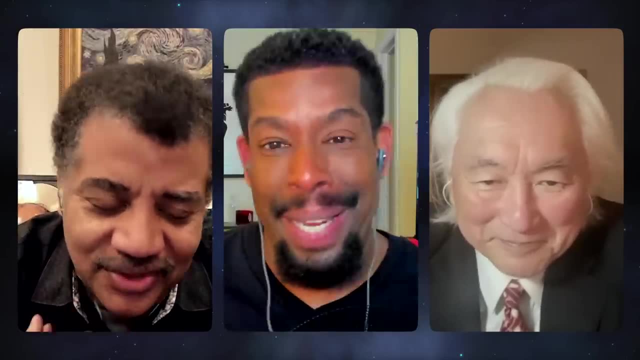 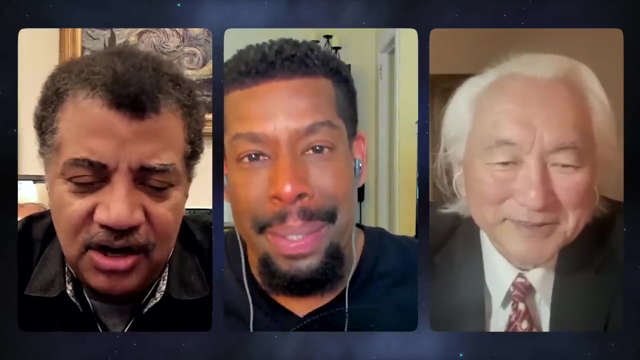 race. It's a little nuts, But, Chuck, it's a computing race, not a race of the thing. All right, That's right. It's computing supremacy, That's right. So, Michio, I actually overlapped with Preskill at the University of Texas. 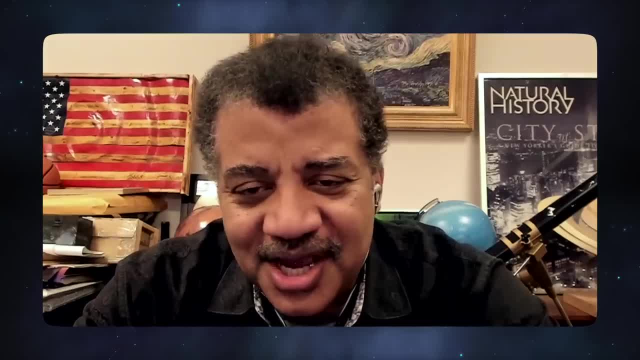 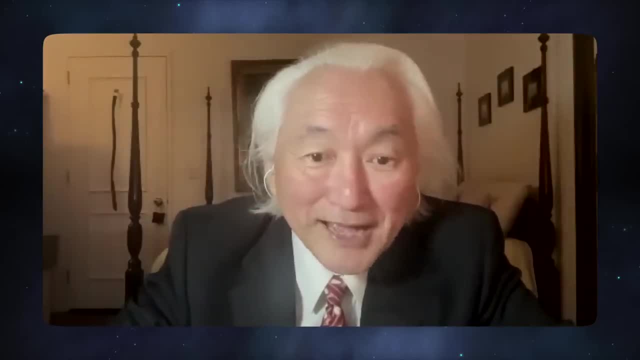 before they snapped him up over at Caltech. Yeah well, he was the one who coined the concept and we actually made it two years ago, and now we're going for the next step, Which is to create an all-purpose quantum computer. 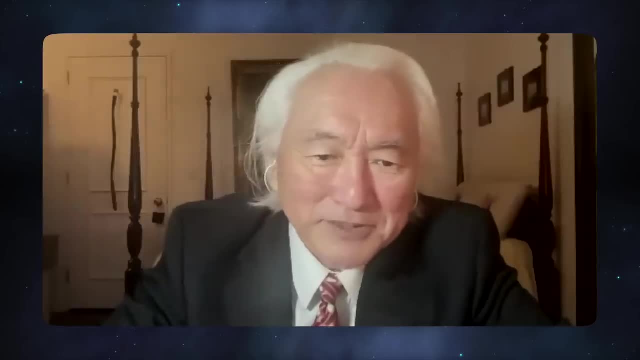 that can handle ordinary problems, problems of medicine, problems of global warming, problems of food production, all the problems that cannot be solved today using digital computers. Or they could be solved, but they would take 1,000 years to run the program. 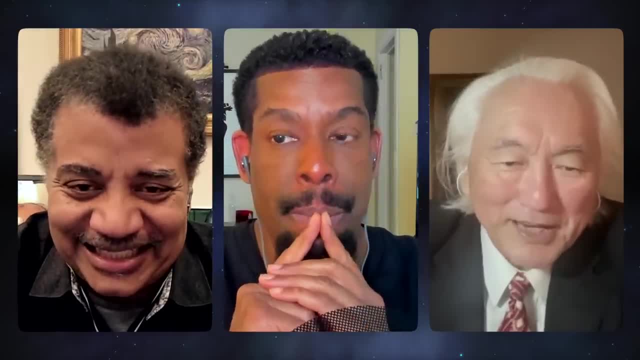 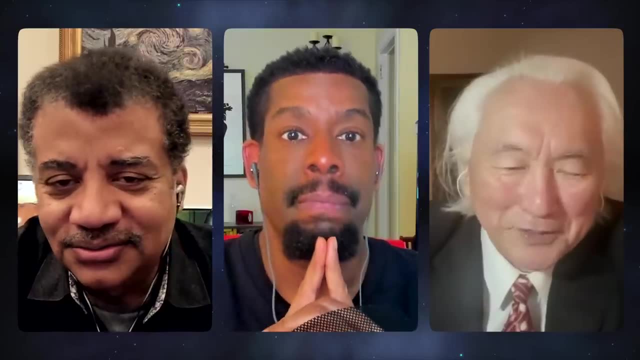 Or infinite amount of time, Or infinite. okay, It would take an infinite amount of time for a regular digital computer to model the electron wave function of a molecule. Okay, But that's what quantum computers can do, You know, I forgot Michio. I forgot about that. 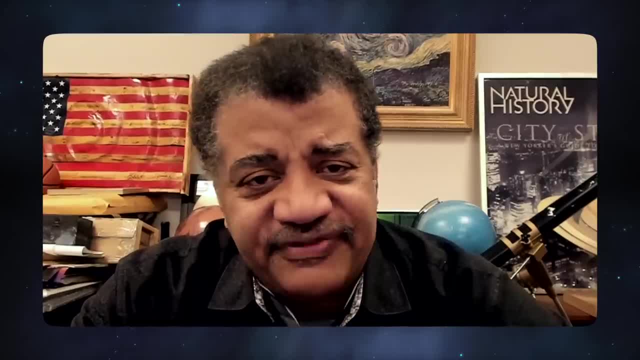 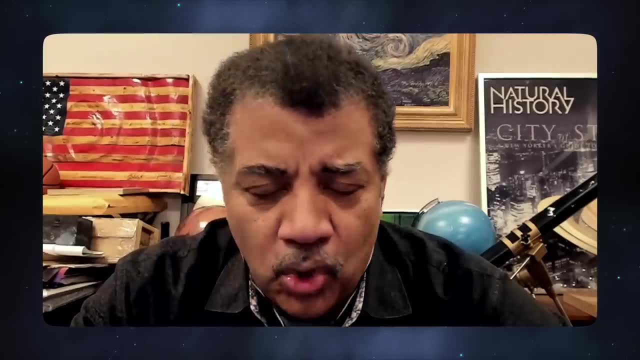 I think we perfectly modeled the hydrogen atom, but after that we just have to approximate, because the atoms are too complicated, Exactly With all the protons and the electrons and what orbitals they occupy and what the shape is. I'd forgotten that, Michio. 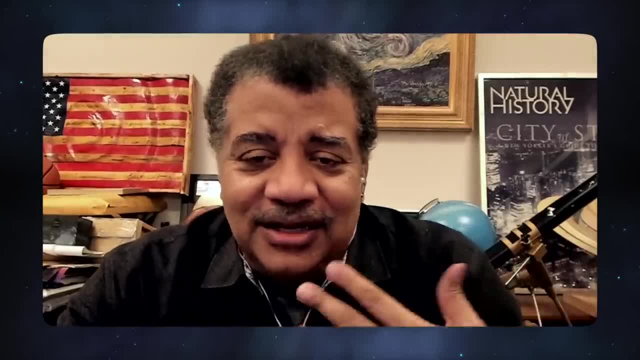 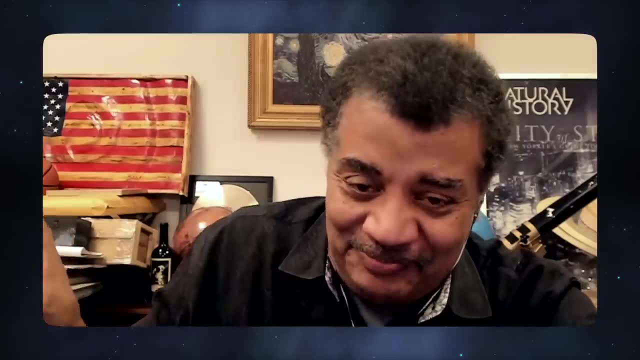 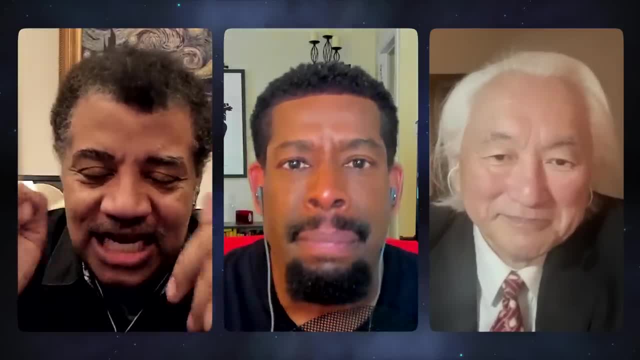 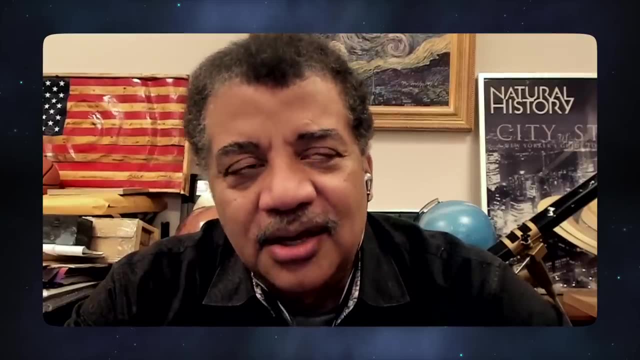 One proton And one electron Right, And it's 90% of the atoms in the universe. Yeah, We're good. I'd never pause to appreciate what you have to go through, Michio, as a physicist. So let me ask you this: 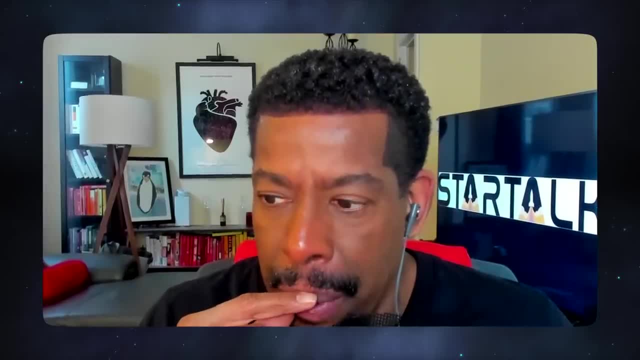 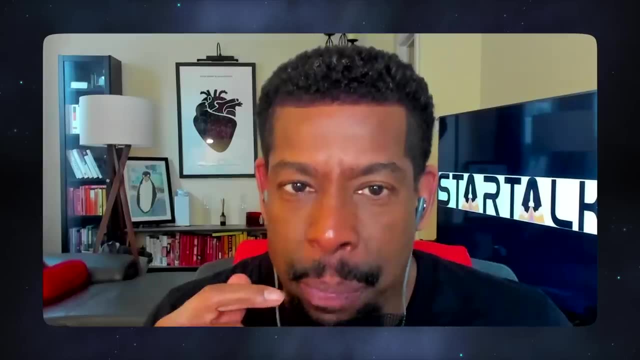 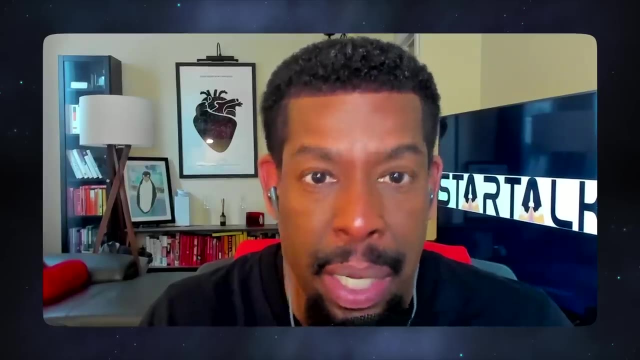 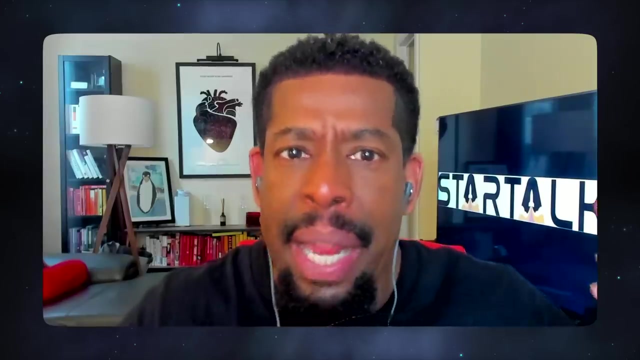 It sounds to me like something this powerful could easily achieve intelligence and then could very possibly, uh, achieve sentience. So you know, just because you achieve intelligence doesn't mean you're sentient, But if you're that powerful and that capable, it's very possible that you could become sentient. 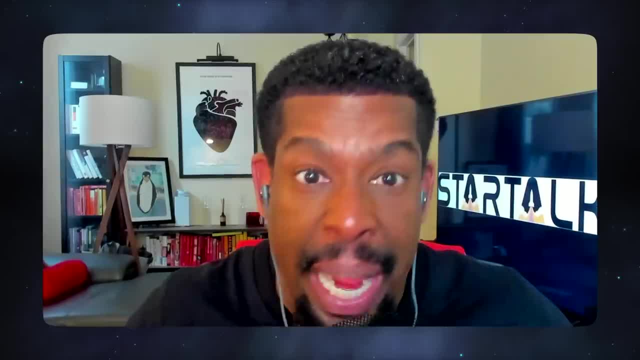 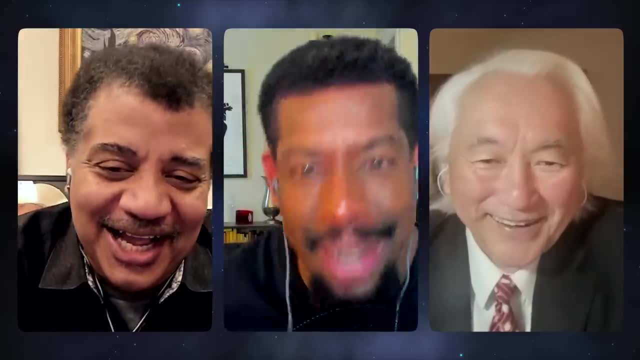 And now isn't that the scariest damn thing that's ever happened since the world has been created? And Chuck, that's a different show. Okay, All right. That's, that's All right. Okay, Forget it. 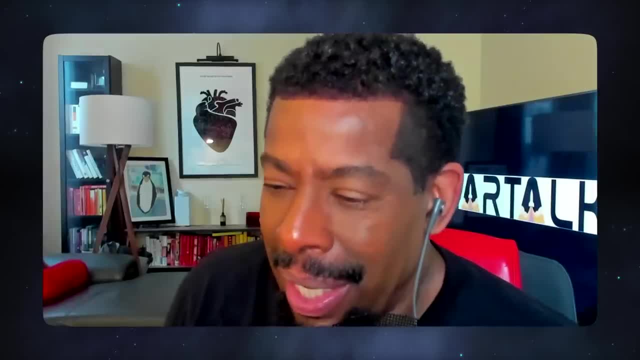 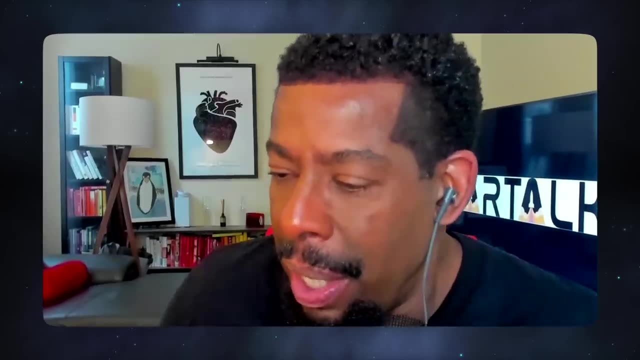 That is a different show, You're right. So, Chuck, Okay, So this is uh Andrei Sibru, who says: uh, I'm sorry. Serbu, who says: hello, my dear brain smoothie makers. 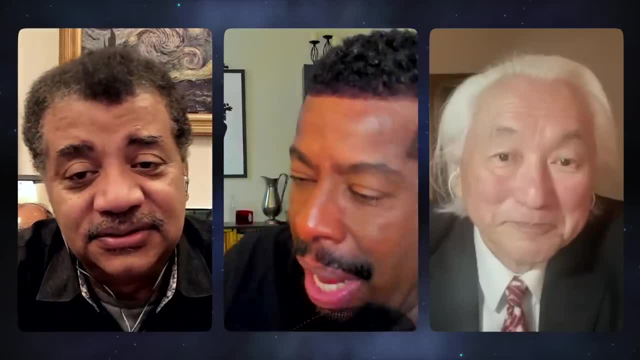 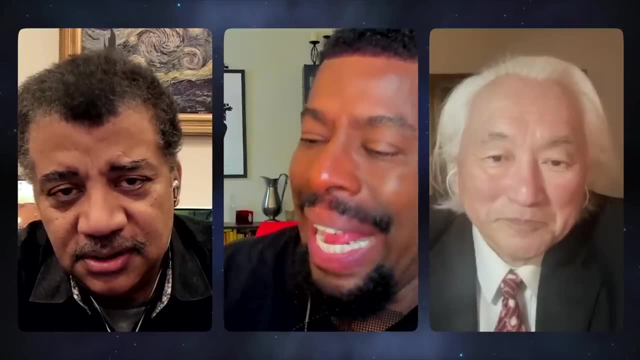 Um, he says as a vampire, non-eternal friend Andrei, from Romania, I've been trying to understand and put quantum computers to good use in the following hypothesis: Wait, did you say non-eternal or non-nocturnal? 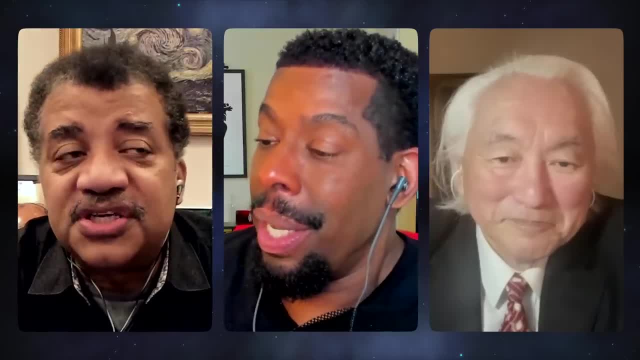 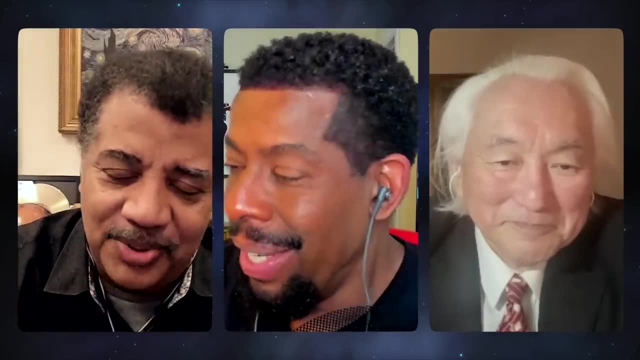 Non-eternal. he says: How do you mean Oh, oh, So he's a vampire that does die. Yes, Because Romania is the original vampire. I think I believe it is Just catch. I'm slow, I'm slow catching up on him. 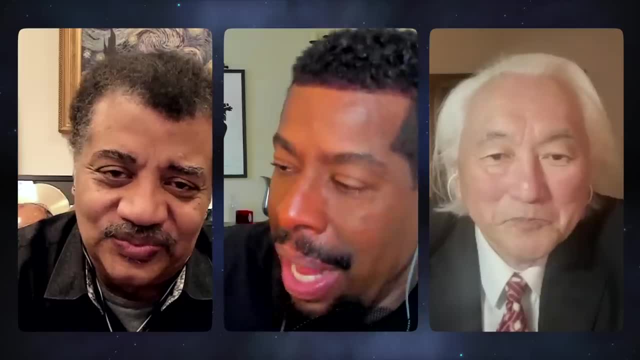 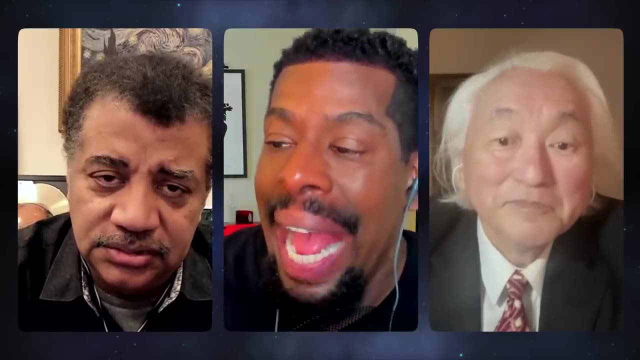 You got it. No, you hit it. You got it. Got it, Okay, Go ahead. Then he says: will quantum, will quantum computers be able to map out and transport our existential information as entities so that we can live eternally inside them and travel at the speed? 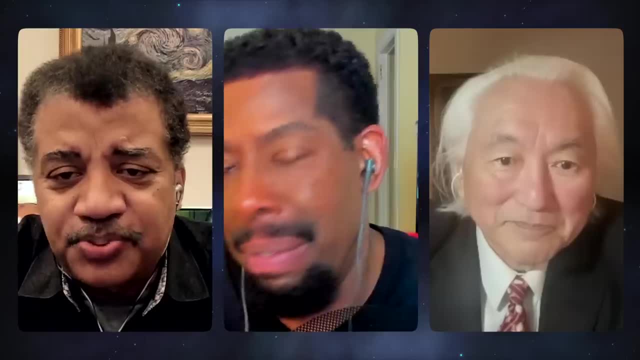 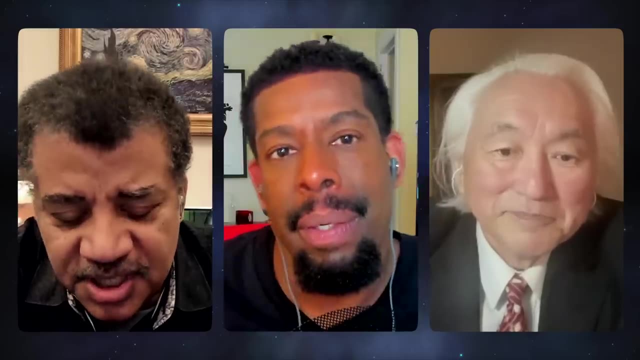 of light between them. I like that Transporter, Transporter, Yeah, Beam your brain, Yeah, Yeah, Yeah, I think that's a great question. I think that's a great question Because I think that's a great question. 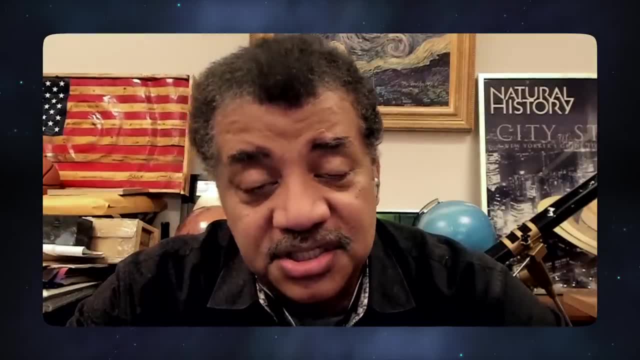 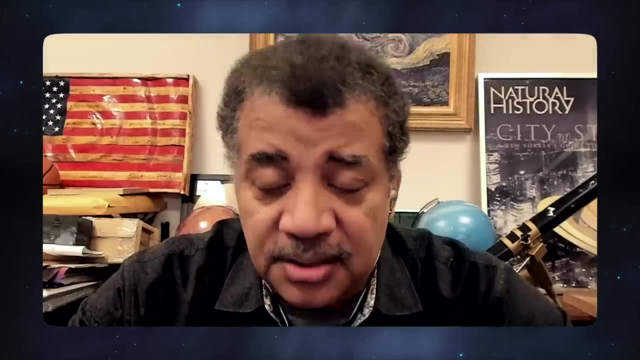 There's so many complexities of the brain and how many neurosynaptic combinations there are, And that's always been kind of an intractable problem. This question suggests, via a question, that the power of quantum computing can simply map our brain with perfect precision. 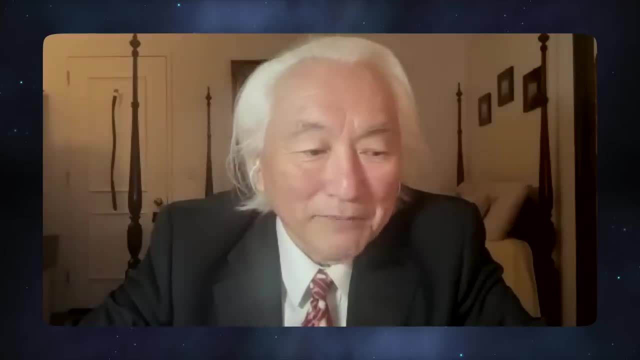 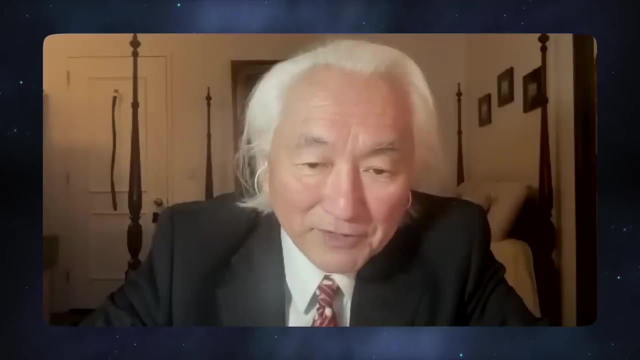 Is that in the future? Well, there is a program to digitize the brain and there is a program to map all the neurons of the brain. Uh-oh, We're at the level of a mosquito. We now know that the mosquito brain has 100,000 neurons. 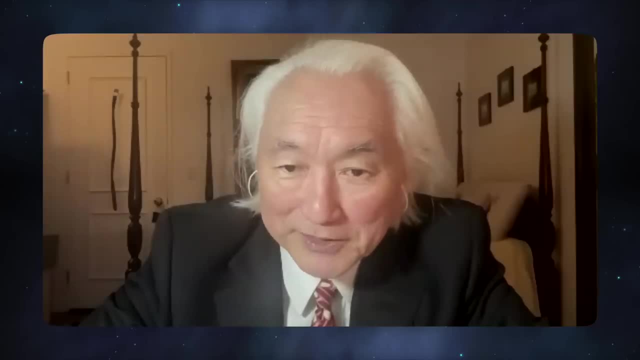 Every single one has been mapped And you can Google it and see what an insect's brain looks like at the level of neurons: 100,000 neurons in the brain of a mosquito. And then, of course, we're going to go up the scale. 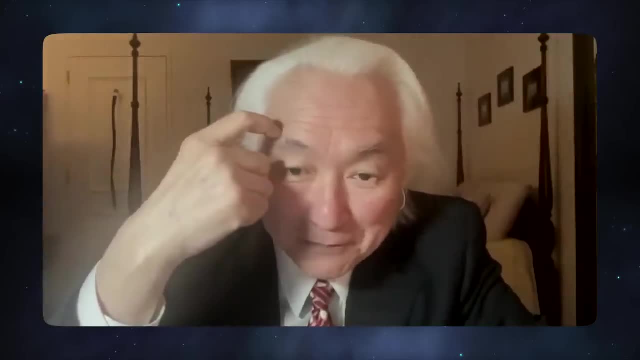 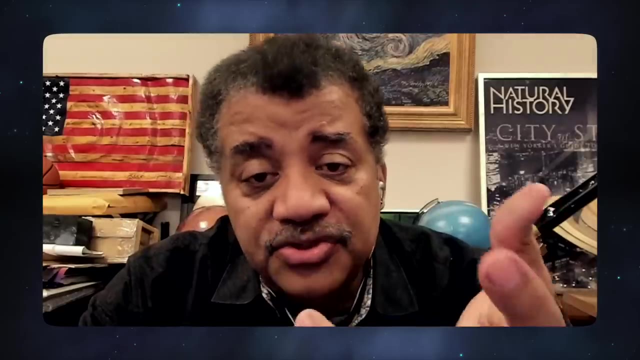 It's going to take time. We have 100 billion neurons in our brain- Wait, wait. So that number is not what's impressive. What's impressive is the number of neurons. What's impressive is the number of connections those neurons can make. 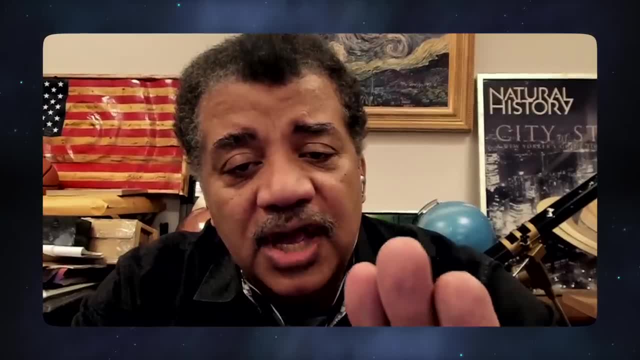 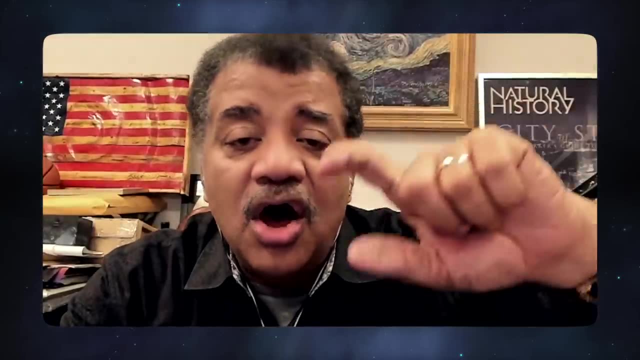 10,000. And that's what you ultimately have. Wait, in a mosquito, how many neurons are there? Approximately 100,000.. And so now the total combinations of total ways those 100,000 neurons can connect, that's. 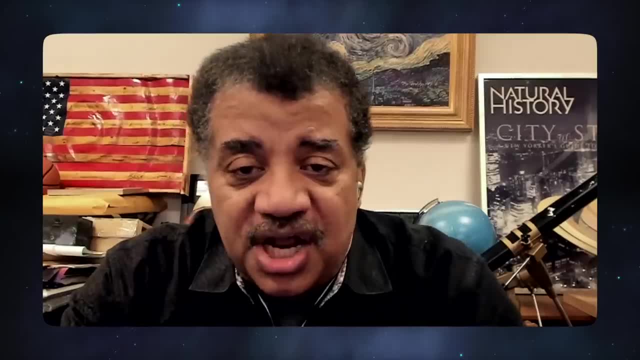 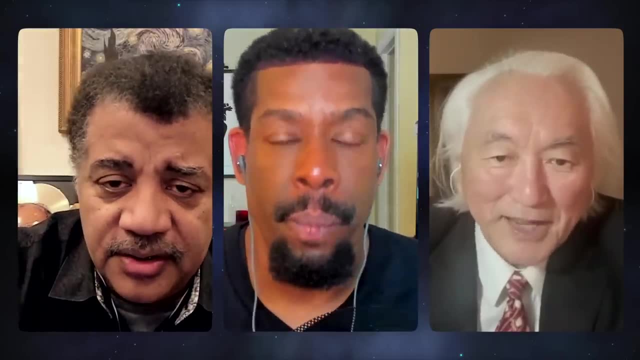 a huge number, correct, Right, Okay. So that's where the computing challenge is not simply that there's 100,000 neurons. right, Right, right. The connection is everything Right. It's the connections that separate us from other animals. 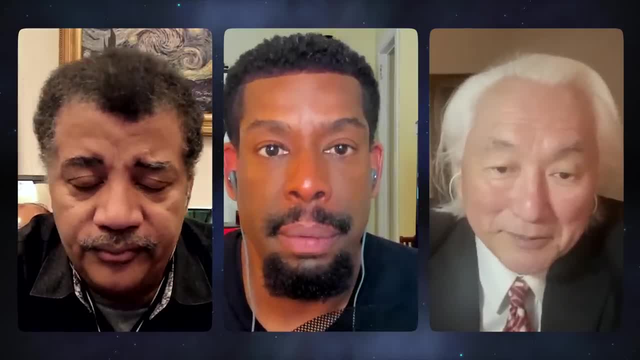 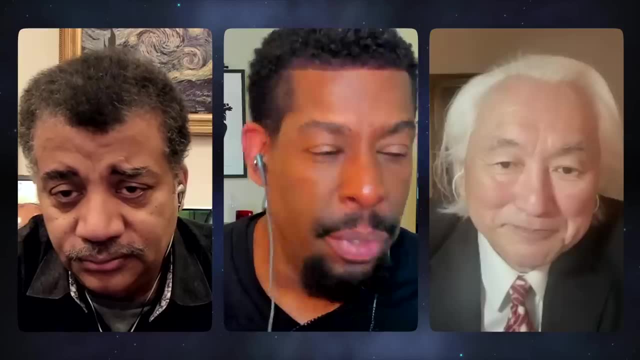 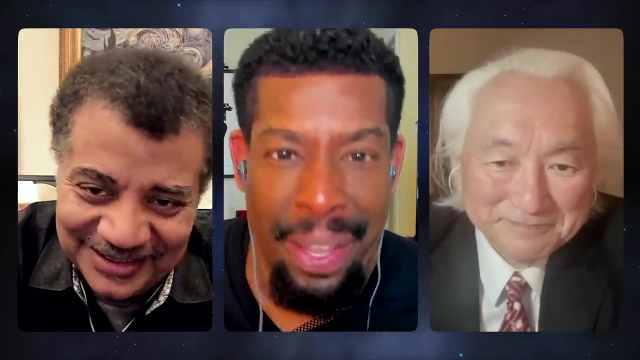 Other animals have brains bigger than ours, for example? Okay, But we have more connections and more ability to do tasks that certain animals do not have. Take that you brig-bane dummies. There you go, You idiot dolphins With your big brains and your stupid self. Stop. No, But you see, a quantum computer has enough computer power to begin to model these things. A digital computer would go berserk counting how many connections you can have within the human brain. But that's exactly where quantum computers excel, because we're talking about the states. 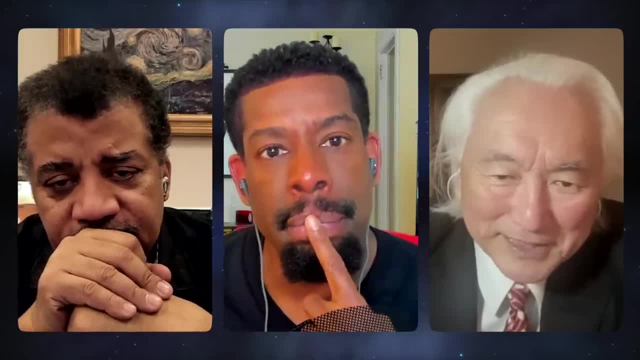 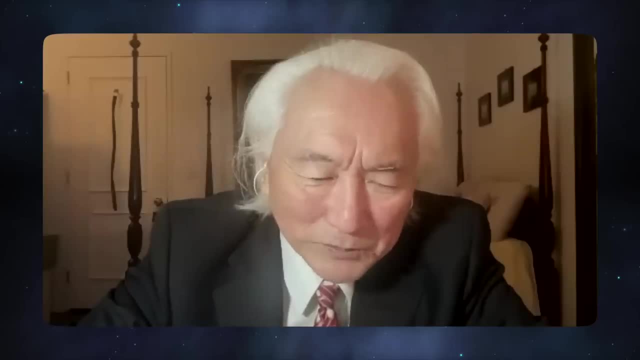 of an atom. How many states of an atom are there? Infinite number of states of an atom For every atom, Mm-hmm. Not that zeros and ones. zeros and ones are binary, which is finite. That's the difference between quantum computers and regular digital computers. 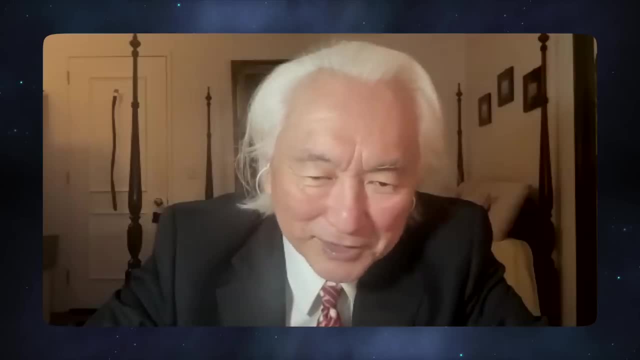 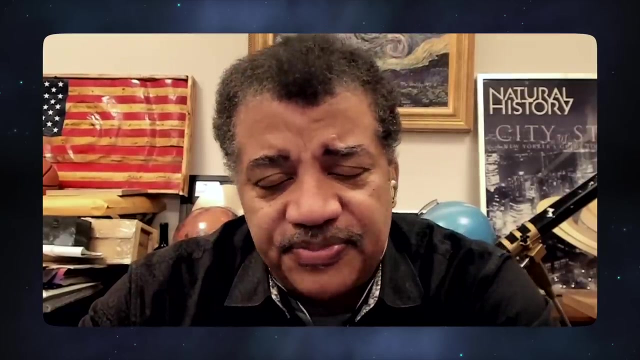 Quantum computers compute on a finite number of objects- zeros and ones- While the quantum computer computes on simultaneously, an infinite number of positions of electrons, In other words, computing on parallel universes. So give us a timeframe. When do you think we can map the human brain and know every neuro-synaptic connection? 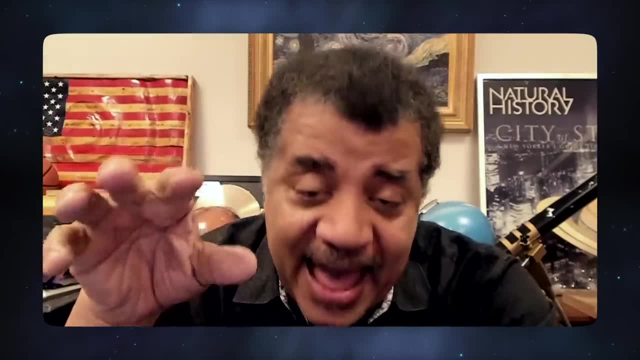 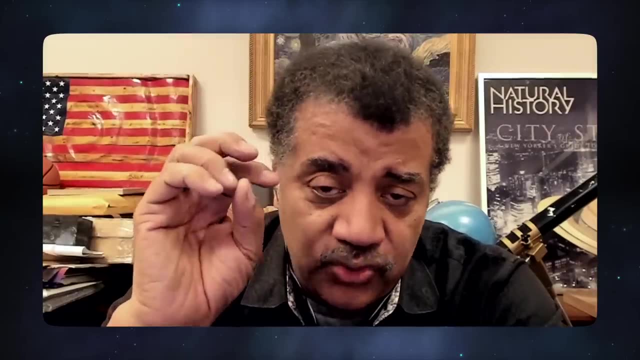 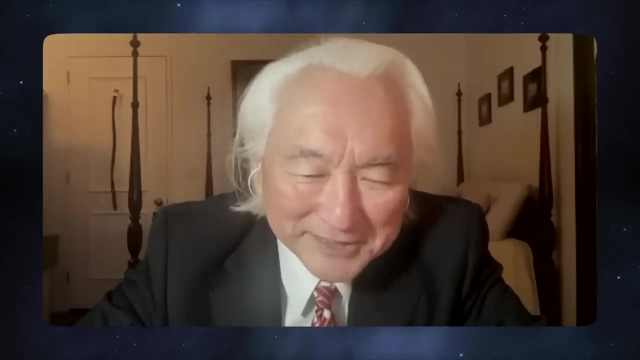 And the day we do, can you just beam that map to another place, thereby beaming your consciousness, Or at least everything stored in your mind in that moment it was mapped? Well, I think it would probably take a few more decades before we can map every single. 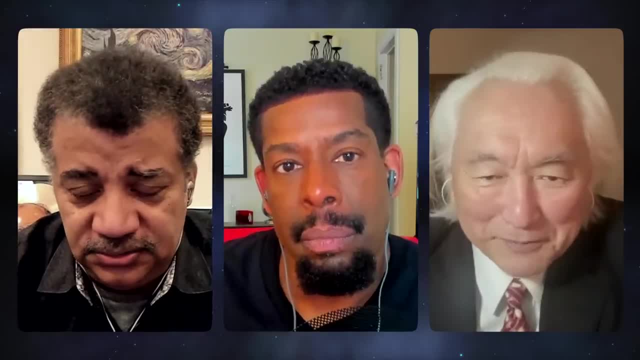 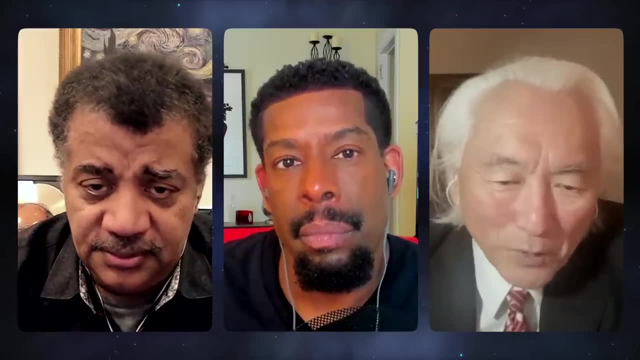 neuron of the human brain, Because there's a hundred billion neurons, each neuron connected to 10,000 of the neurons in the human brain. It would take a while, But once it's done, then the quantum computer can easily begin to manipulate it and fire. 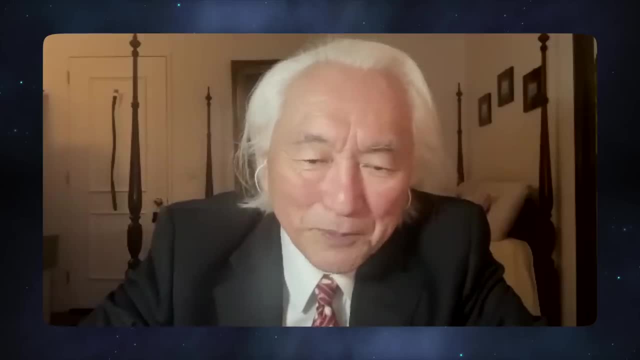 away and create certain thoughts. okay, So the problem is not the quantum computer. The quantum computer has more than enough power to model the human brain. The problem is to slice up the human brain, slice and dice the human brain so that we get all the connections of the human brain mapped. 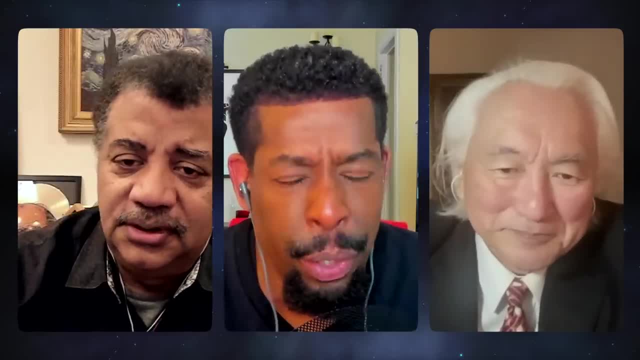 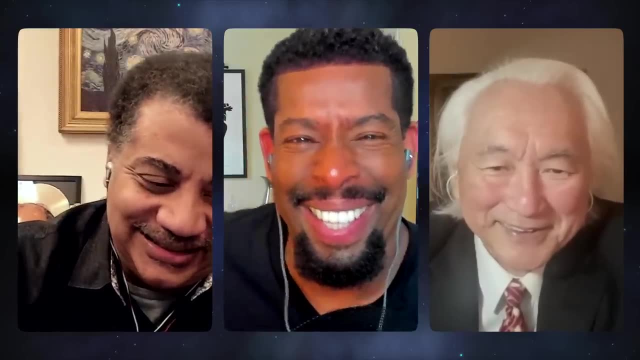 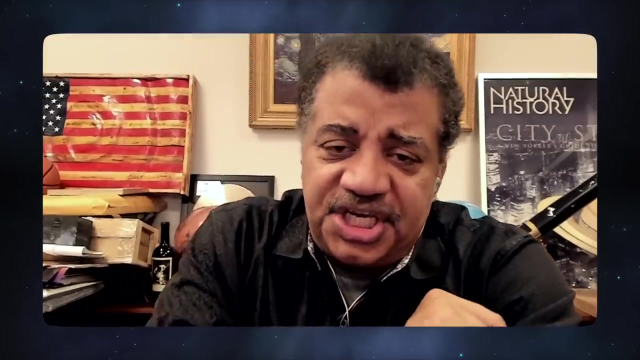 That's what takes time, That's labor intensive. So what we're lacking are volunteers. That's really the problem here. Brain volunteers- Yeah, that's right, All right, So it's still a little while before that happens, But the day it does happen, do you foresee being able to beam an entire person's Is? 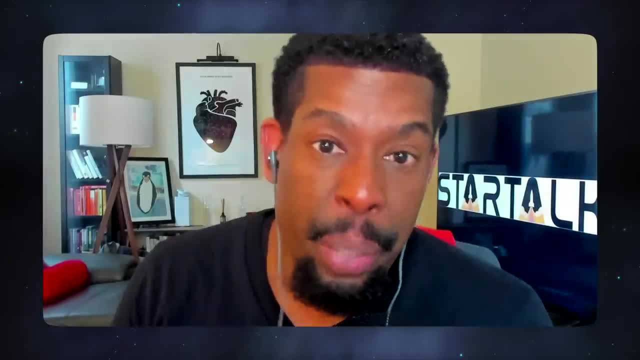 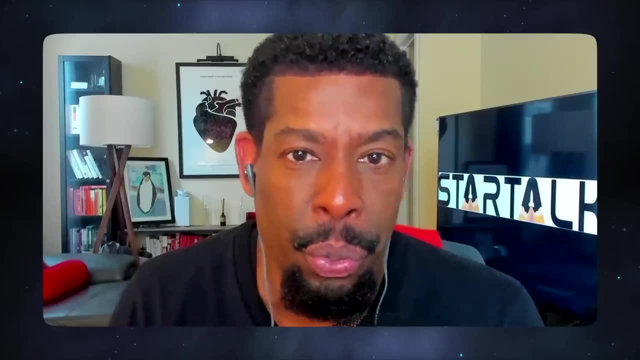 that the same as beaming their consciousness, Just knowing how everything connects. At that point the quantum computer would have to locate consciousness within the brain. But once you do that, why wouldn't you be able to recreate it, download it or manipulate? 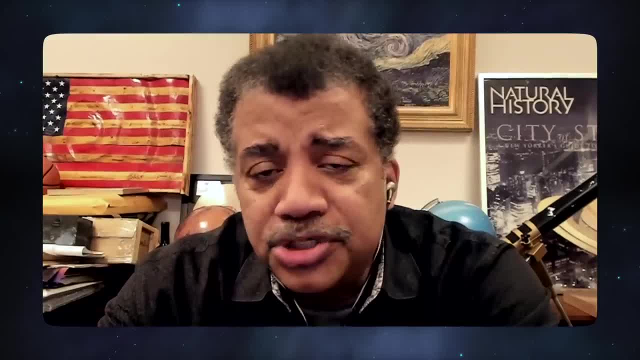 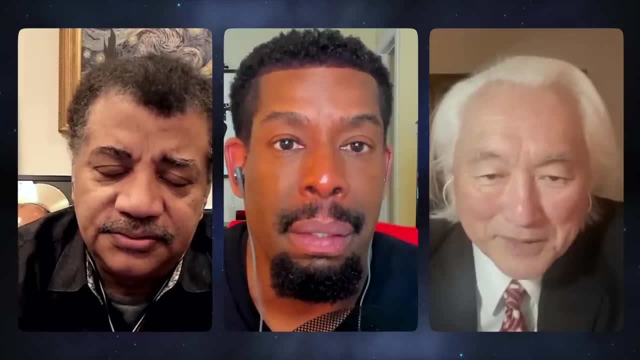 it. And maybe consciousness is not a thing in the brain, Right? Maybe it's an emergent feature brought forth because of all of those connections? Yeah, Right, So you're saying that it is emergent? There's no one quantity that you can put into a computer. 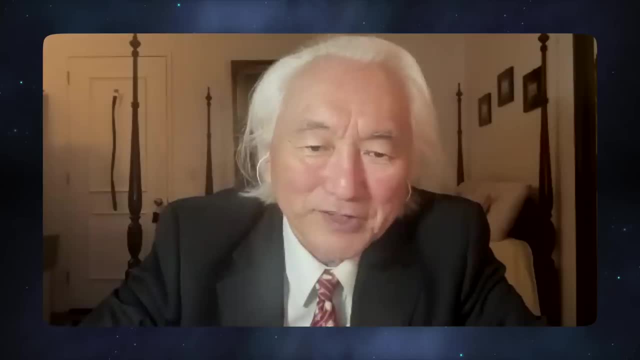 It emerges naturally as a consequence of all the neural connections. Consciousness emerges just as a byproduct of hooking up everything. You plug it in and it becomes conscious. basically, Love that. Okay, Next one, Chuck, Keep it going. 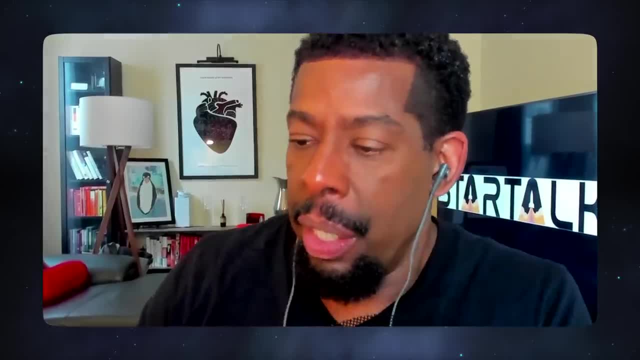 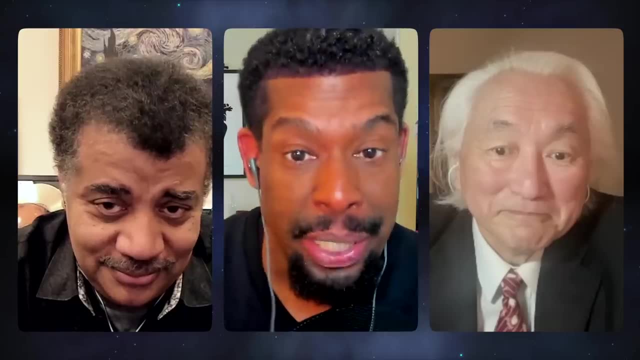 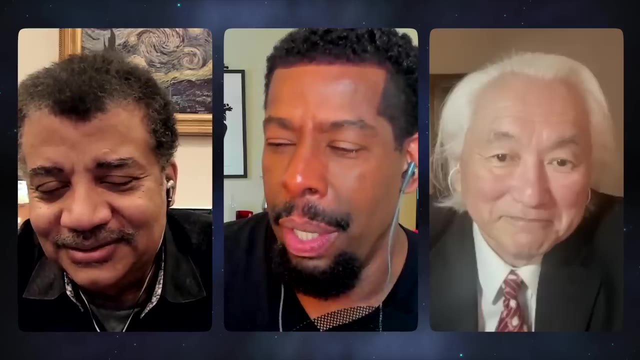 Okay, Here we go, Let's keep going. This is Chris Trent, And Chris says hi. I have heard Michio Kaku say That his day job is actually string theory. I have always wondered when he shows up at the office, gets his coffee and gets to work. 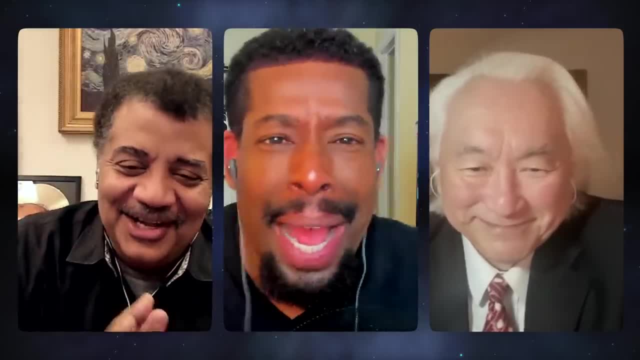 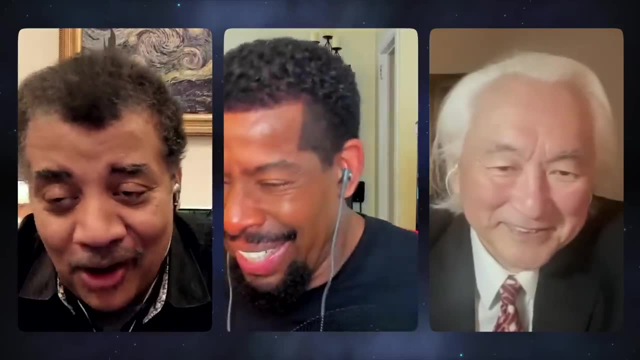 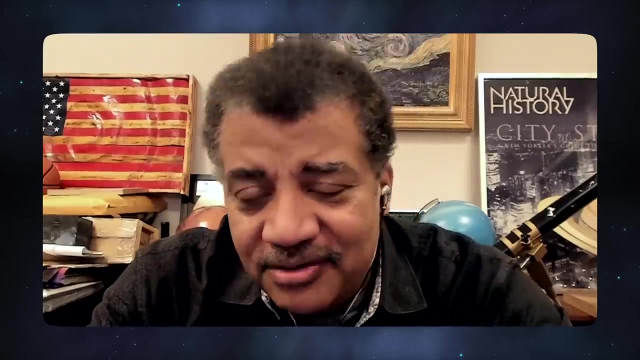 what exactly does he do? How does one work on string theory? Yeah, Michio, is there anything on your desk at all? Is there a pad and paper? See, so, Chuck, I've always joked that string theorists, they're really cheap. 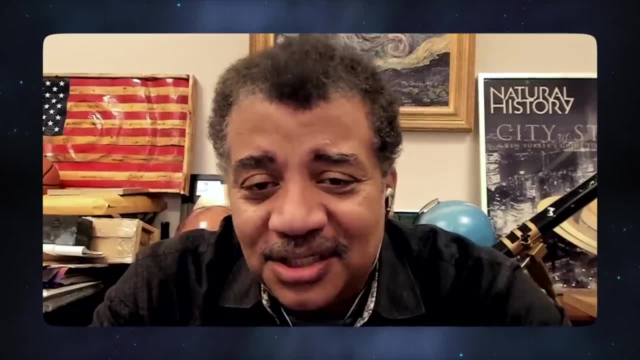 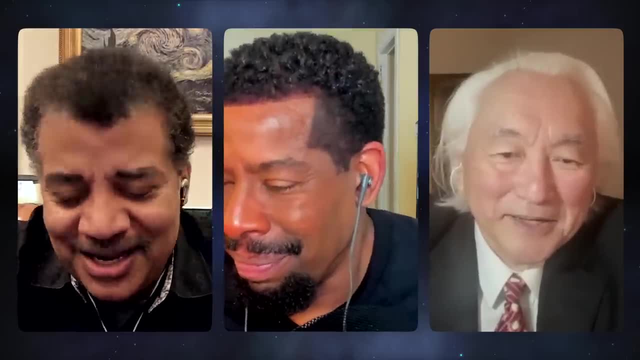 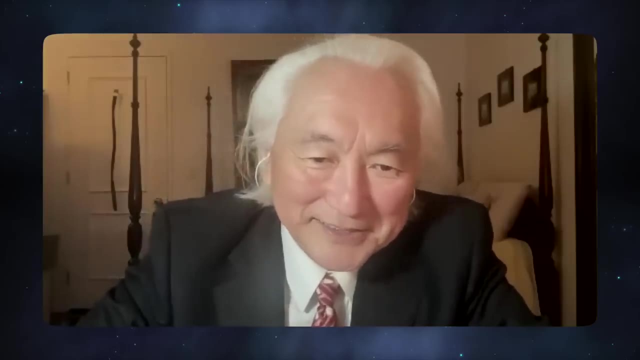 Right. Give them a laptop, maybe a pad and a pencil, and just give them a room, and they're good to go. They're good to go. So, Michio, have we completely characterized you professionally? Well, when I was in the Army back in 1968 as a GI, I used to- I read the first articles: 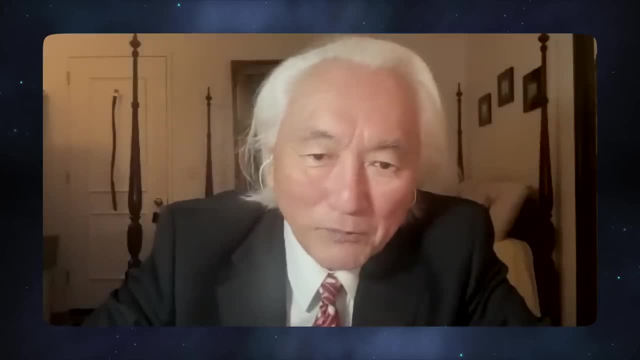 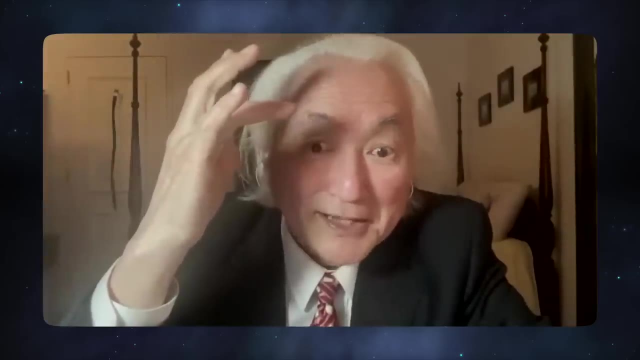 on string theory and I began to play with it when I was doing basic training. So, dodging machine gun fire, I would imagine twisting strings in my mind And so, in other words, it's very visual. These are real strings, like violin strings. 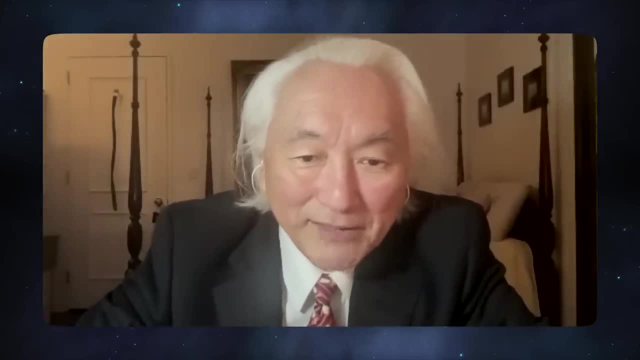 You can turn them around, twist them, make knots out of them or whatever. And that's what I would do when I was in the military. After I got out of the military, I would write up the papers, okay, And I would create something called string field theory. 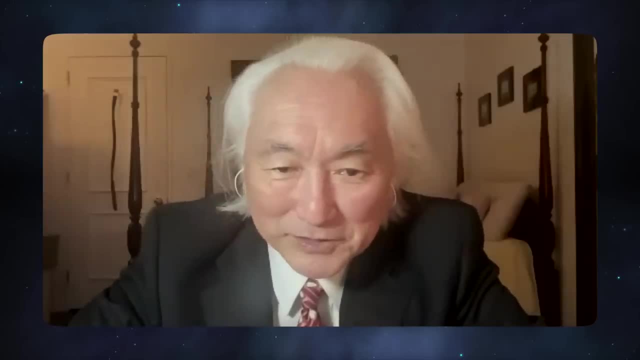 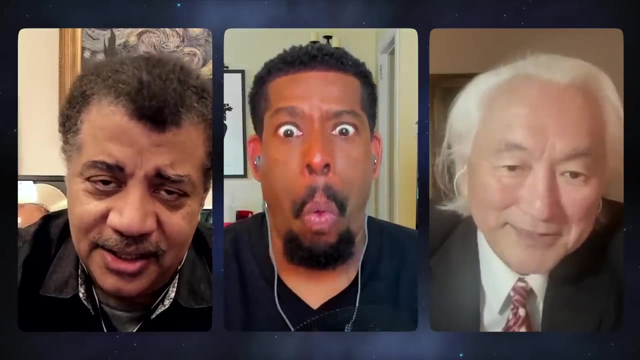 The field theory of strings, Just like Maxwell's equations. there's the field theory of electricity and magnetism. Aren't you the father of that whole branch of physics? Is that correct? Exactly, Okay, That's right. Wow, Uh-huh. 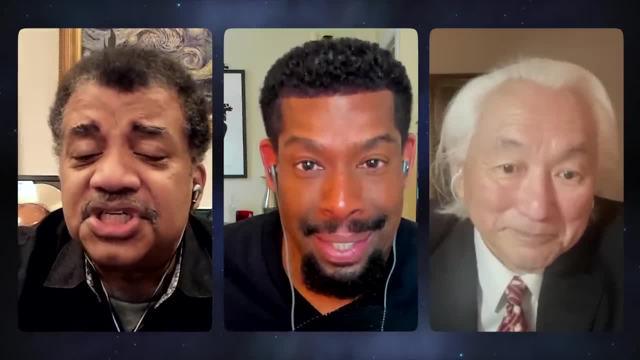 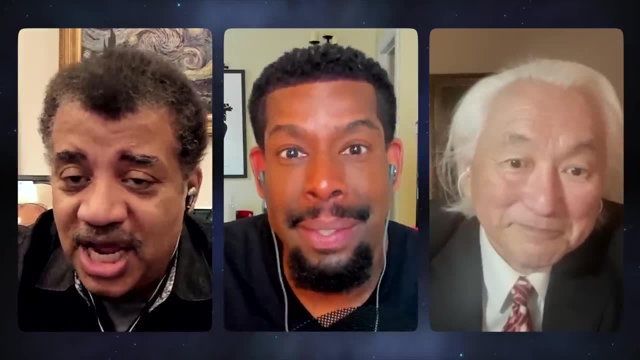 So, Chuck, you see, he must have known something in the. Did you hear what he said? He said as I was dodging machine gun bullets. Machine gun bullets, Right See. So he's got some extra access to higher dimensions there, because the bullets were not hitting. 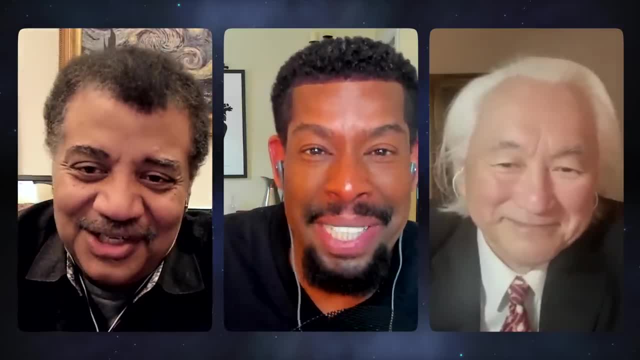 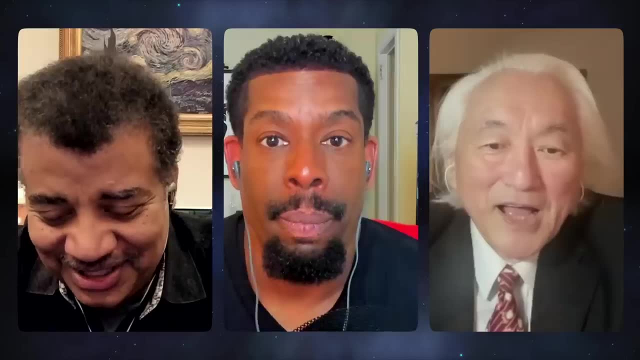 them. You were phasing in and out of this dimension, Exactly So, Michio, you're at your desk and now what? You sharpen your pencil Right And I go through hundreds of pages, I go through hundreds of calculations. 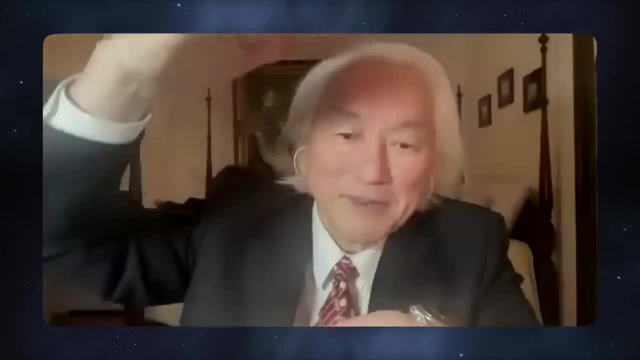 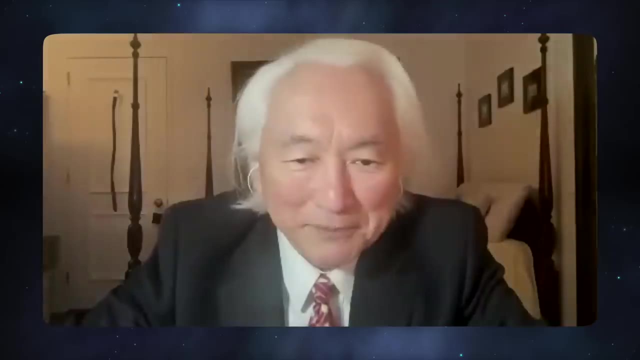 This is tensor calculus, supersymmetric tensor calculus. On my desk is a pile of paper, Each paper basically filled of chicken scratches, because it takes a lot of brain power to be able to write down all the equations. because these are resonances. 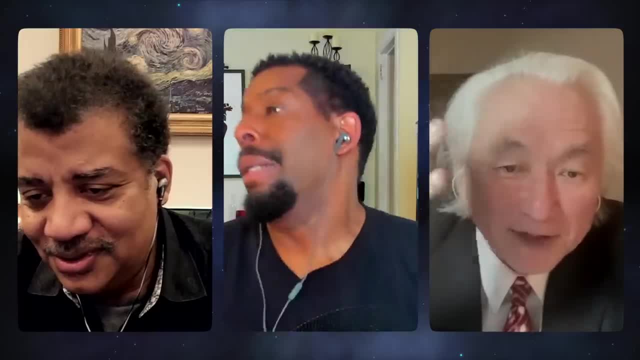 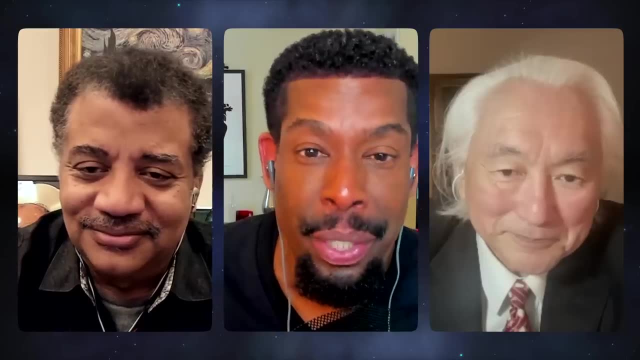 Resonances of strings vibrating in 11-dimensional hyperspace, And so it takes a lot of paper to do that. Dang Go on. I mean, can you just say that again? I want to get a t-shirt that says that. 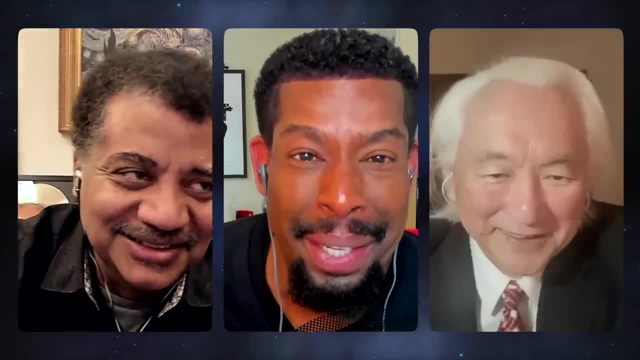 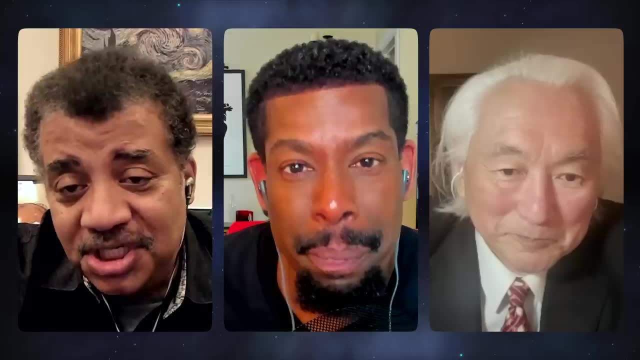 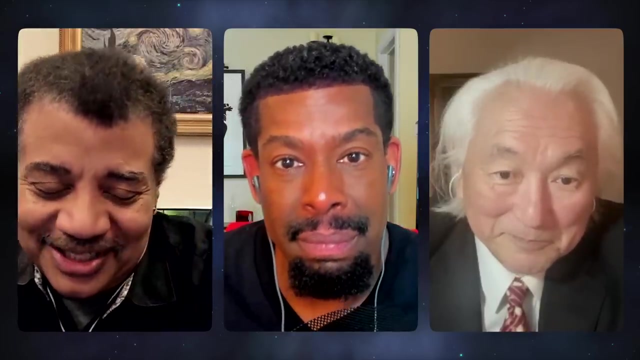 Wait. So now combine that with when Michio was in the army. He just slipped it out that he was dodging machine gun bullets. So last I saw that was in The Matrix, where Morpheus is teaching Neo how to be badass. 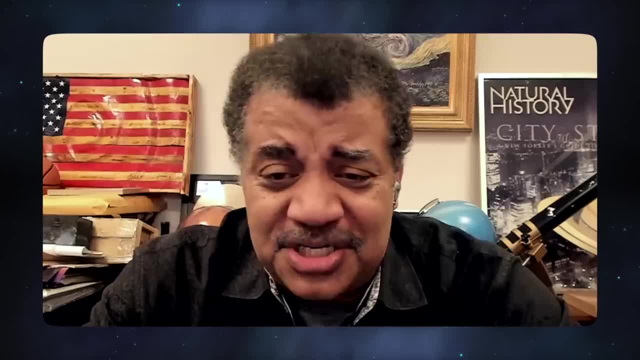 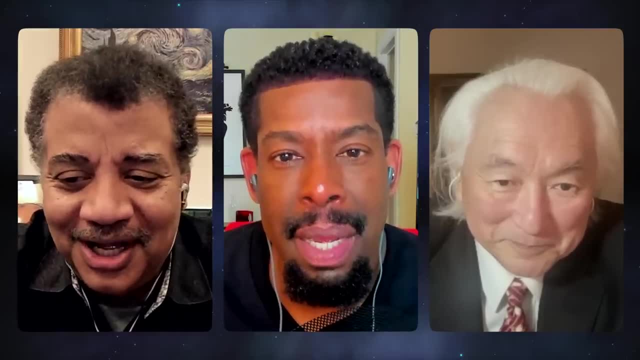 and Neo's saying: you mean, one day I'm going to be able to dodge bullets. And Morpheus says, Neo, when that day arrives, Yeah, You won't have to. Ah, Yes, Oh. And then he's like: what does that mean? 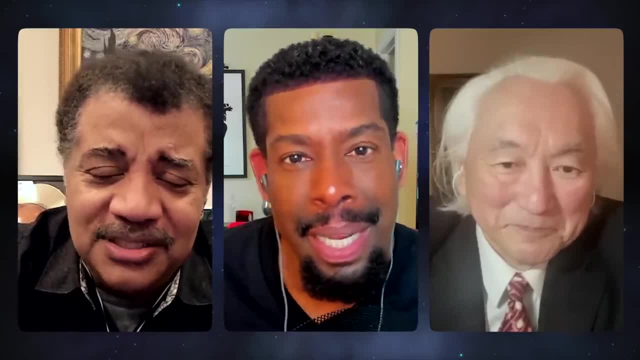 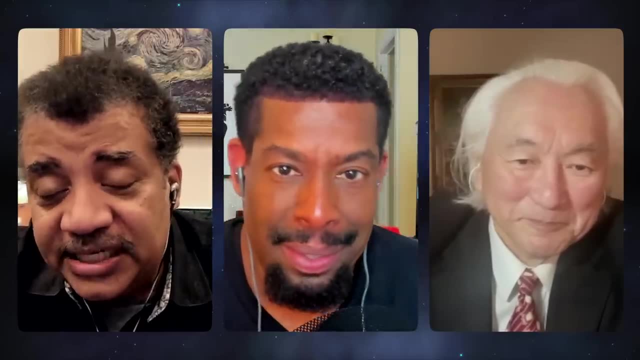 You don't have to dodge them, And my boy just stopped the bullets in midair And that's what happened. Yes, There it is. I'm not even going to duck, I'm just going to stop. So I think Michio has those powers and he just leaked it on this show. 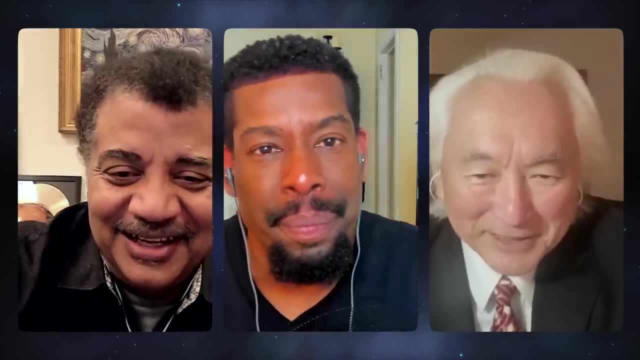 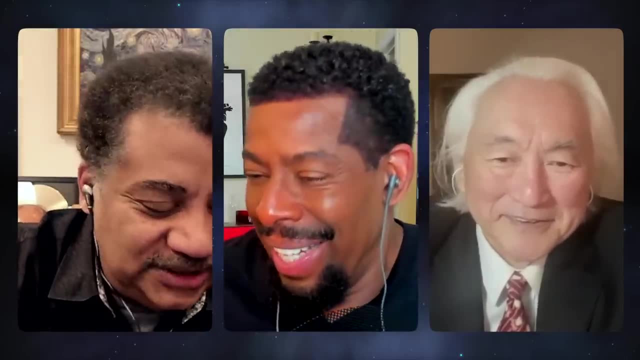 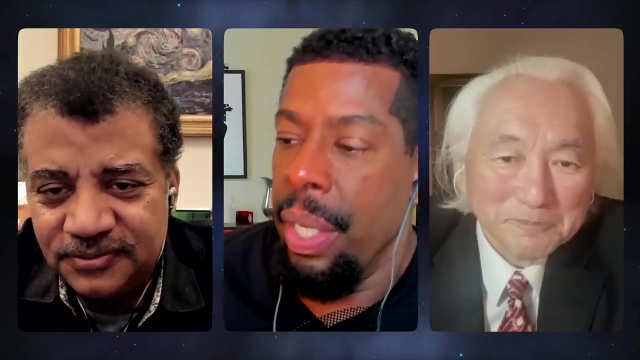 Just now, Nice. I just want to demonstrate it: No free demonstration, No free demonstration. That's right, There you go. All right, Excellent, Keep going, Check Okay, Here we go, Here we go. This is Chris Henderson, and Chris says-: 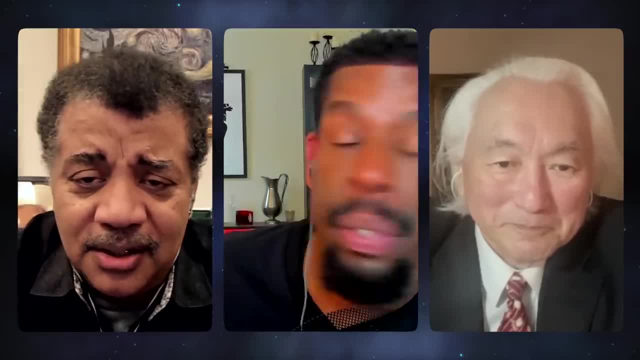 Do we know where they're from? Don't they say where they're from, Or are you skipping that They do? No, they don't, They don't. Okay, If they say where they're from, I let you know. 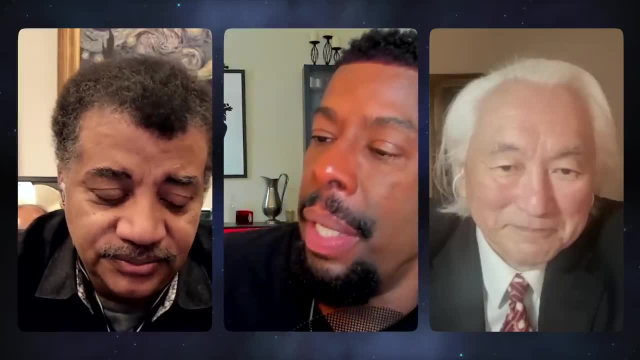 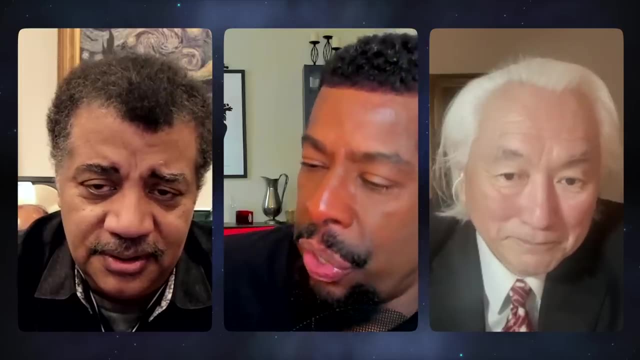 I like knowing where they're from. Okay, Go on. Or sometimes they'll put it in the body of the question. Yeah, Hello Dr Tyson, Hello Dr Kaku. This is or is it theoretically possible to make communications that uses quantum entanglement? 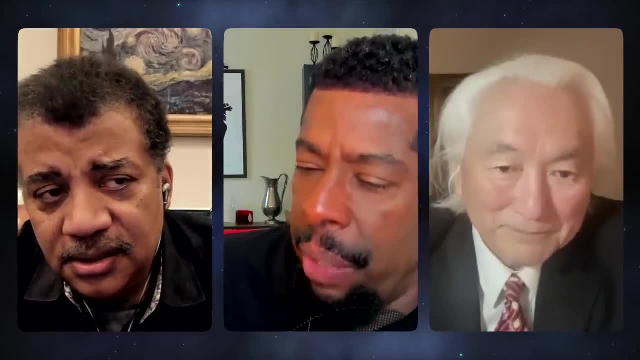 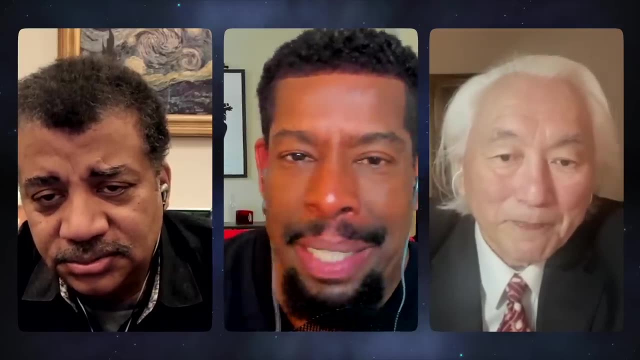 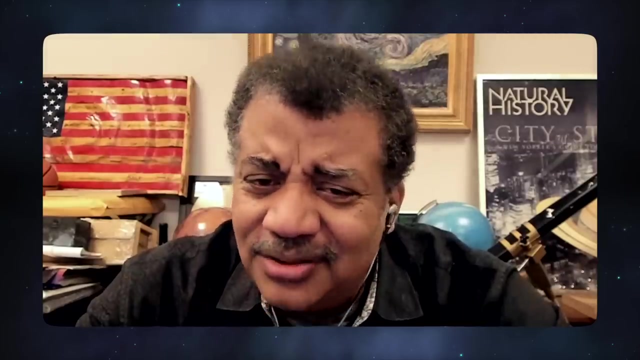 Ooh, If it is. If it is, would this give us the ability for instantaneous communication with distant spacecraft? So he's talking about subspace communications, A subspace network. yeah, And Michio, adding to that, I read, because I only know from what I read, right about. 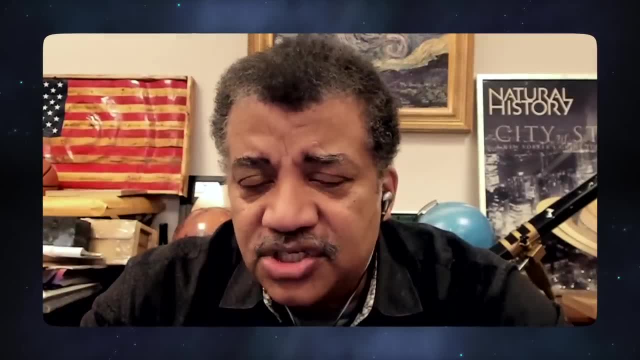 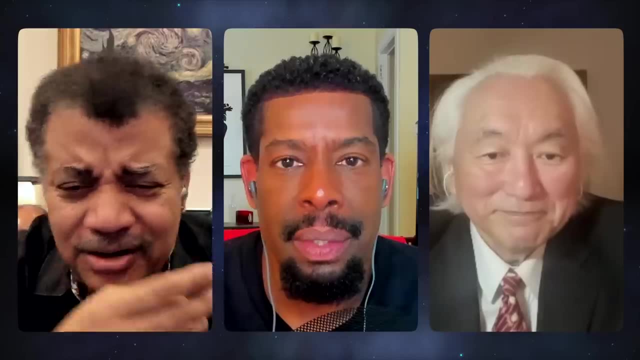 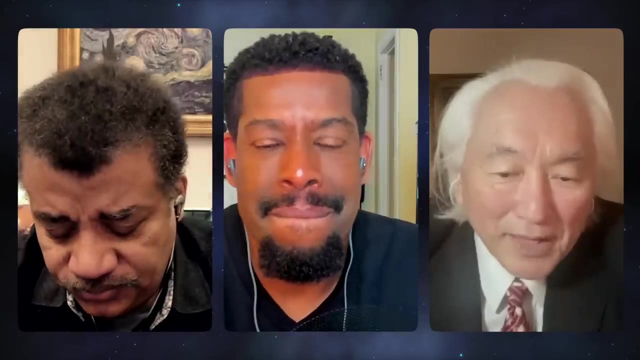 quantum computing. that isn't the circuitry of quantum computing, exploiting quantum entanglement between adjacent particles in the circuit board. I heard something about that. I heard something about that. So how does quantum entanglement fit into quantum computing? Well, yeah. 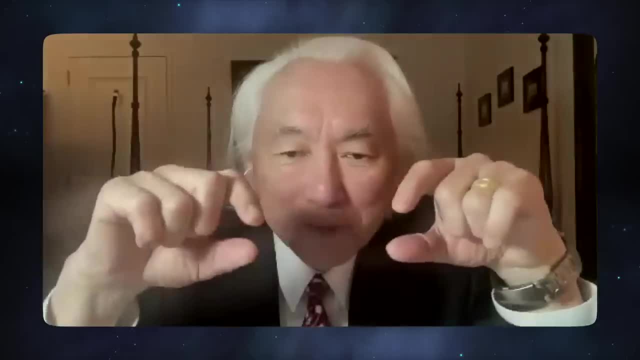 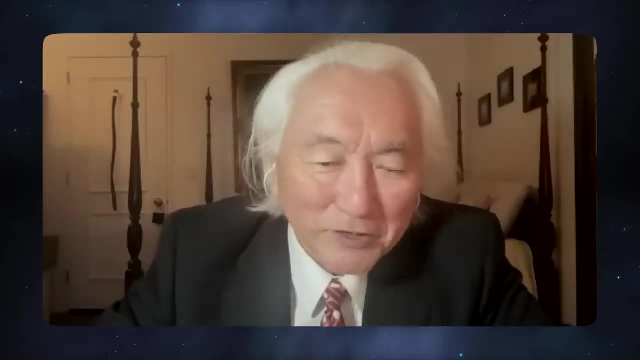 Quantum entanglement is one way in which these qubits can communicate with each other. Now you know that in a digital computer the bits do not talk to each other. Zeros do not talk to one. One does not talk to zero. 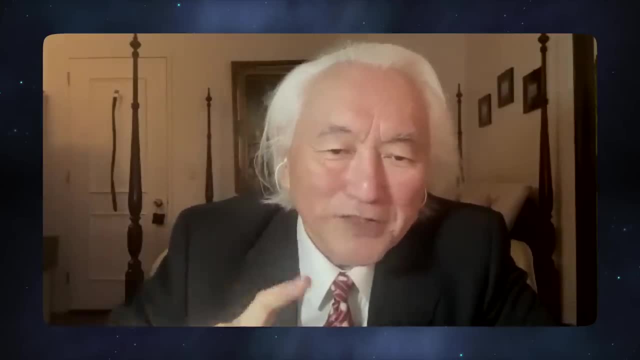 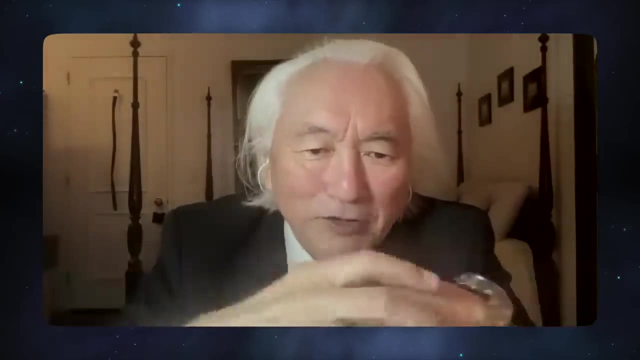 They are independent when you do a calculation, Not so the atom. If I have two atoms close together and I jiggle one atom, the other atom responds, The other atom responds to it. This is called entanglement. And the question is: well, that's one reason why quantum computers are so powerful. 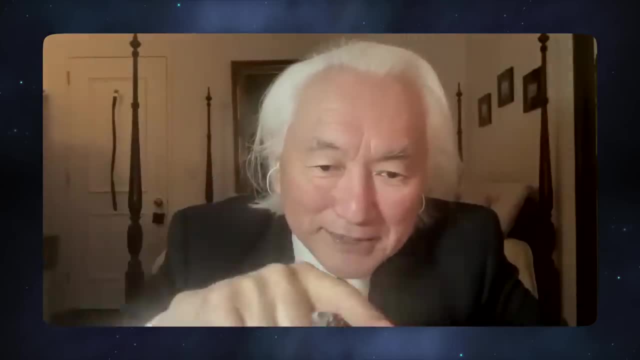 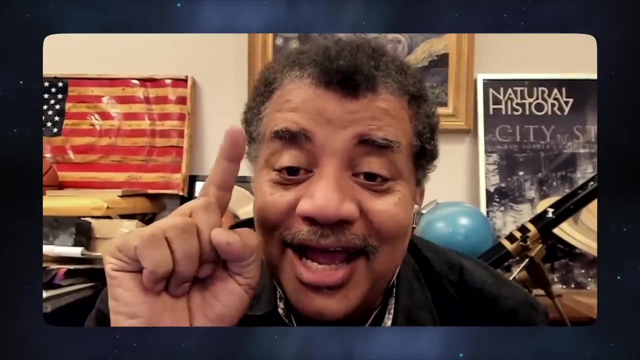 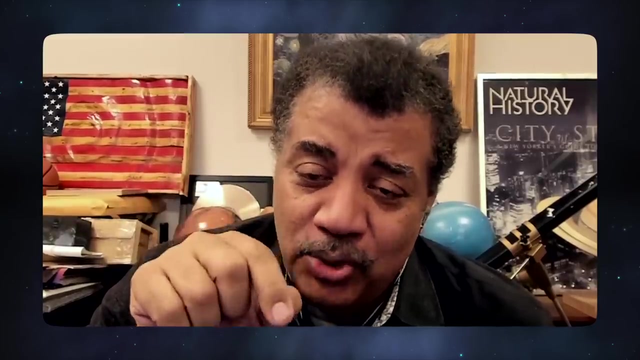 All the different kinds of qubits talk to each other simultaneously. Then the other question is: do they talk to each other faster than the speed of light? Let's take a break there and leave everyone dangling on a cliff edge about whether we are communicating on a circuit board faster than the speed of light. 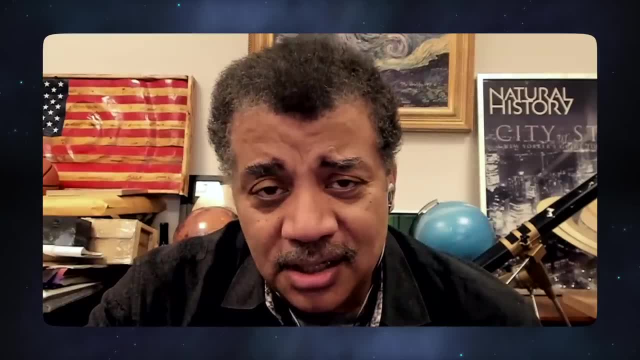 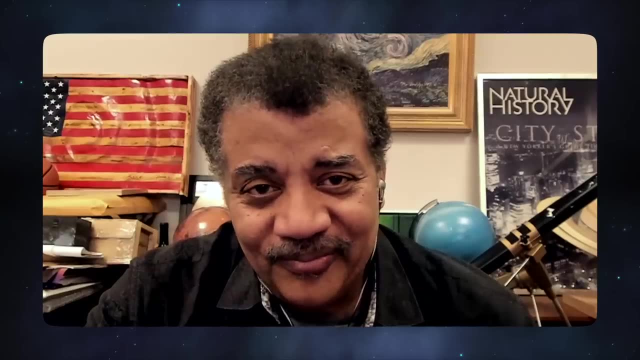 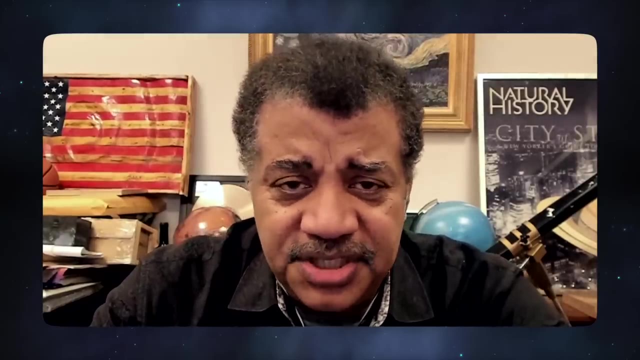 We're going to take our second of two breaks Here at StarTalk, where it's Cosmic Queries, with my good friend and colleague, Michio Kaku. We'll be right back. We're back. Third and final segment: Cosmic Queries- StarTalk with my friend and colleague, Michio Kaku. 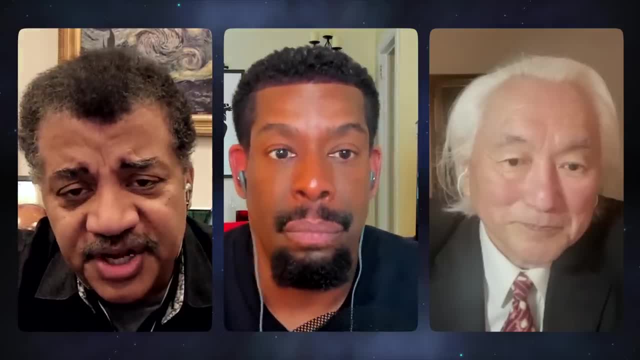 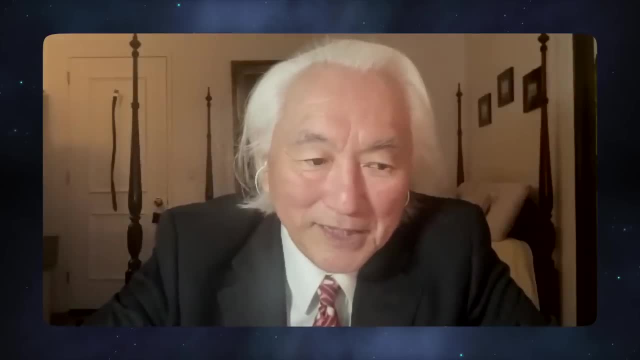 Michio, tell us about your social media footprint. How can we find you? Go to mkakuorg M-K-A-K-U dot O-R-G. I have about five million fans on Facebook and the Internet. I'm definitely on the Internet. 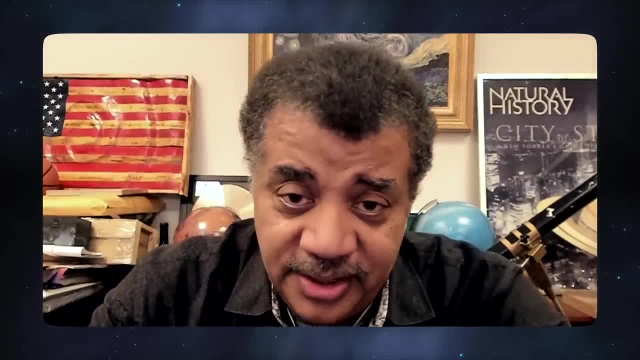 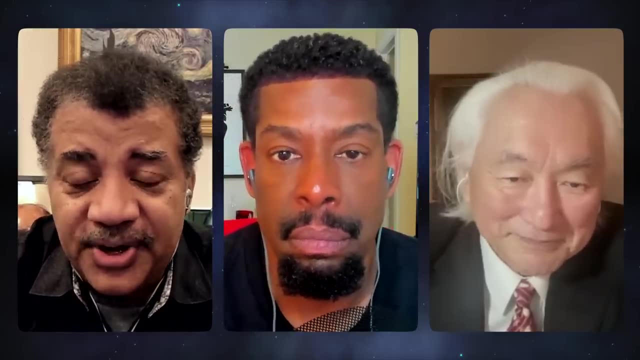 You're totally on Twitter, right? You're active on Twitter. I follow you on Twitter. I know where you're coming and where you're going. Okay, that's what we can do. Chuck, you left us off with a question about quantum entanglement. 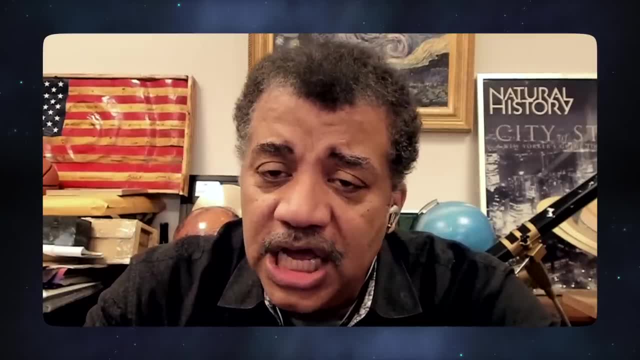 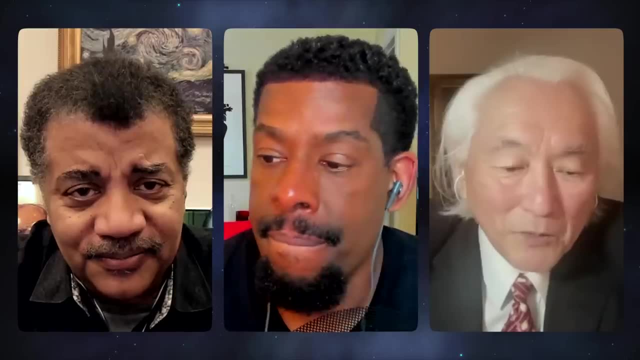 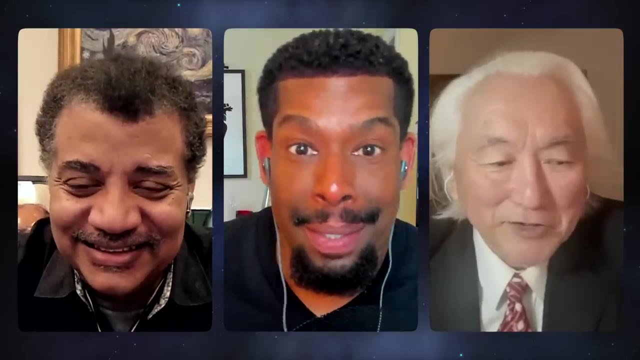 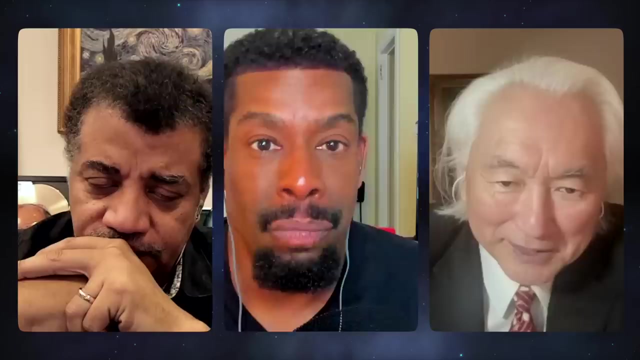 and whether we can use it as a byproduct of quantum computing for instantaneous communication. Michio, what can you tell us there? Well, it turns out that Einstein was wrong on this question. Einstein said that you cannot break the light barrier. It turns out that these qubits will actually communicate with each other instantly, faster than the speed of light. 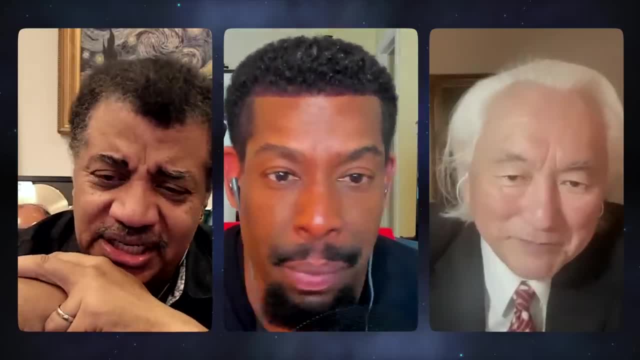 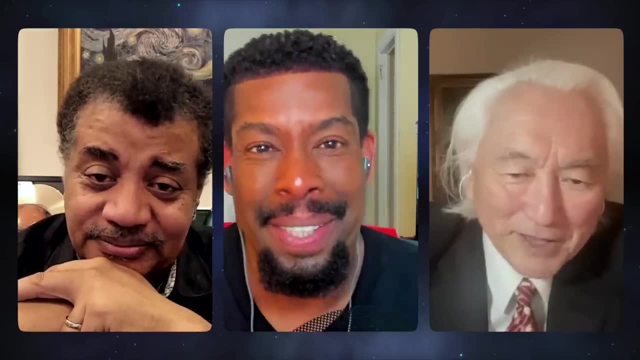 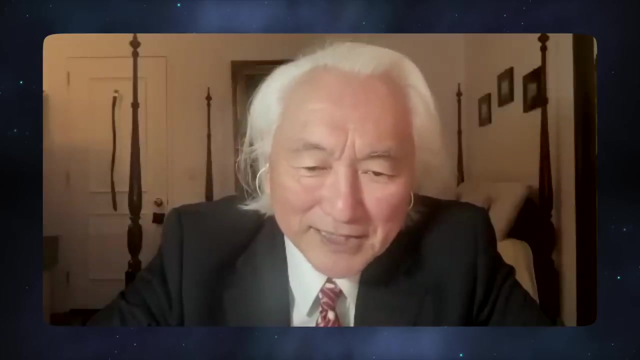 Einstein was such an idiot. I'll tell you what a dumbass That Einstein. Even though Einstein was wrong on that- that some things can go faster than the speed of light- he has the last laugh Because it turns out that what goes faster than the speed of light is nonsense. random information. 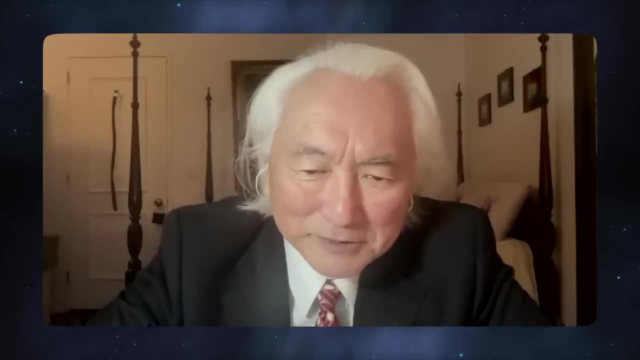 Morse code cannot be sent faster than the speed of light using the EPR effect E for Einstein, And it turns out that we can test this in the laboratory. We can now prove that you cannot break the light barrier for usable information like Morse code. 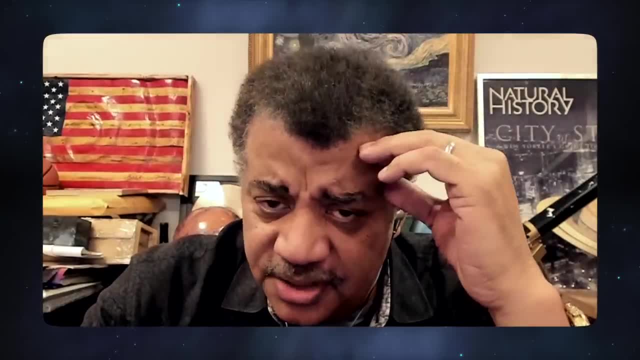 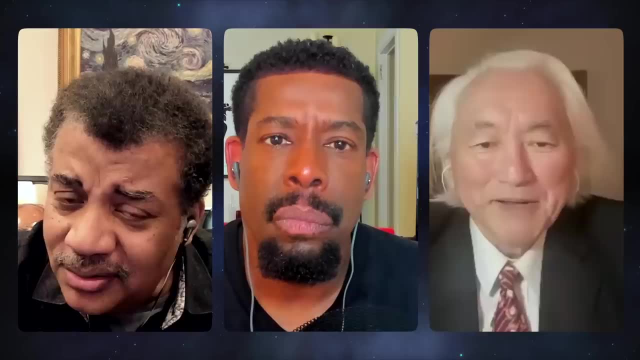 So EPR, Einstein, Podolsky, Rosen, That's right. Effect, That was some experiment that they proposed to test something about quantum physics, That's right. Let's say I have two electrons that are together: One spins up, one spins down. 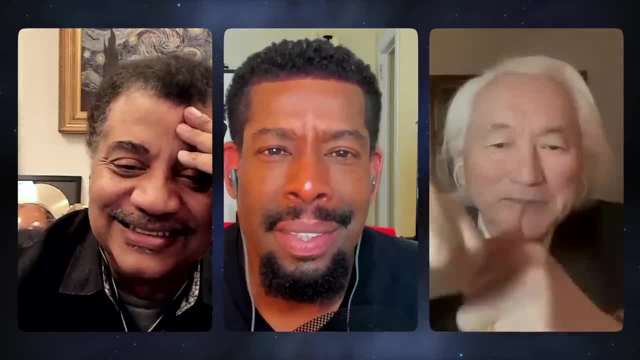 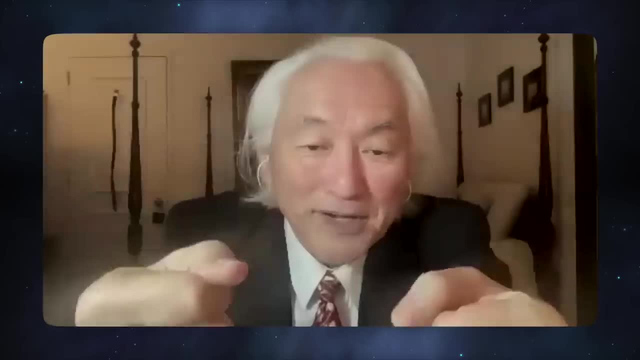 See, he's thumbs there. He's got his thumb there. They are in opposite directions. Okay, Then I separate them. I separate them by a light year. Okay, If one of these is measured to spin up, then the question is, what is the other one spinning? 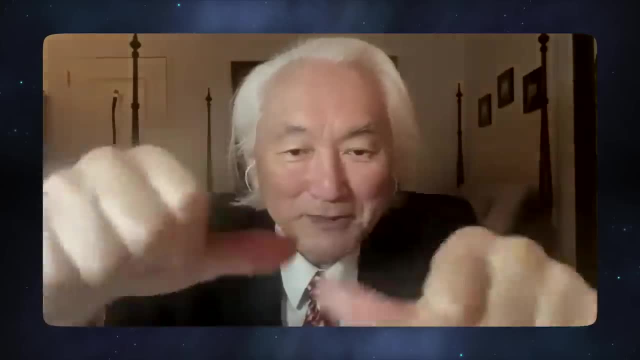 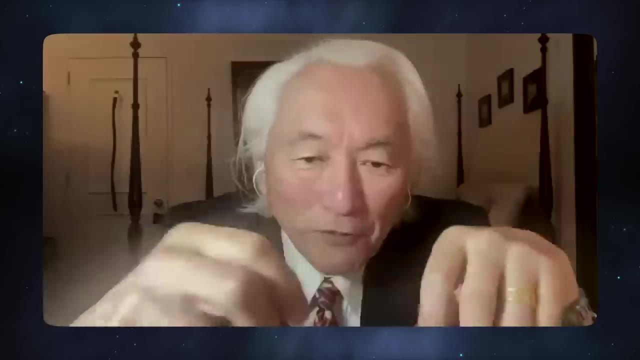 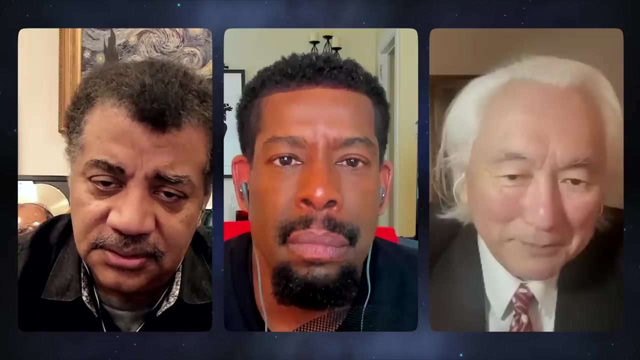 The other one is spinning down because the sum of the two has to be zero. it has to be either like this to cancel out, you have to cancel out like this. okay, but before you open up one of these photon electrons, you don't know what the other one is. but as soon as you know that one is up, the other one, you know the other one's down. 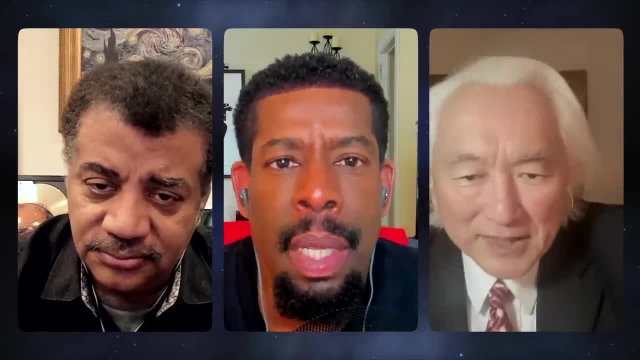 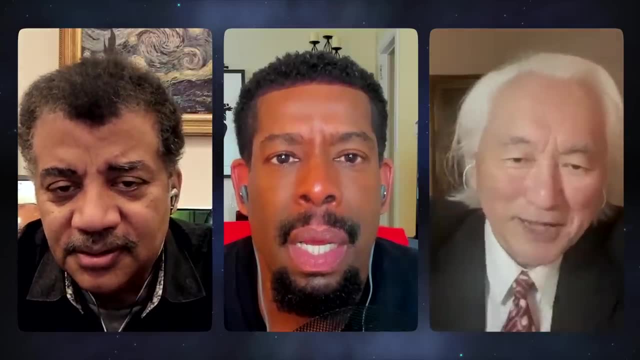 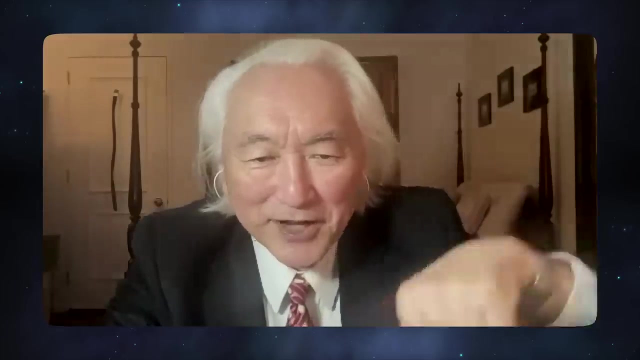 now, how fast did? how fast did you know that instantly, instantly, faster than the speed of light on one side of the milky way galaxy, you know the electron is spinning up. therefore, you know that on the other side of the milky way galaxy, faster than the speed of light, the other. 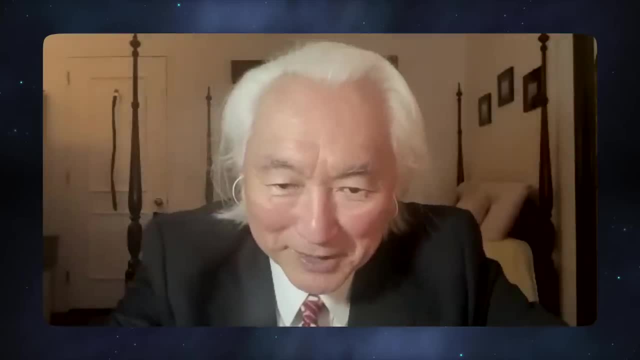 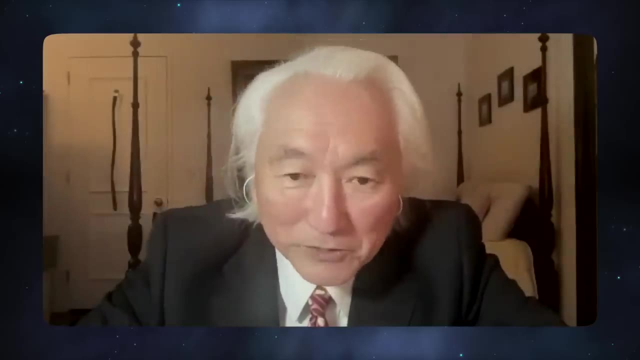 electron spins down. that is the EPR experiment. and Einstein thought: ha, that proves that it's all nonsense. it proves that all quantum theory is wrong. well, we do these experiments now. Einstein was wrong. information travels faster than the speed of light, but it's not usable information. 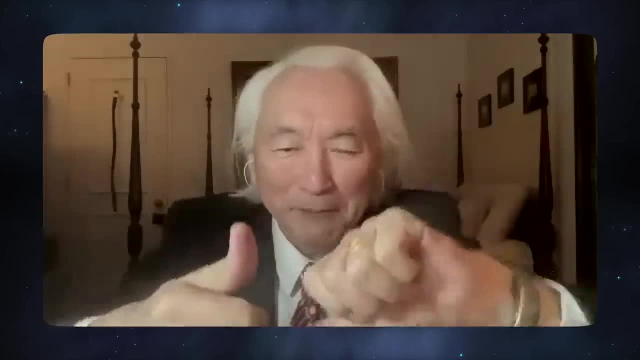 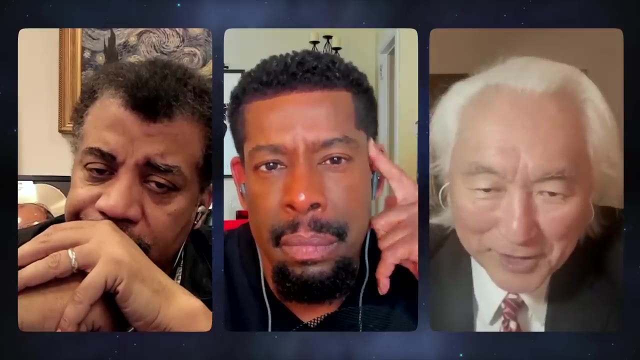 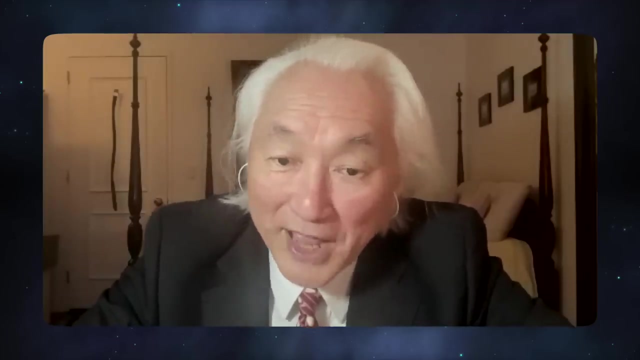 you can't send Morse code this way. Morse code cannot be sent this way. let's say, for example, that you have one sock which is green and one sock which is red. okay, you put the red sock on and the other sock is green. now let's say you open the sock one day and it is red. what? 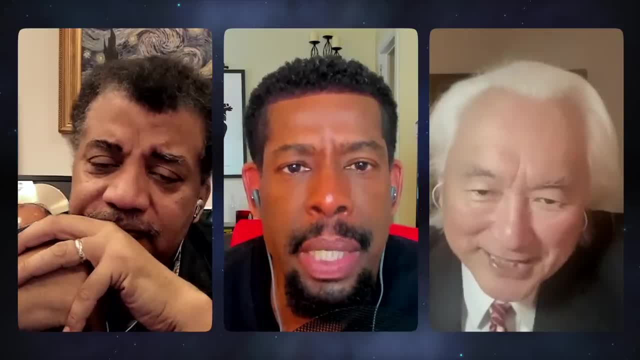 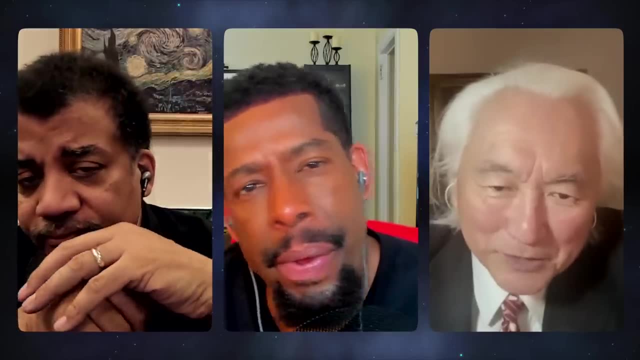 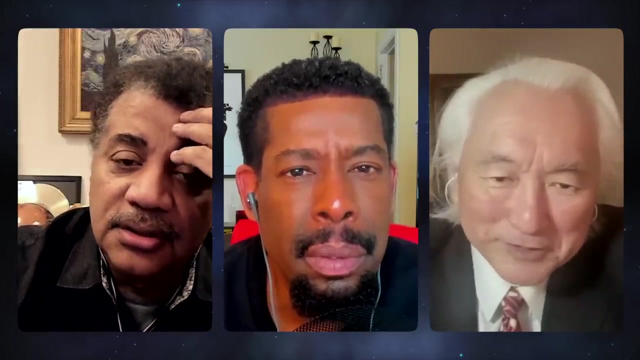 is the color of the other sock? well, it has green. how fast did you know that? instantly, faster than the speed of light. okay, you knew that the other sounds like you're sending information faster than light. so, but you see, it's not usable. you can't send Morse code this way. Morse code cannot be sent using socks. why not? I mean think. 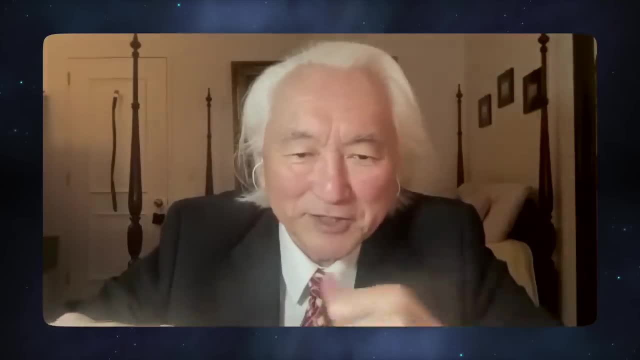 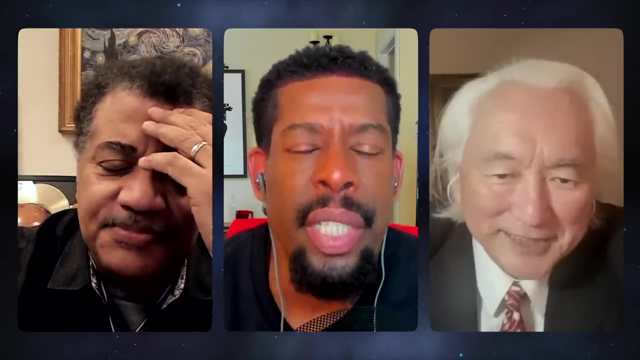 about it for a moment, because as soon as you know that one sock is red, the other sock is green. but where did where did the message go? there's no message there. you're not saying that, you're saying. you're saying you're saying that the message is fixed. therefore, it's not usable. 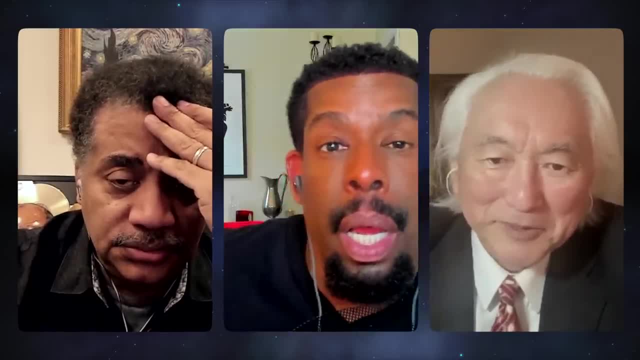 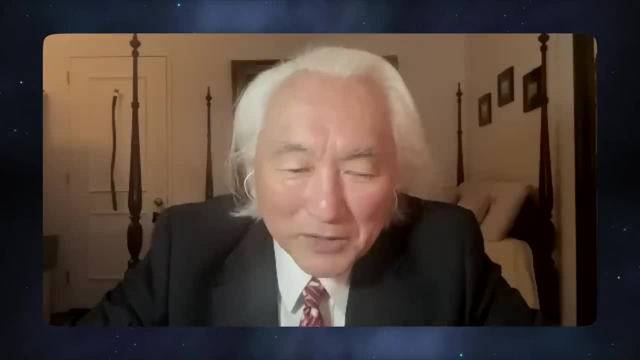 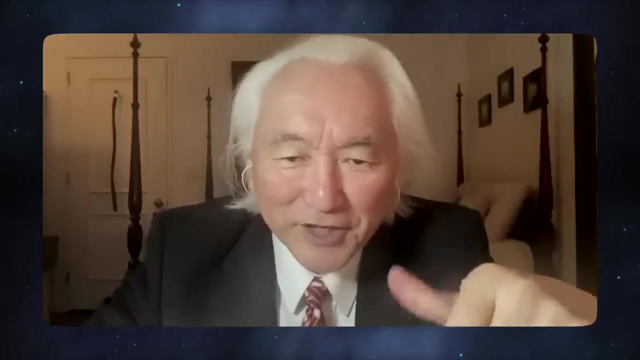 oh no, it's random. it's random and therefore not usable. okay so, but it's. but it's random, even though you know the outcome. oh well, you don't know the outcome until you reveal that one is green, the other one, on sock, is going to be red. but that knowledge, the knowledge. 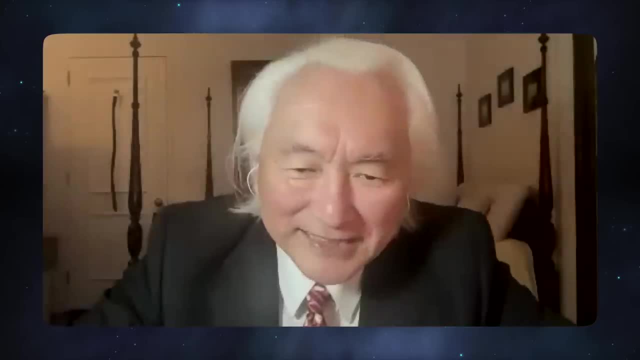 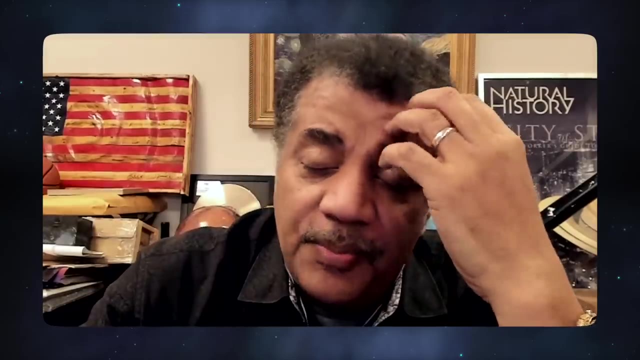 of the fact that the opposite sides is instantly transmitted, faster than the speed of light. but try, try, sending Morse code that way, wait, wait. so what you're saying is: but but then maybe you misspoke because you said you put on the green sock, right, right, and then send out the red sock. 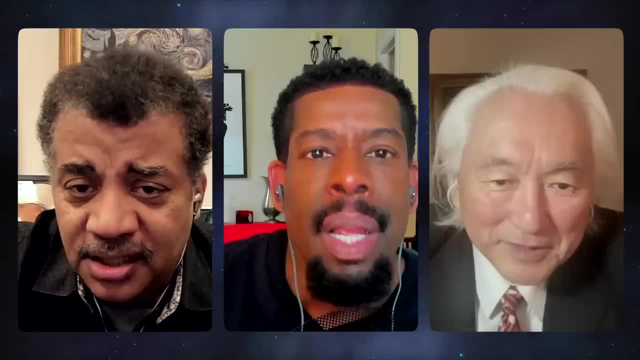 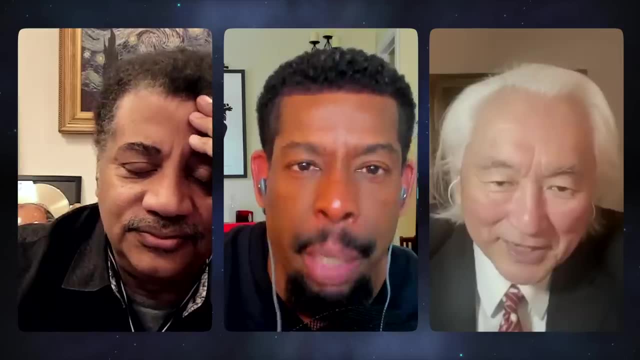 but you don't know that you put on a green sock. You just know you put on a sock, Right, Yeah, okay, Well then, reveal that. It's the reveal that we're really talking about. Right, We're talking about the reveal. 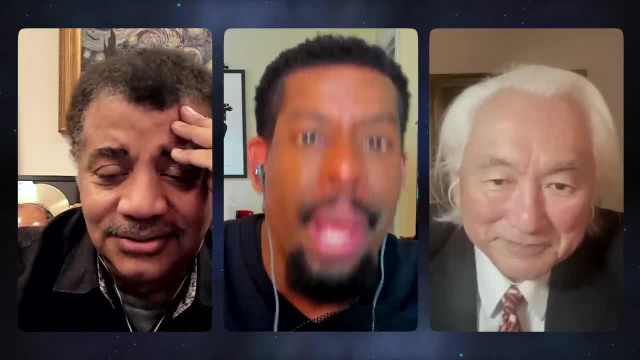 The position of the sock existed before the reveal, But we don't know what it is. But once we know what it is, then we know the information, Then everybody knows everything, Then we know the information By George. he's got it. 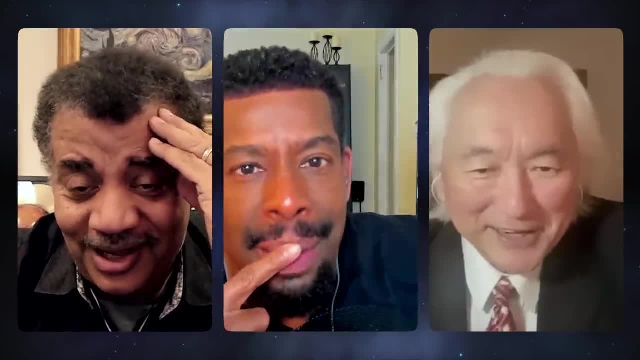 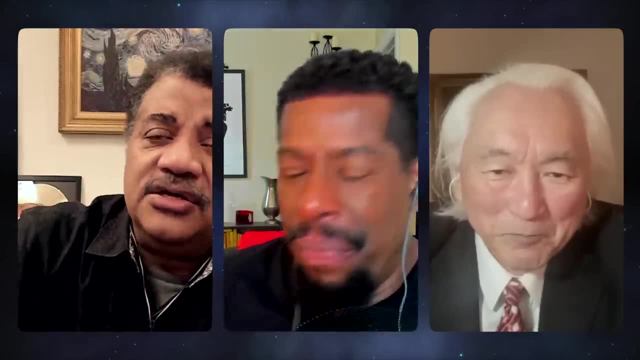 Got you There, you go There. it is A physicist in the making right here. We're going to give him an honorary StarTalk degree at the end of this. Okay, All right. Wow, All right. so it's not useful. 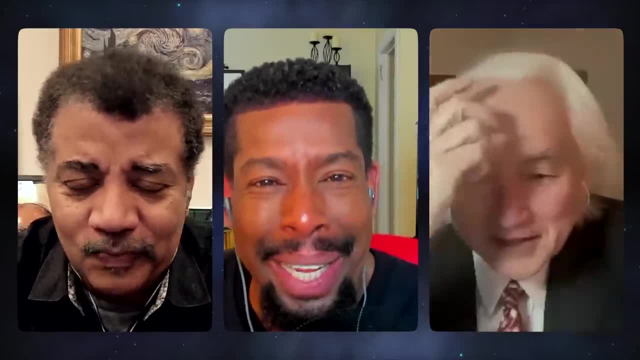 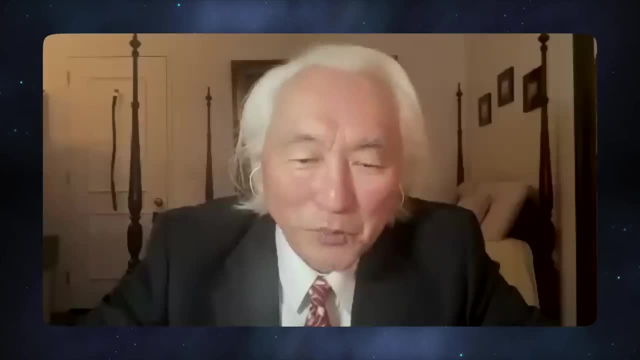 All right, It's not useful. God, that's so disappointing. I know Now the way to go faster than the speed of light, consistent with Einstein's theory, is wormholes. Wormholes will take you faster than the speed of light. 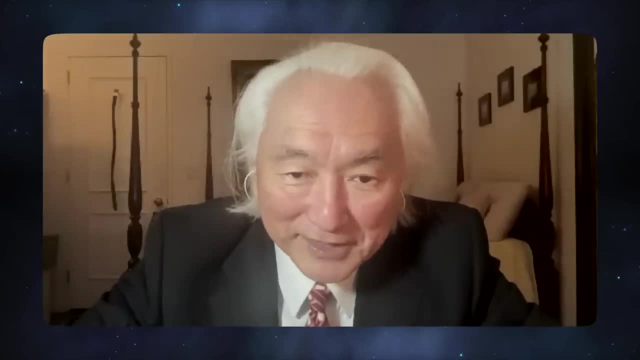 And it is consistent with the known laws of relativity. Stephen Hawking even wrote papers on it. Now, to create a usable wormhole is quite difficult. You'd have to have negative matter and positive matter, But in principle if you could have negative matter, 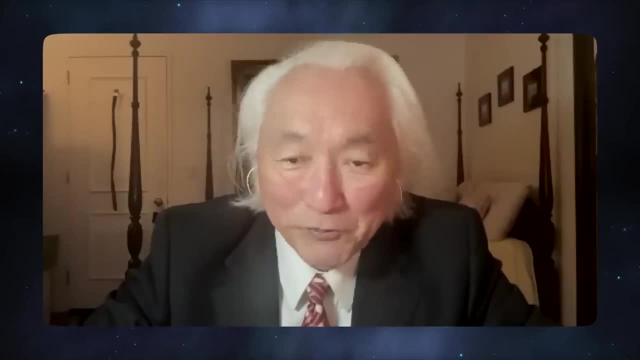 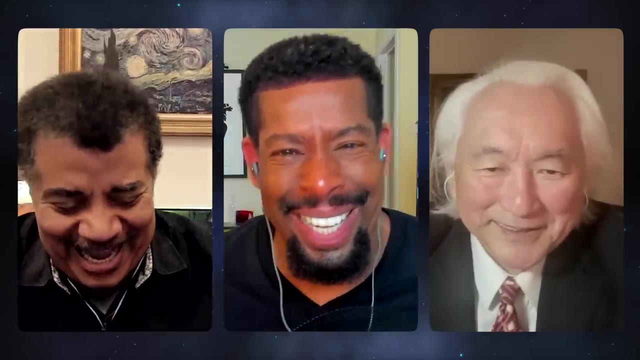 and positive matter. you could go faster than the speed of light in a wormhole, And Stephen Hawking even wrote papers. Wait, Chuck, he just said when pigs fly. Just to translate: All we need is negative matter. Yeah, 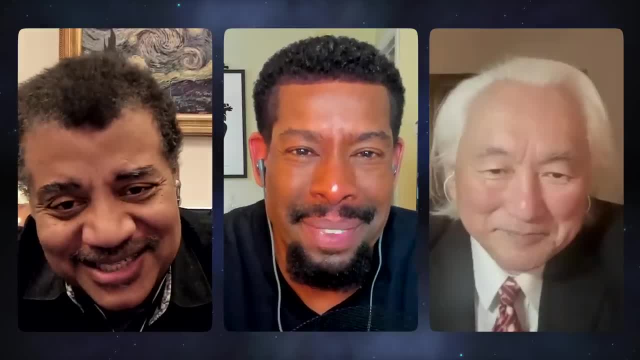 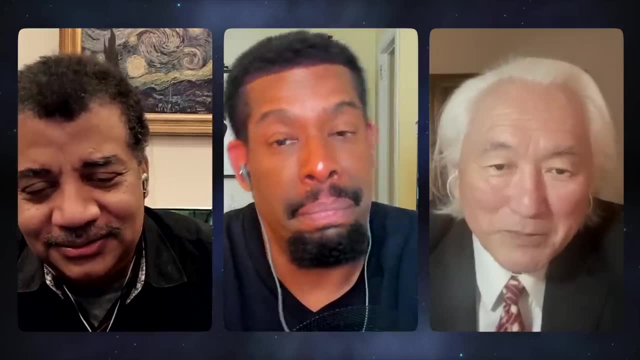 Yeah, okay, All right. So, Micho, when pigs fly, continue, Yes, No, negative matter is very rare. Instead of falling down, negative matter falls up. Now, when was the last time you saw a rock fall up? 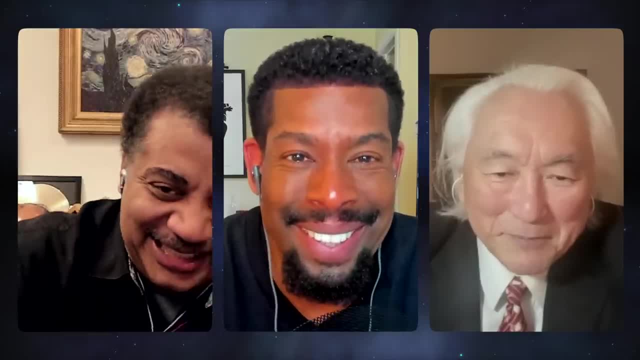 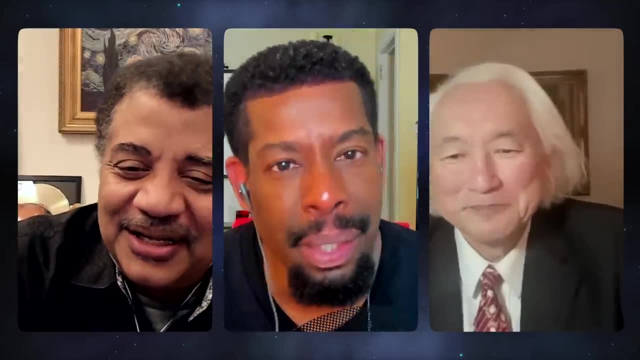 When was the last time you saw a pig fly? Okay, Okay, But if you could, if you could create negative matter, you could go faster than the speed of light through a wormhole. All right, Got you. Okay, And just to be clear, you're not actually. you're still not moving through space faster than light. You're kind of cheating in an authentic way by curving space And the wormhole then cuts through a passageway And so you're effectively going faster than light, But you're not actually moving through the fabric of space. 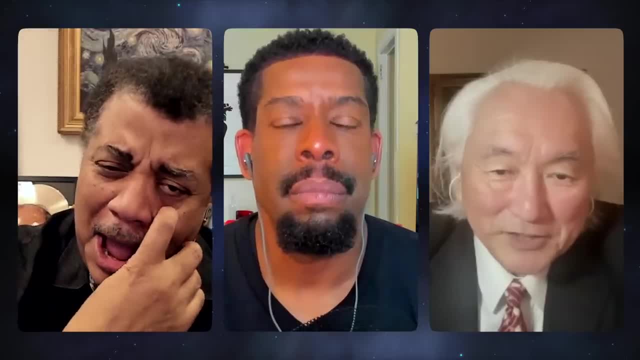 You're actually moving through space time faster than light. Is that that's a fair way to say it, right? Yeah, that's right. You simply hop across. Yeah, Yeah, it's a hop. So you're a whole. there's a hole there. you just hop across. 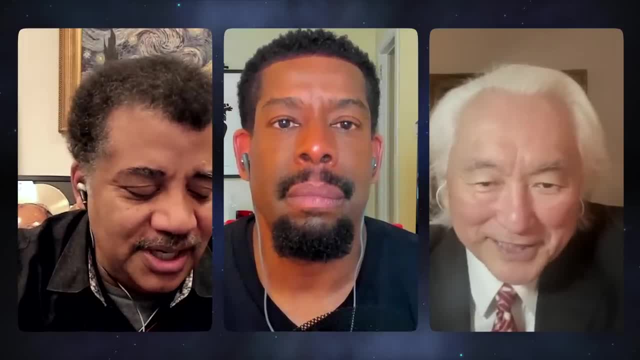 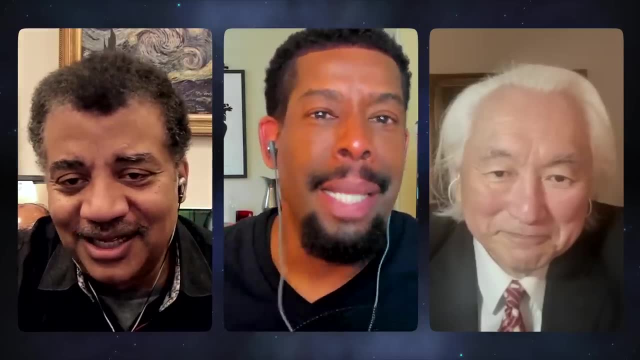 How fast did you go? Zero, Zero velocity, Right right, You just hopped across, Right Okay, There you go, Wow. And Rick and Morty knew all about this. Exactly, That's portal guns. That's all. that's all we need. 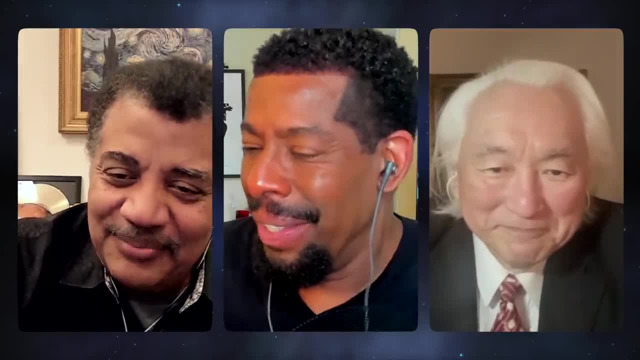 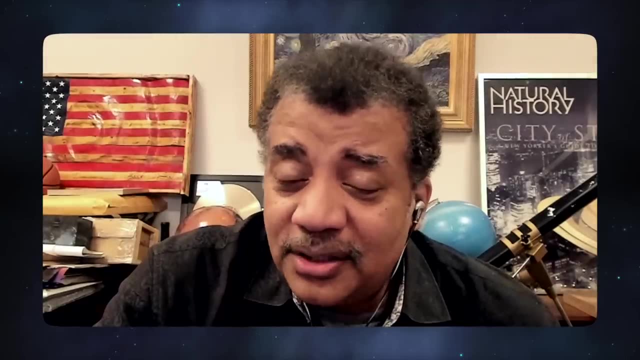 All we need are portal guns. All right, Maybe Violetta will invent one of those, a portal gun. Probably, I think she'll tell us about it first, and then we can, like, take over the world from there. I love every second of that. 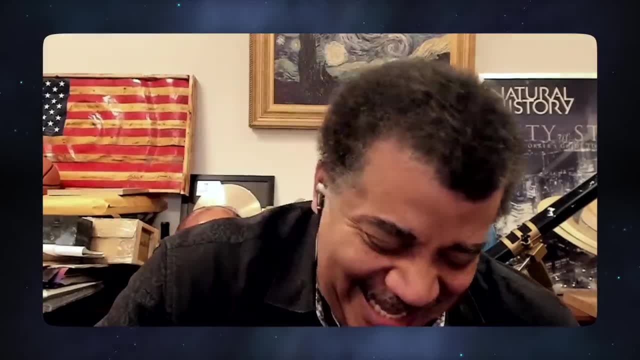 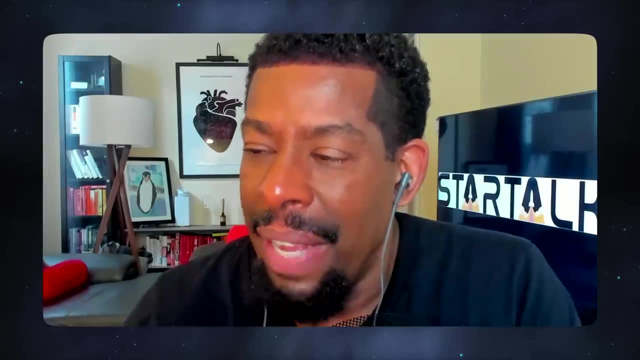 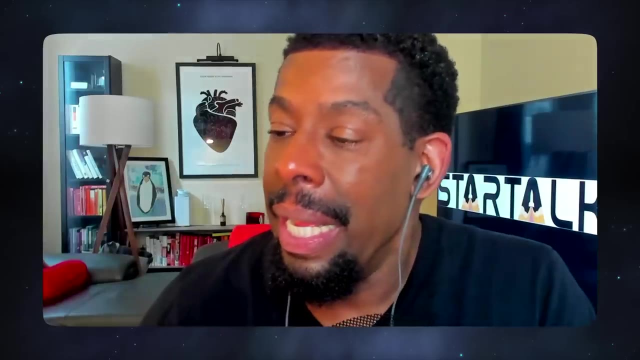 Yeah, Violetta will be the world's overlord. All right, This is Zygmunt Wasik, I believe. I believe. that's it Zygmunt Wasik. He says in singularity: I have been told that mass could have infinite density. 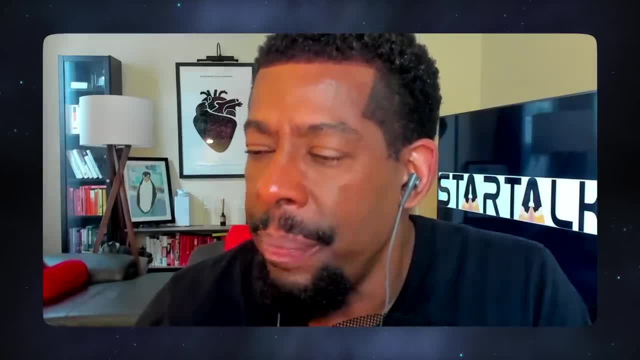 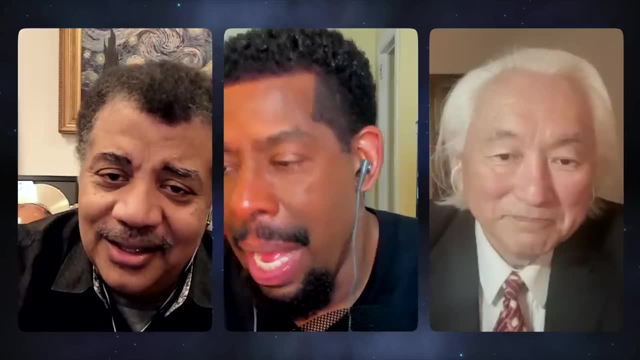 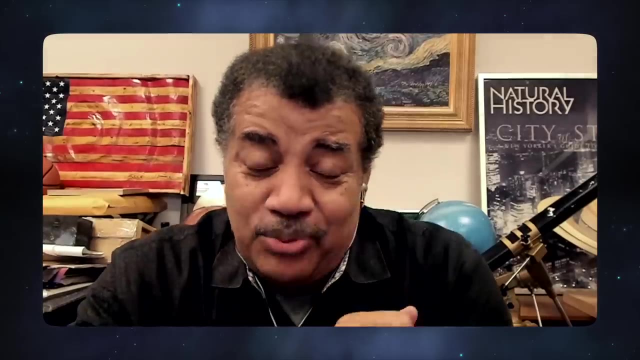 Can the algorithm of a quantum computer resolve mathematically infinity? I like that. Wow, I like that. So, Michio, it seems to me that if you take general relativity to its limits, at some point you're dividing by zero or its equivalent right. 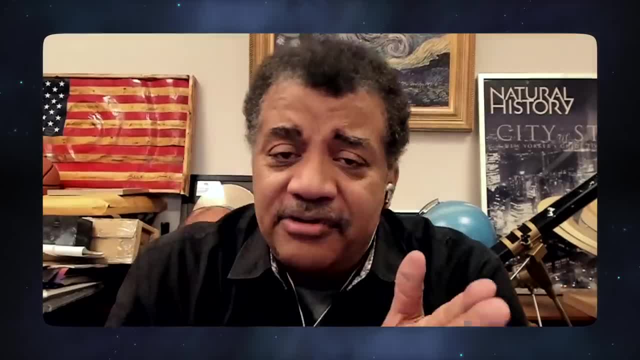 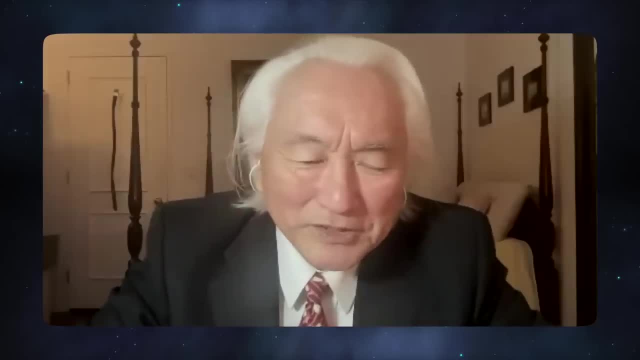 So is there some point where you say, uh-oh, general relativity stops. now we need some different kind of math or more powerful physics, That's right? The distance at which Einstein's theory of gravity breaks down, and the quantum theory? takes over is the Planck length. Planck length is 10 to the minus 33 centimeters. Okay, All right, That's a very small number, Damn Yep, Yep. And how would you then manipulate something like this, If you have empty space and you could heat it up, heat up empty space to the Planck temperature. 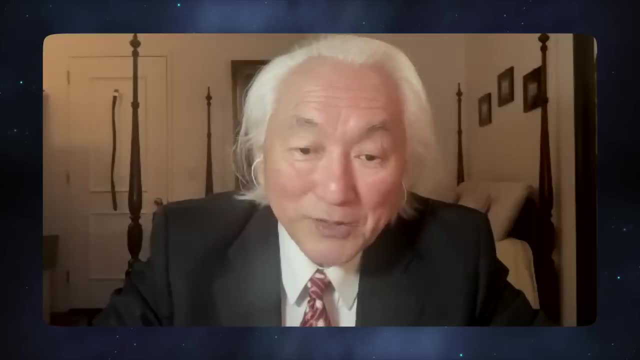 then bubbles will begin to form. just like you boil water, You heat water. water boils, You heat space. space will boil at the Planck length or the Planck temperature And at that point each bubble is a wormhole and each bubble in principle can become. 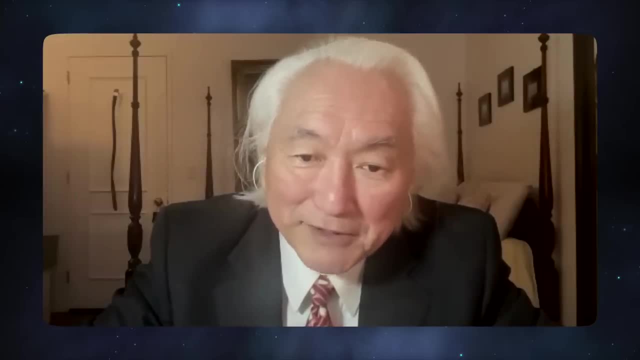 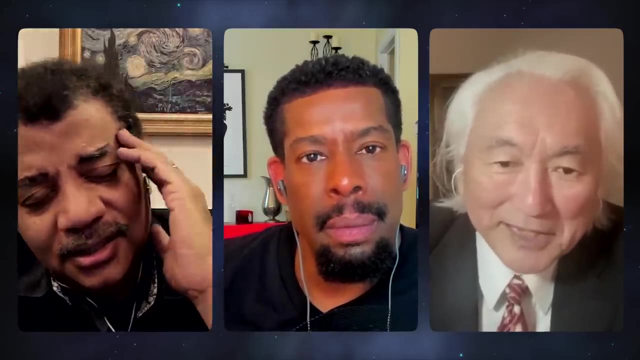 a universe. Oh, In fact, that's probably where our universe came from. Our universe probably came from a bubble in nothing that expanded, giving you the Big Bang of today. Okay, Michio, you keep talking like that. Chuck is going to run out and smoke a joint. 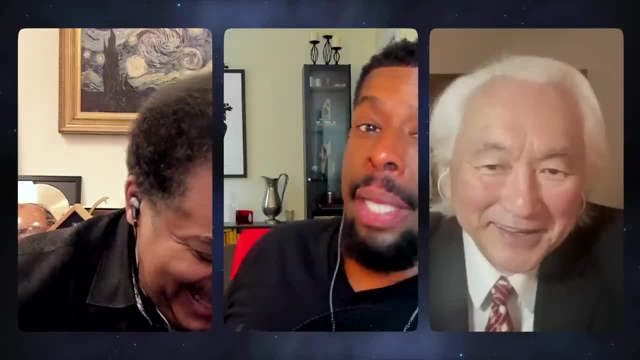 Okay, I didn't smoke one. Are you kidding me? I don't know why y'all were talking. I couldn't wait to smoke. I was like: forget it. You want to boil the universe, Michio? That's amazing. This sounds like out of control. We've done the calculation. People who are doing what is called inflation theory have calculated what it would be like to be a god to create your own universe. Of course you want to do it safely. You don't want to blow yourself up in the process. 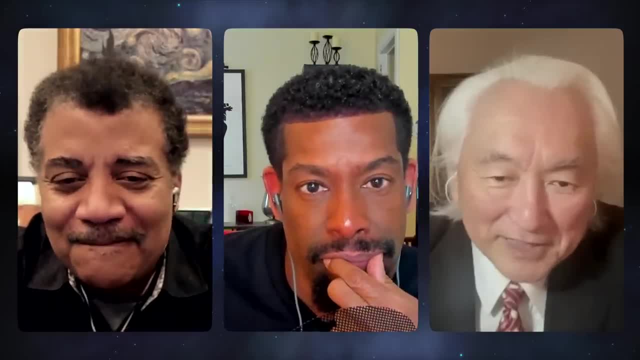 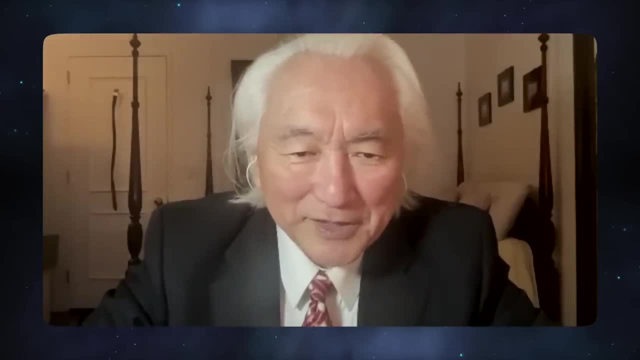 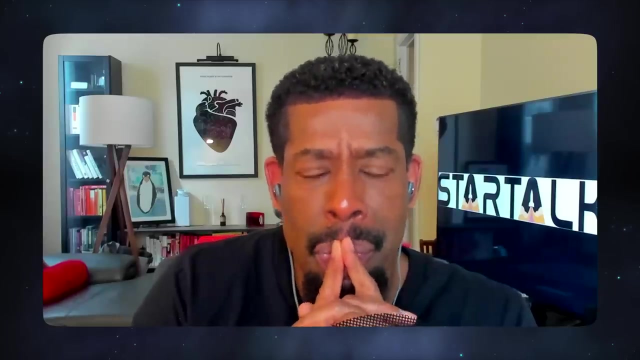 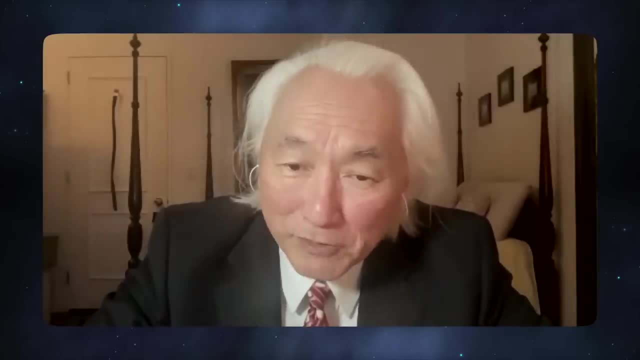 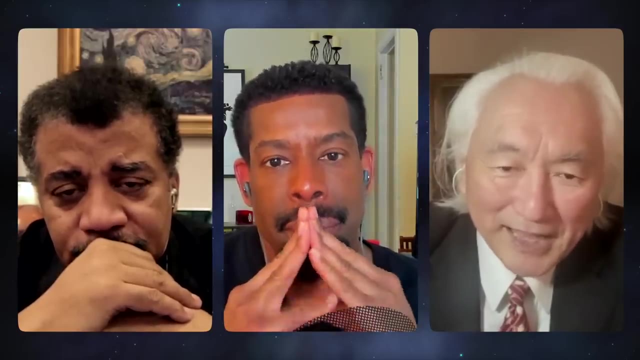 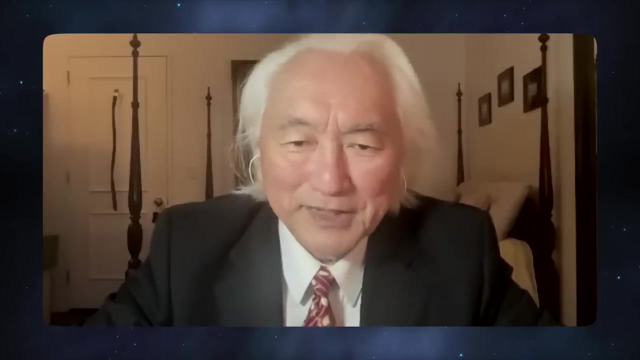 all the time, each bubble being a wormhole, But one of those wormholes just kept on going and here we are. That's how the universe started. we think, Wow, Wow, of the Planck energy, or the Planck length, as energy is 10, to the 19 billion electron volts. 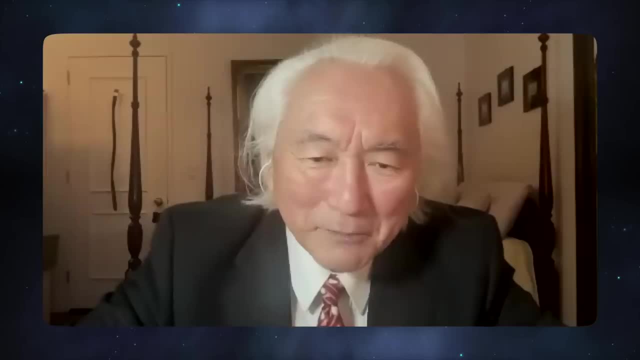 as a distance is 10 to the minus 33 centimeters. But that's my world. I live in the Planck length and the Planck energy String theory lives there. Michio, that ain't right to call us a fluctuation. 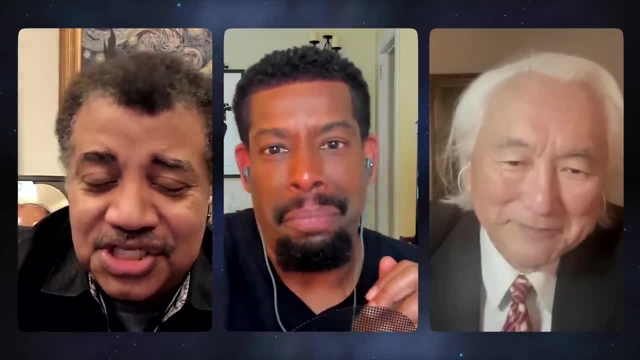 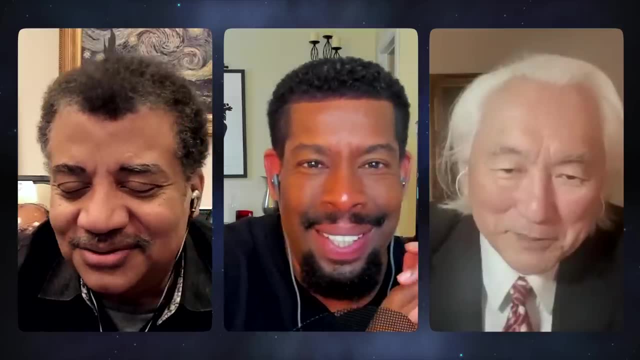 That's right. We are a fluctuation. Yeah, It's a cherished universe is a fluctuation. All right, There you go, You guys are. you're a blip, That's what you are: A fluctuating blip, That's. 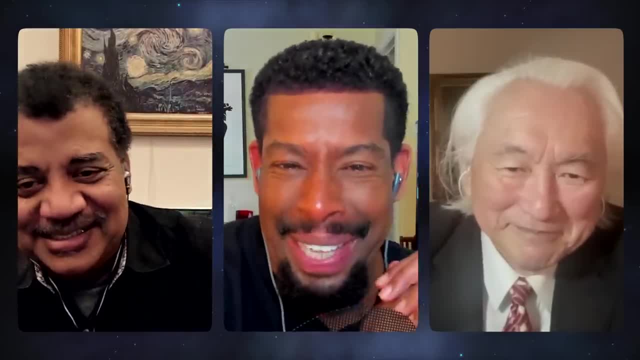 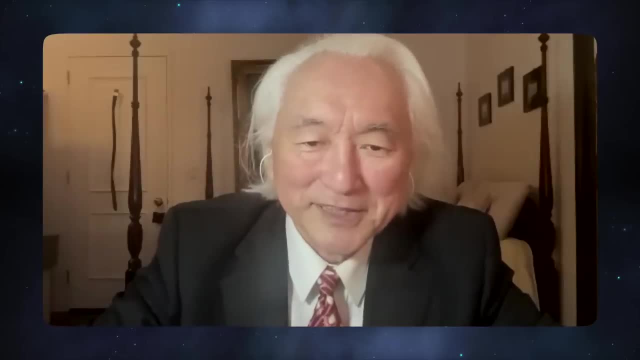 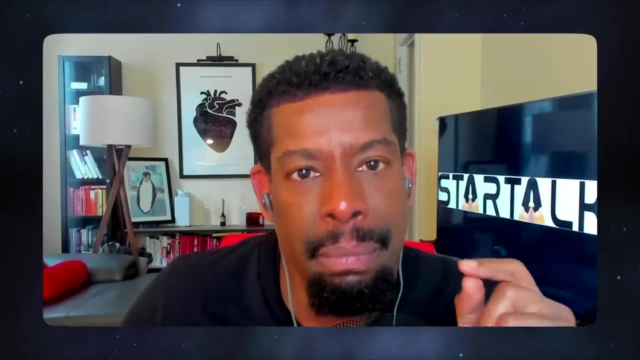 what you are, Don't you feel good about yourself? No, that's what we call them. When you write papers, you write papers on quantum fluctuations of nothing. Even nothing's unstable Nothing would violate the Heisenberg uncertainty principle. Pure nothing is not possible. 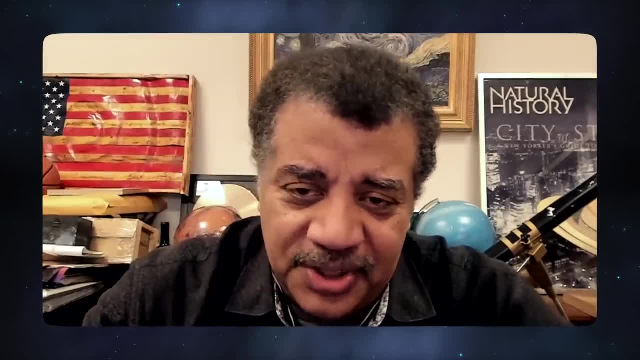 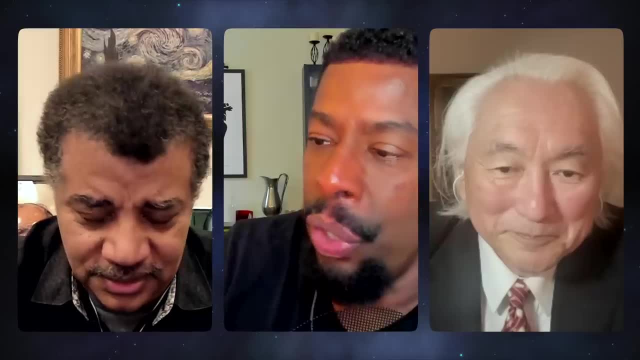 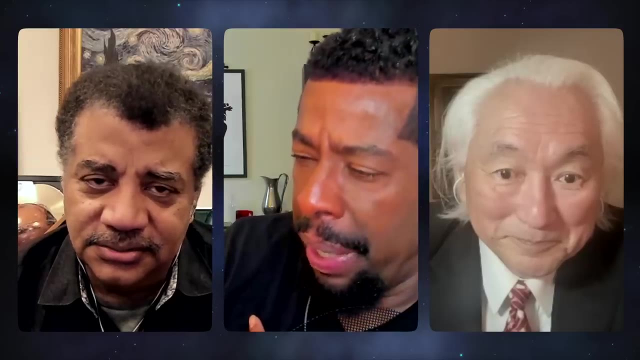 Right, All right, Let's get back Time for a couple more questions on quantum computing. This is Alan, And Alan says hello. Dr Kaku, I used to watch your YouTube channel and I've been watching since 2012.. I'm a huge fan. I live in Lithuania And could you please explain on string theory. 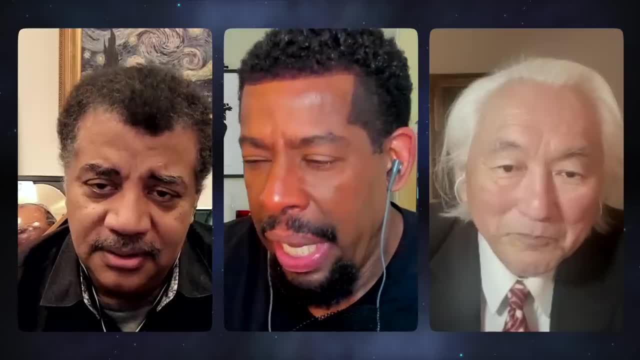 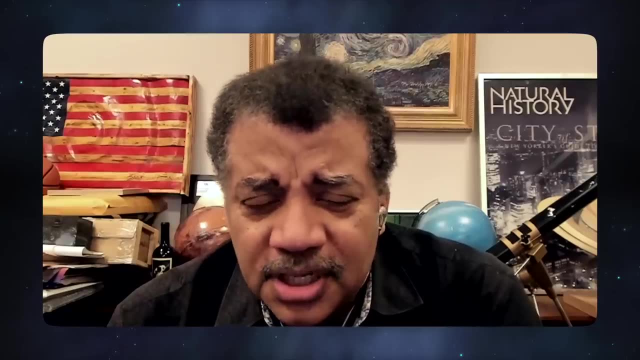 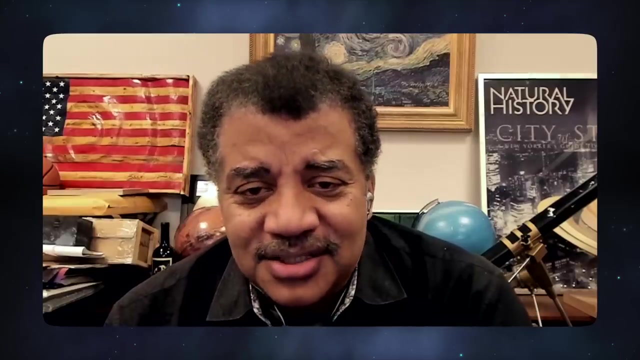 what force makes a quantum string vibrate its string? And are there strings in the circuit boards of quantum computers? Or you're just going to say there's strings everywhere. you know, just strings all the way down, as they say. So how does everything you know about strings inform? 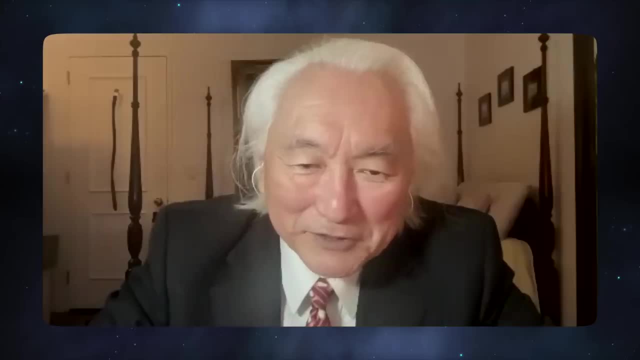 the people trying to perfect a quantum computer. Okay, First of all, strings have to fluctuate because of the Heisenberg uncertainty principle. Pure, nothing pure, motionless pure, anything like that- violates the uncertainty principle. Therefore, strings have to vibrate. 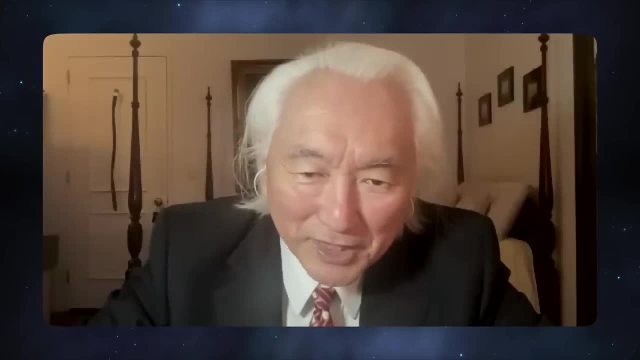 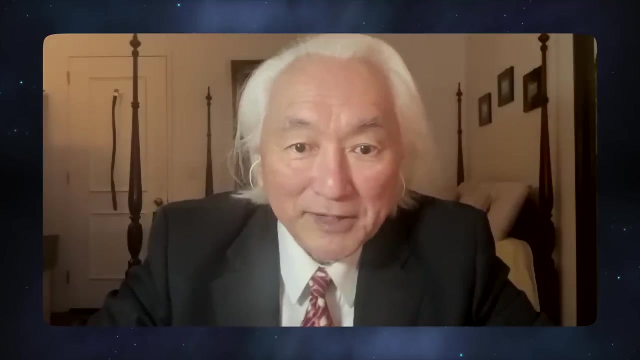 The lowest string, the lowest vibration of the string gives us our universe. Our universe is the lowest vibrating octave of the string. There are higher octaves of the string And these higher octaves, we think, correspond to dark matter. So that's why we have dark matter, because 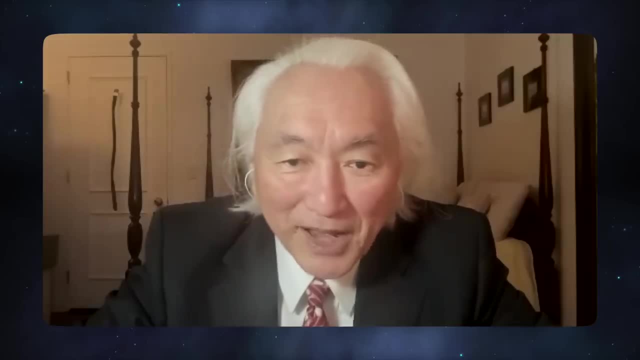 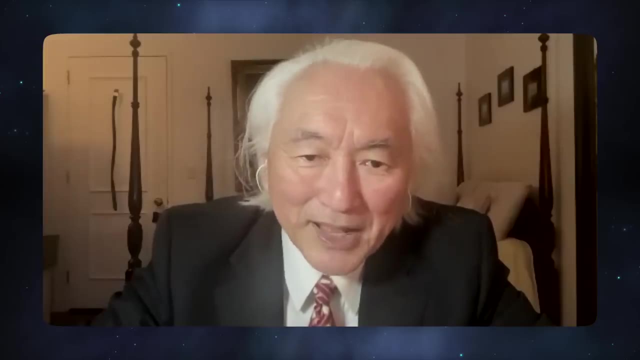 it's nothing but the next higher excitation of a vibrating string. But again, strings have to vibrate because of the Heisenberg uncertainty principle. This is a quantum theory, And when the strings vibrate they create subatomic particles, mainly us. We are the lowest vibration. 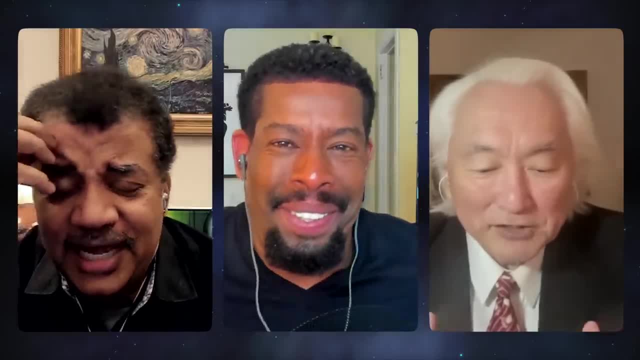 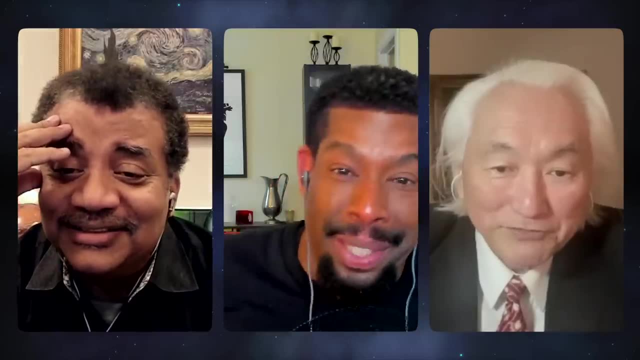 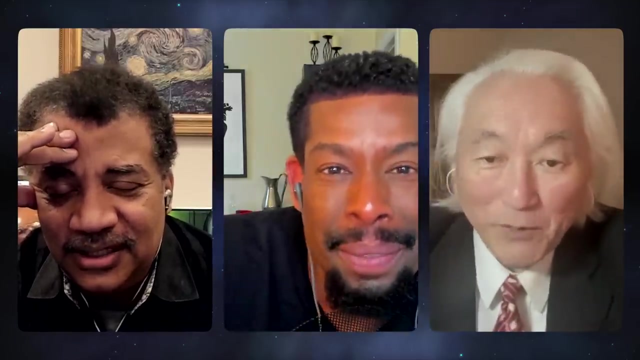 of the string Sometimes say: well, can the string predict our universe? Yes, our universe is the lowest vibration, We're fluctuating blips and we're the lowest of the low. That's right. And the next set of vibrations would be dark matter, And one day we're going to find 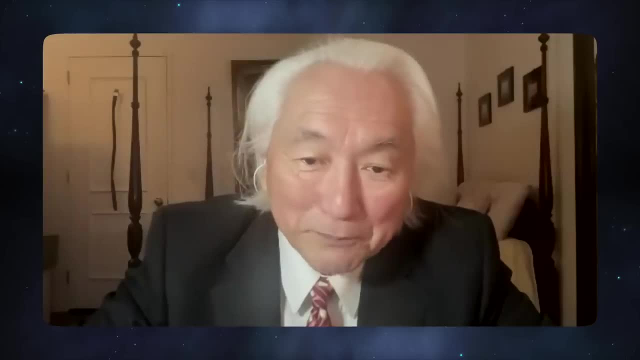 dark matter and that could clinch it. People want experimental proof of the correctness of string theory. That could prove it If we find dark matter in a laboratory, analyze its properties and show that it's predicted. it gives us an answer. 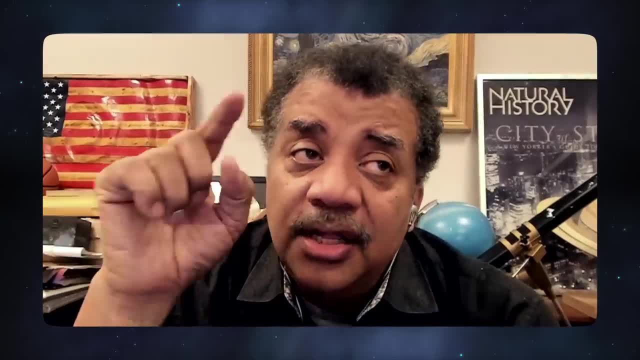 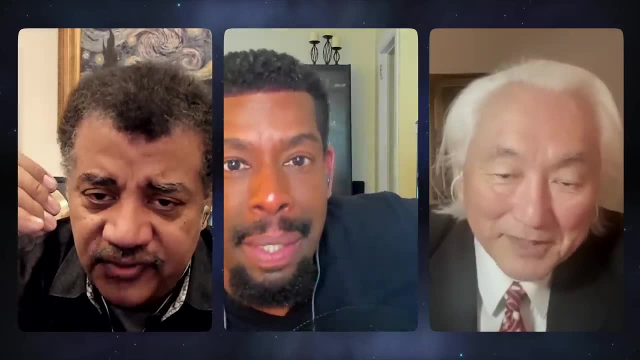 But that should not be part of the next vibration, the next octave of the string. OK, So back to the question. The string, in its natural state, vibrates, because it can't not vibrate Right, That's it, Because of the quantum mechanics. 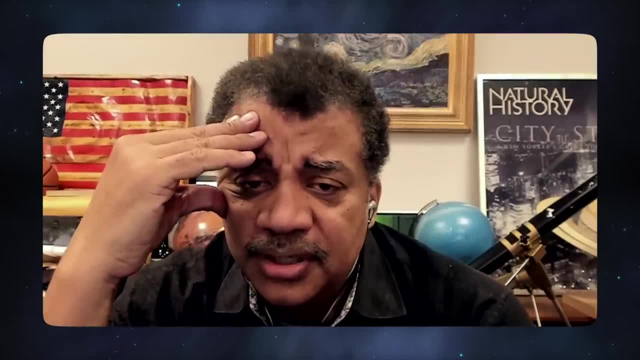 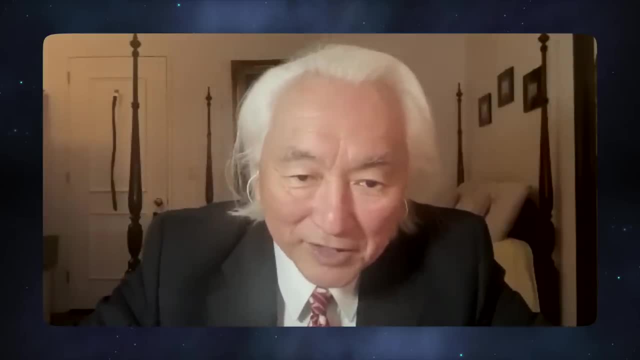 The quantum mechanics Got it. So then now is this exploitable in a computer circuit, In quantum computing? Well yeah, a computer circuit would have a low excitation of the string, I mean a low excitation of the electron. but the electron itself is an excitation function, Because the charge is only meant to be decisions grown byzn scallion, but if we have the dominant starting phase, then because obviously there may be logic to love the cost and the Speech-Wea Set. we just need a���hesia in this slice. Yes, 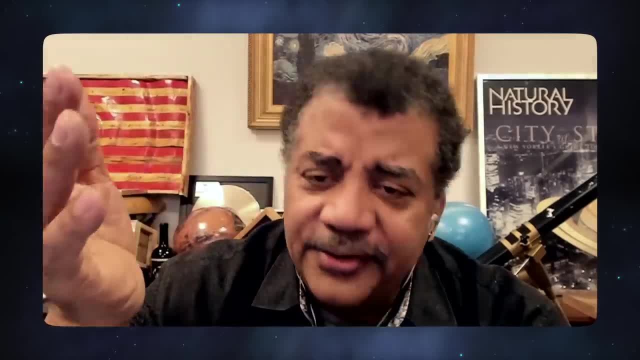 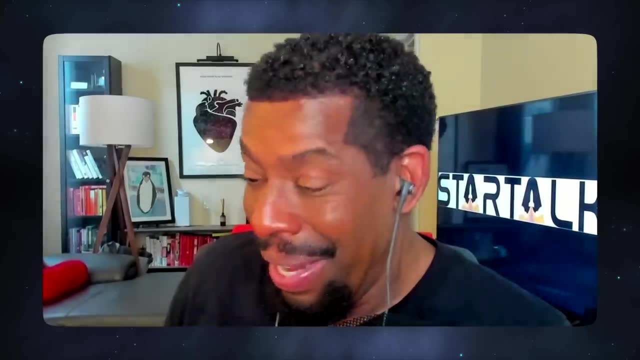 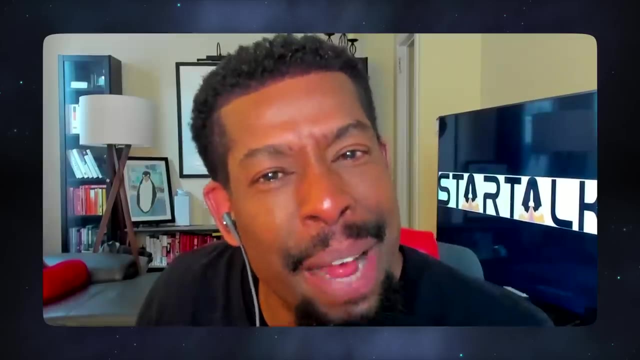 itself is an excitation of the strength. of the strength got it, okay, all right, there you go. so, chuck, do we have one last quick question? all right, how about this one? this, here we go, charles macko or mako. he says, hey, what comes after quantum computing? 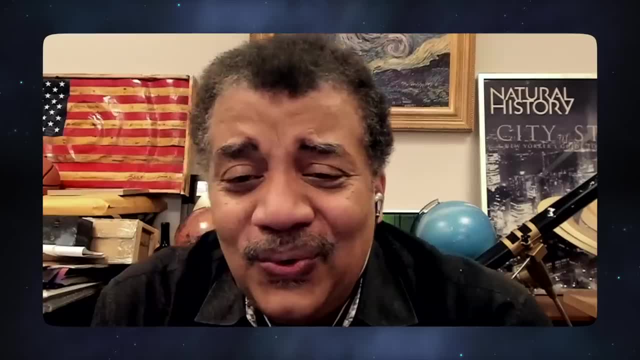 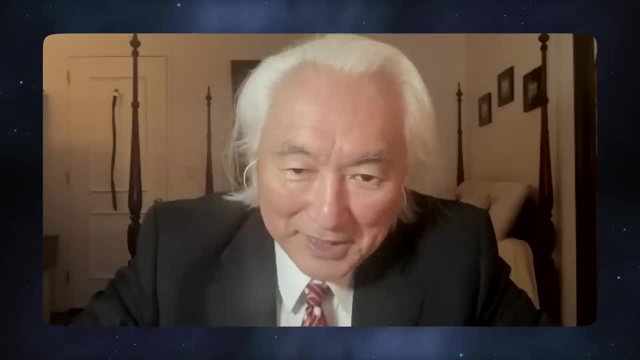 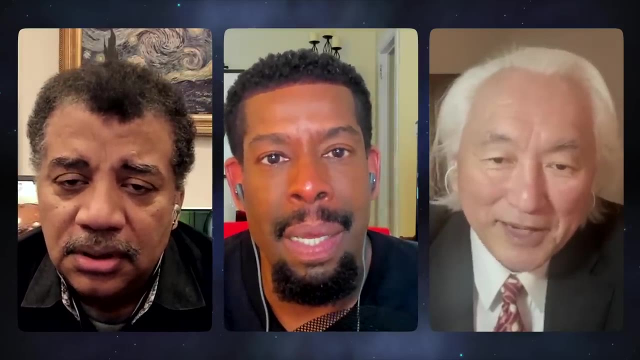 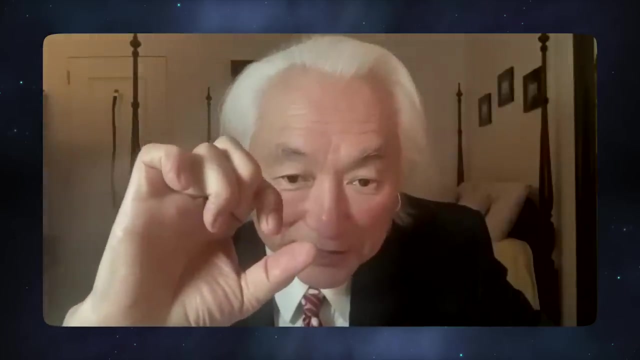 i think that the step beyond quantum computing is nuclear computing, because quantum computing computes on electron shells. we're talking about the electron shells that give us the bore atom, you know, electrons going around the nucleus, but the nucleus itself is nuclear and it also is quantum mechanical and that, in principle, is stable. 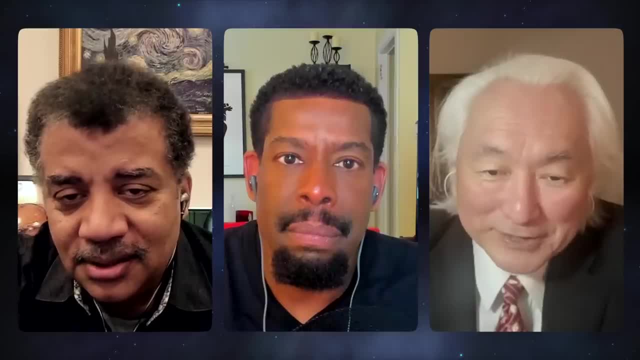 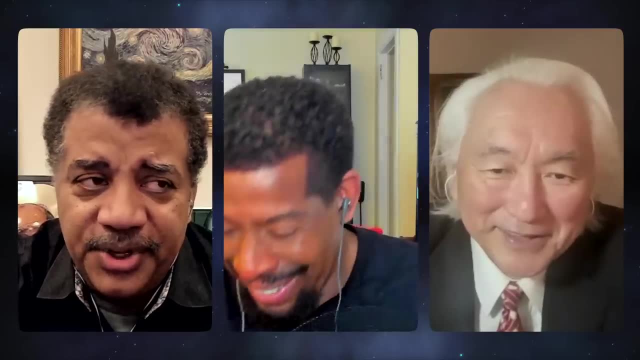 and that, in principle, is stable. and that, in principle, is stable, So you can make things out of it. However, of course, if you don't watch out, you could hit critical mass, in which case that would ruin your day. It would destroy the universe. 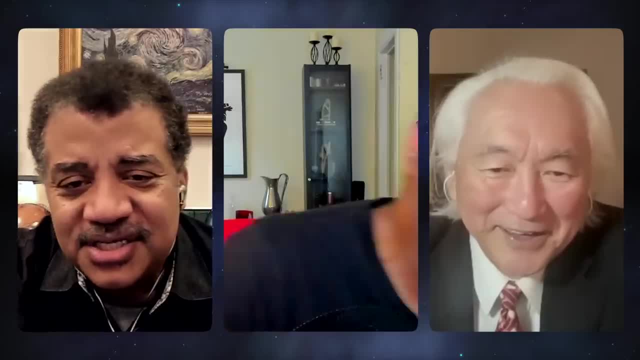 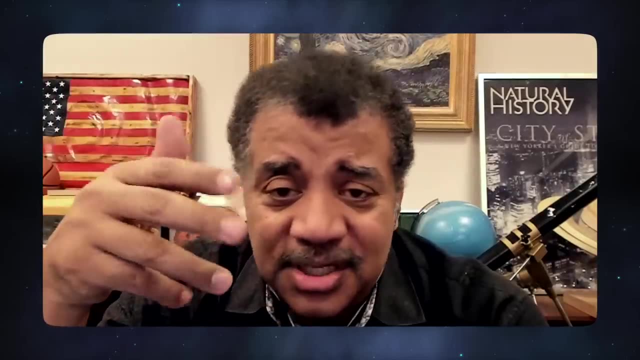 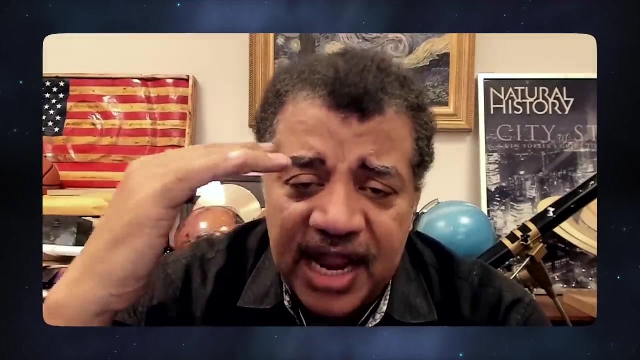 Yes, Okay, so it's interesting. What you're saying, Michio, is that all these rules that we're talking about are electron-based and electron orbitals and all of this electron spins, But you can go deep into the nucleus and there's a whole other realm that is, in principle, in reach.